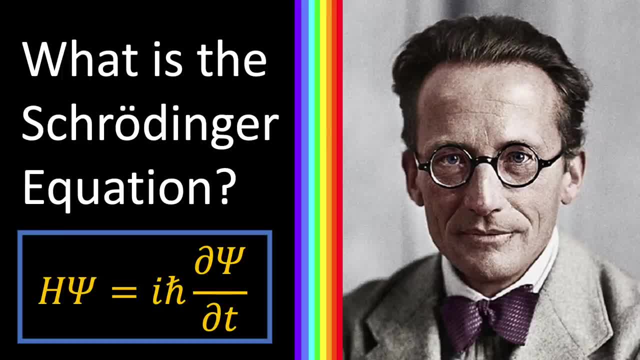 In this video, I would like to tell you about one of the most famous and important equations in physics: the Schrodinger equation. It's an equation that lies at the heart of quantum mechanics and it forms the basis of much of our modern understanding of the universe. But what exactly is the Schrodinger? 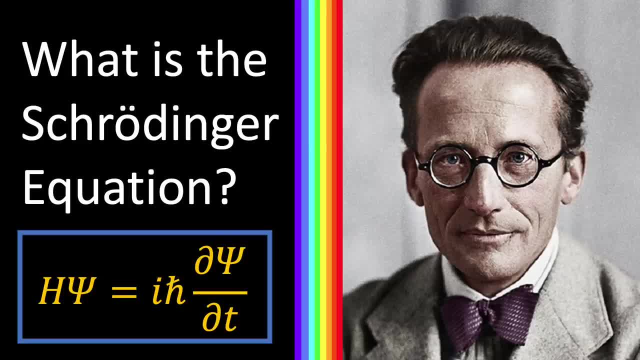 equation and how can we use it to perform quantum mechanical calculations. In this video, I will provide an introductory overview of Schrodinger's equation, with my aim being that by the end you should hopefully be ready to pick up an undergraduate textbook on quantum mechanics and actually enjoy the experience. So if you're up for the challenge, stay tuned. Our story begins. 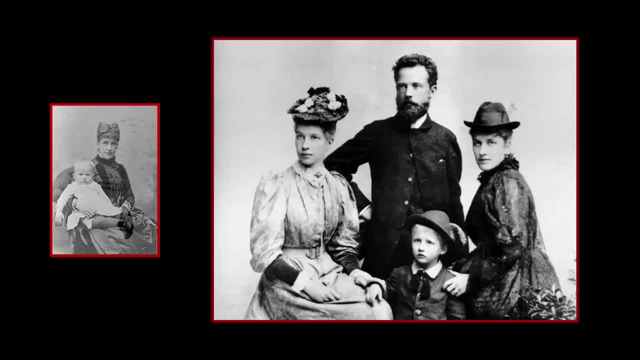 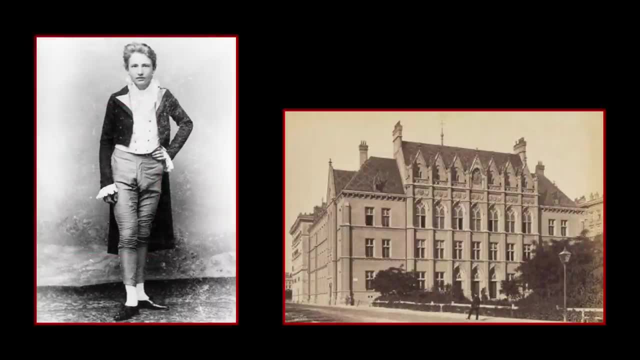 in Vienna when, on the 12th of August 1887, Erwin Rudolf Joseph Alexander Schrodinger was born. As was customary at the time, Schrodinger was educated at home for the first 11 years of his life before attending the local gymnasium school, almost from the very first day until he 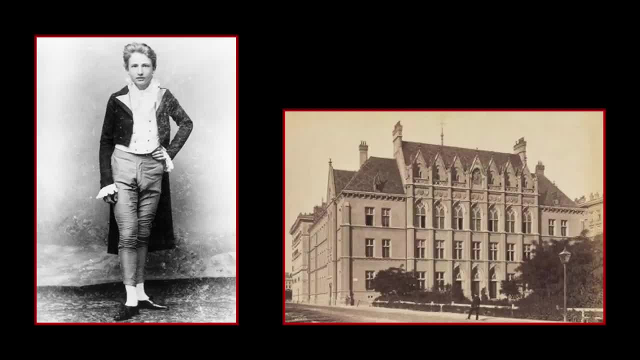 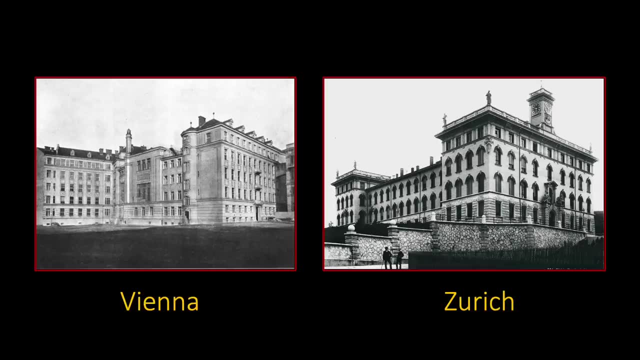 left eight years later. Schrodinger excelled in mathematics and physics. When Schrodinger eventually arrived at the University of Vienna, much was expected of him and he did not disappoint, consistently coming top of his class. His efforts were rewarded in 1910. 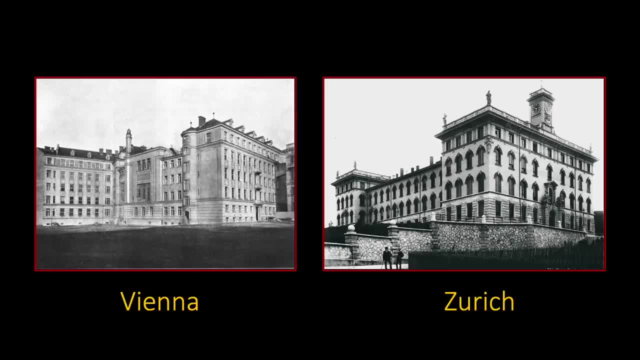 when he received his doctorate, and after a short stint of military service, Schrodinger joined his old university as an assistant of experimental physics. In 1914 the first world war intervened, and soon after the war ended Schrodinger was sent to Vienna to study physics. He was then 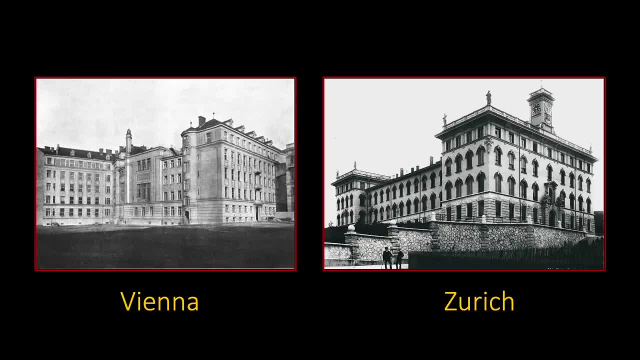 sent to the University of Vienna to study physics, Schrodinger took up a position at the University of Jena. The next 10 years saw Schrodinger move between numerous institutions in Europe before he finally settled in Zurich, Switzerland, at the age of 34.. As the next few years passed, 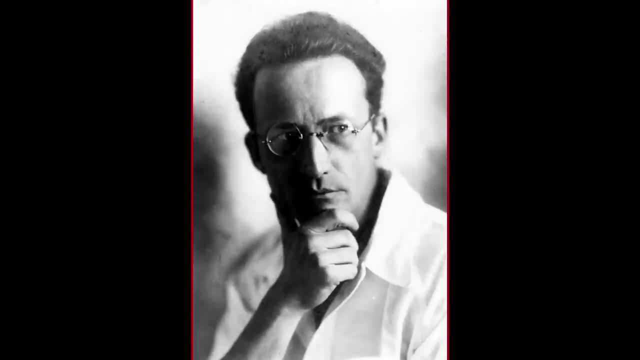 Schrodinger began to wonder if he would ever make a major contribution that would establish him among the first rank of contemporary physicists. At the beginning of 1925, he was 37 years old, long past his 30th birthday, which was believed by many to be the watershed in the creative life of a theoretical physicist. 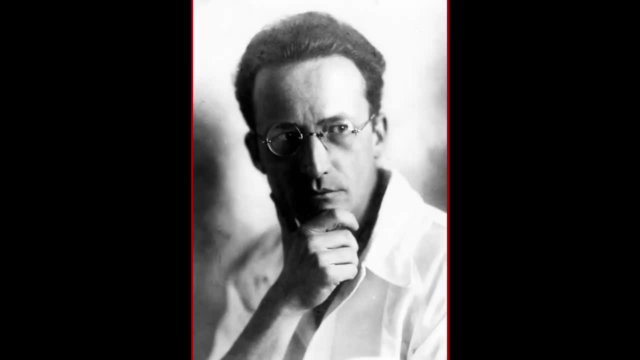 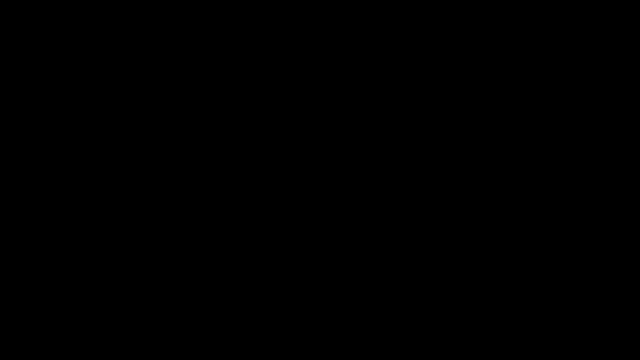 However, by the end of the same year, he would make a breakthrough that would ensure his place in the pantheon of physics. So what was it that suddenly changed the tide for Schrodinger? In October 1925, Schrodinger read a paper that Einstein had written earlier in the year, relating 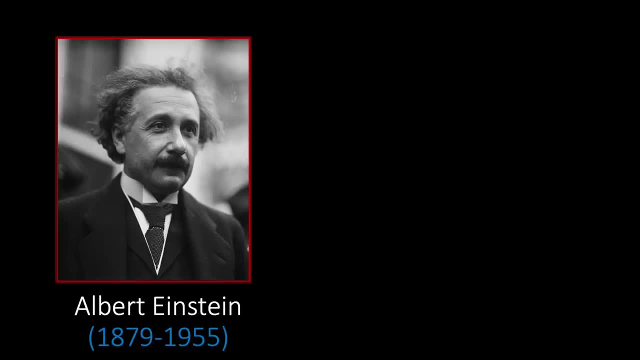 to the latest developments in atomic physics. A footnote in Einstein's paper mentioned the thesis of a young French physicist named Paul Schrodinger. He wrote that the idea of a new world of physics, which was believed by many to be the watershed in the creative life of a theoretical physicist, 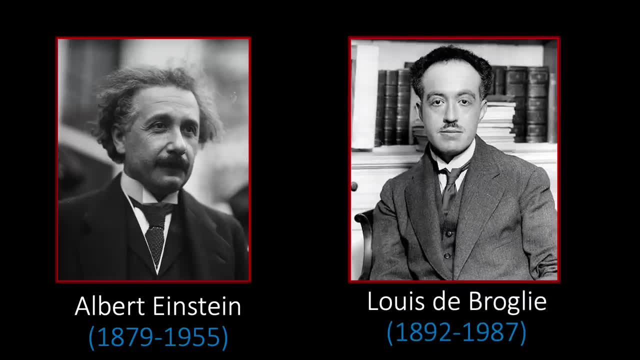 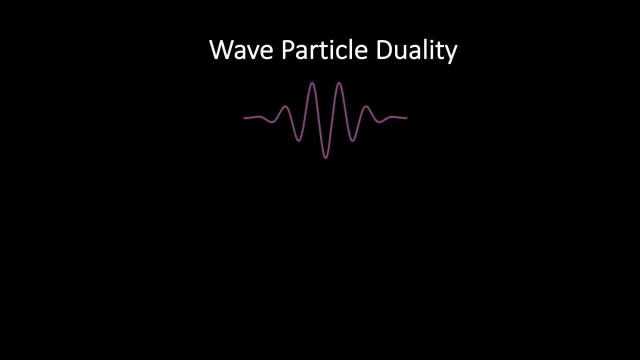 had been revealed by a scientist named Louis de Broglie, who had recently published his thesis on the theory of wave-particle duality. a few years earlier, This rather innocent footnote caught the attention of Schrodinger, and he set about acquiring a copy of de Broglie's thesis. What was particularly exciting for Schrodinger? 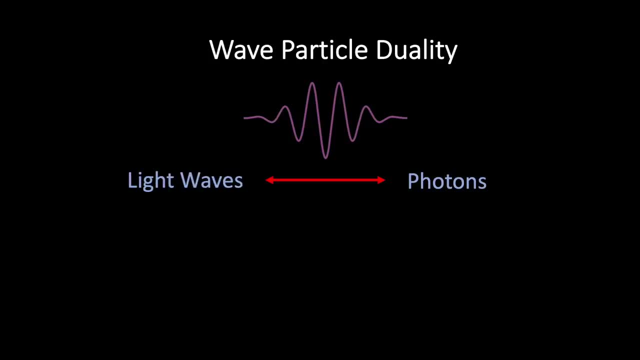 was that de Broglie had dared to ask the question that if light waves can behave like particles, as has been shown by Einstein's explanation of the photoelectric effect, is it then possible that particles such as electrons can behave like waves? De Broglie's answer to this question. 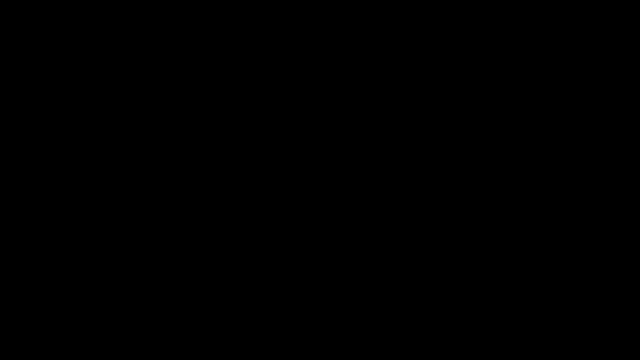 was an unequivocal yes. In summary, De Broglie proposed that for a matter particle with mass m moving at velocity v, you can associate a plane wave of wavelength lambda equals h over p or h over mv, where p equals mv is the momentum of the particle and h is Planck's constant. Furthermore, 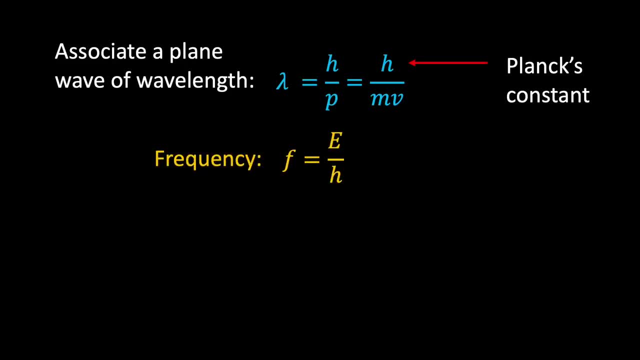 if the particle has energy, e, then you can assign a frequency given by f equals e over h, and these relations connect the particle concepts of energy and momentum, e and p, with the wave concepts of frequency and wavelength, f and lambda. Now, what De Broglie did was simply: 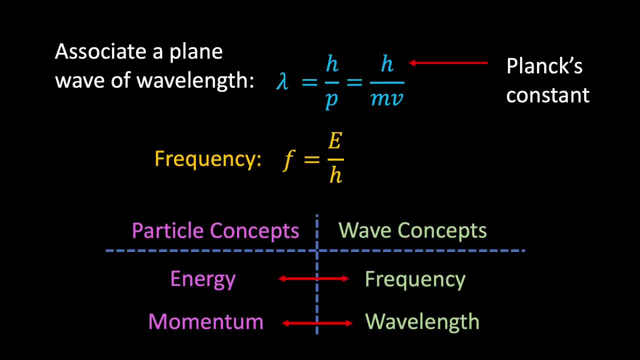 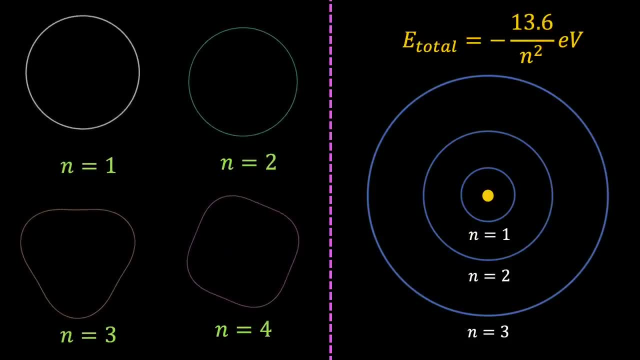 assume that these two relationships hold for all matter particles, including electrons. Although there was no experimental evidence at the time to support De Broglie's hypothesis, he was encouraged to work by the fact that he was able to provide an explanation for Bohr's model of the atom. 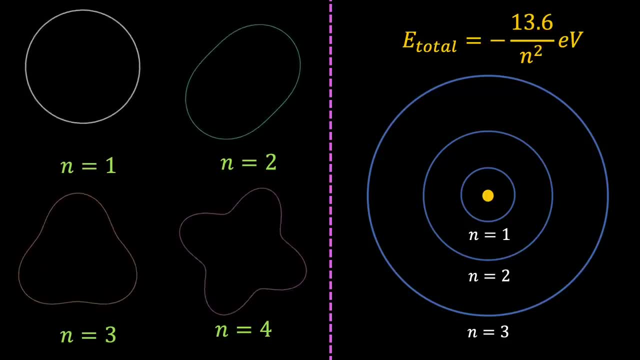 Although other physicists had taken a passing interest in De Broglie's work, the lack of experimental evidence dissuaded most from spending too much time thinking about the ideas. However, when Schrodinger read De Broglie's paper, he immediately wrote to Einstein to: 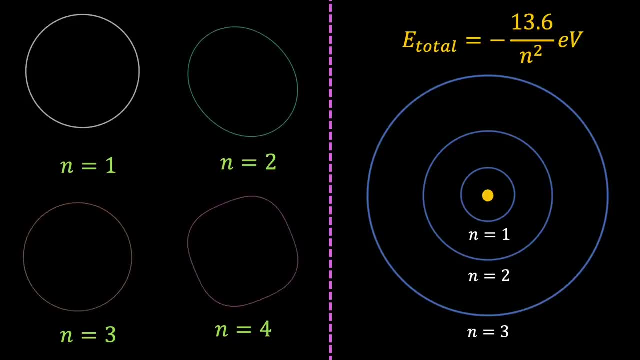 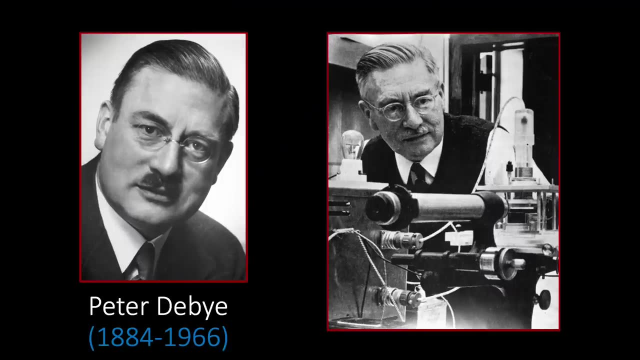 share his thoughts about the implications of wave-particle duality. A couple of weeks later, Schrodinger was asked by the physicist Peter Debye to present a talk on De Broglie's work at a physics colloquium in Zurich. Schrodinger gave a beautifully clear 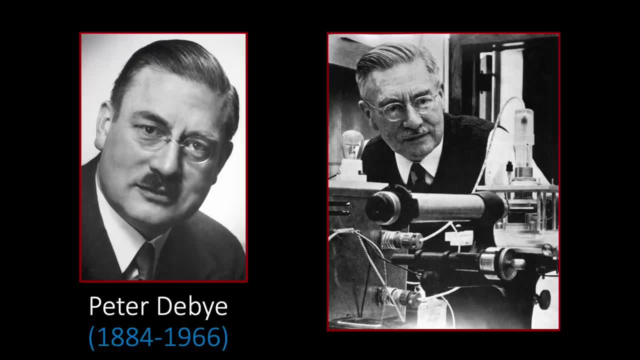 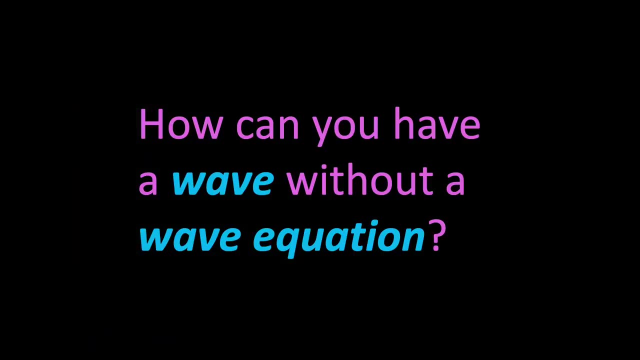 account of De Broglie's work. however, not everyone in the audience was convinced. In particular, Peter Debye did not like the fact that, according to De Broglie's theory, there appeared to be matter waves but no wave-equation to describe these waves. 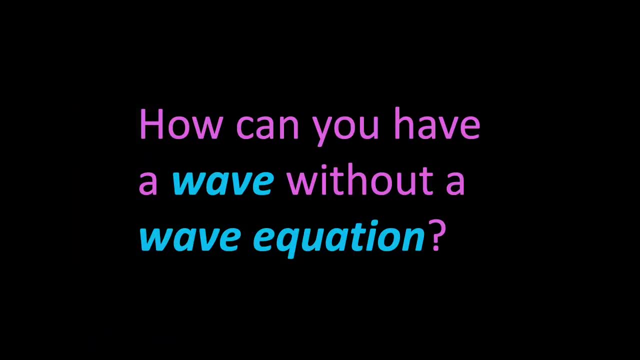 How can you have a wave without a wave-equation? According to the well-established Classical Laws of Wave Motion, any wave, whether it's a sound wave or a motion wavesren, can be replaced by a wavemotion, from the idea that those waves and waves, John Jay Gilchristill. 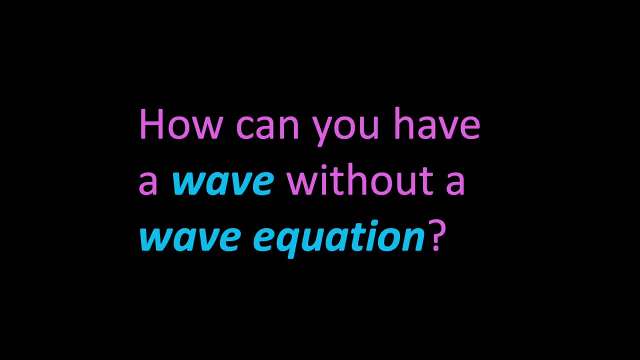 cooked for the planet and not for worse. This, was noted after Richardiander, was most consistent with the pirickểu in Szlugilar's paper, and in addition to that Karl siguitler wrote that no waveEST sums. whether it's a sound wave, electromagnetic wave or wave on a vibrating violin string has an equation. 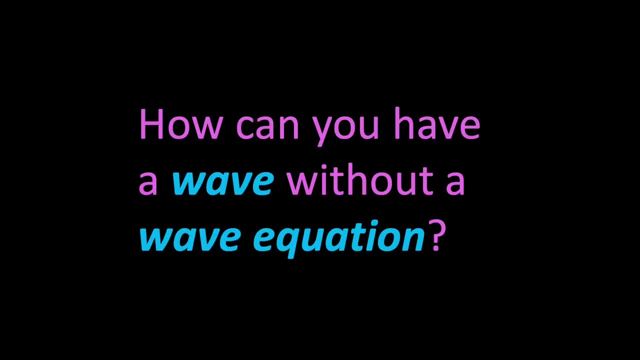 that describes its motion. however, in de broglie's theory there was no wave equation. de broglie had never attempted to derive one, and neither had einstein. schrodinger knew at once that de by was correct: you cannot have waves without a wave equation, and almost at once he decided to set. 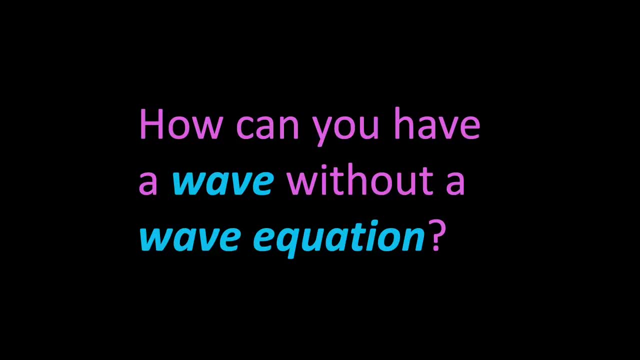 himself the task of finding the missing equation, and in the space of only a few months, schrodinger was able to take de broglie's tentative ideas surrounding wave particle duality and develop them into a fully blown theory of quantum mechanics. in the remainder of this video, i would 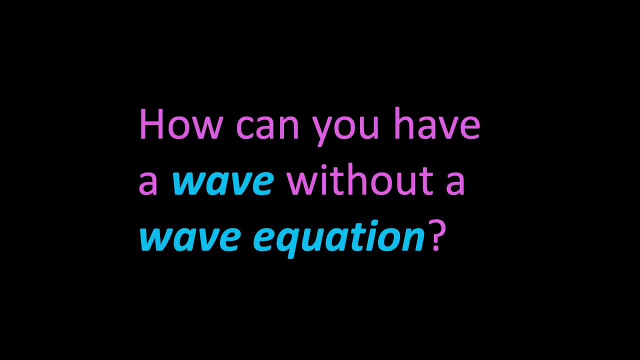 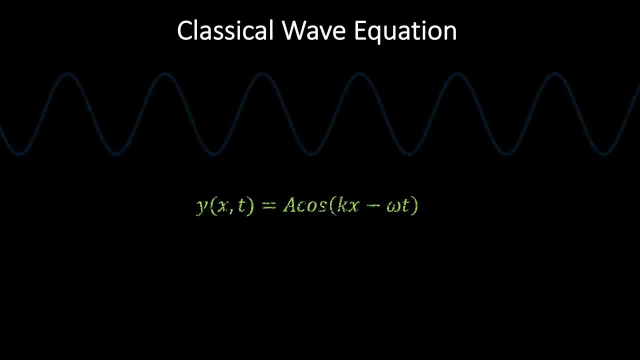 like to provide a simplified overview of schrodinger's theory. we will begin our investigation with a simple review of the properties of classical waves. a simple progressive wave which is moving towards the right can be described using a cosine function where y of xt is the displacement at. 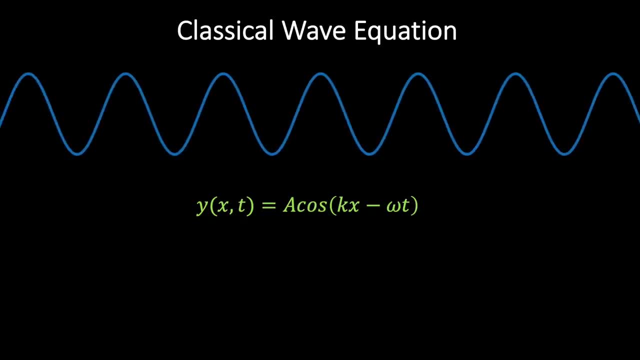 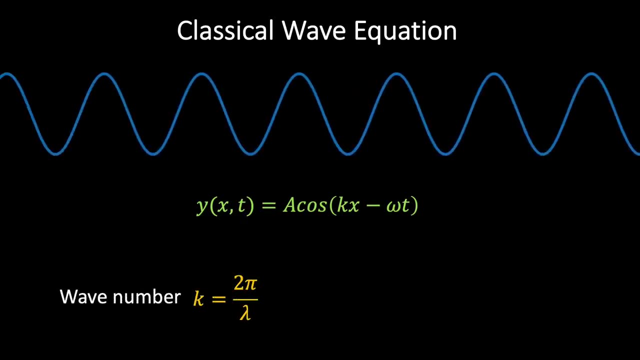 position x and time. t and a is the amplitude or maximum displacement of the wave. in this expression we have defined the wave number k as 2 pi over lambda, where lambda is the wavelength, and we've also defined the angular frequency, omega, as 2 pi f, where f is the frequency of oscillation or vibration. 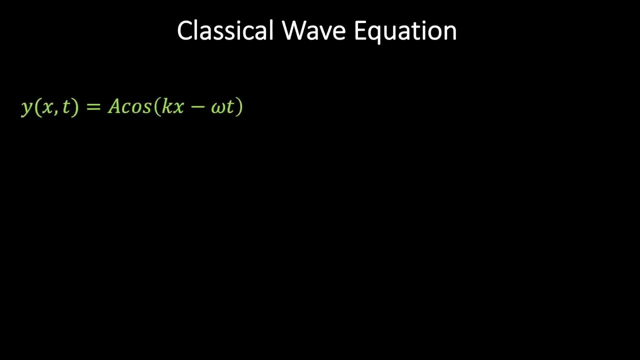 of the wave. now, this displacement function is a solution to a general wave equation which takes the following form: it's worth noting that this equation involves partial derivatives, which are represented by the curly d symbol. in the wave equation, the displacement function y is a function of two variables, x and t, and so it's appropriate to use the partial derivative. 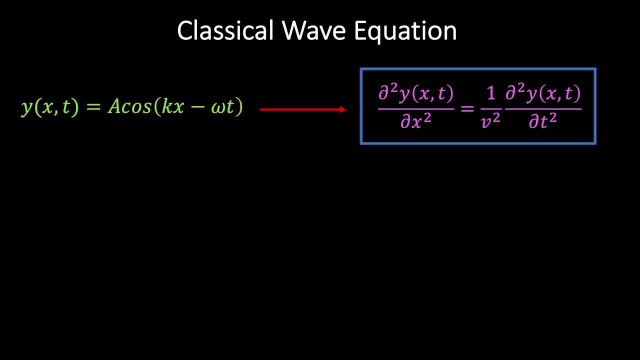 symbol when differentiating with respect to one of the variables, we can confirm that the cosine wave function is indeed a solution to this wave equation by substituting it into the equation. if we take the first and second derivative of the wave displacement relation with respect to time, 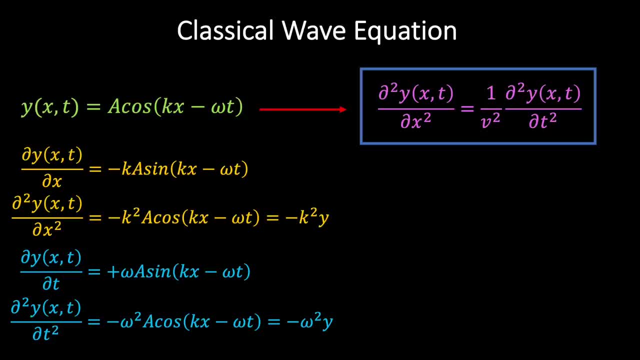 and space, we get the following result: this expression works to understand the expansion variant relations. and then, if we sub these back into the wave equation, we find the following green expression: If we then divide both sides by y, we find that v squared equals omega squared. 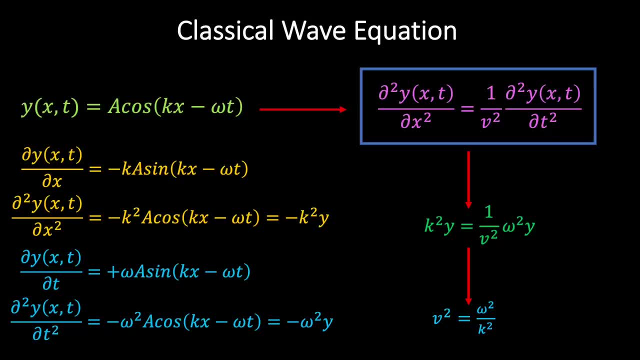 over k squared, and therefore we see that this displacement function is indeed a solution to the wave equation, provided that v equals omega over k. If we then substitute in the definitions of omega and k, we see that this constraint is none other than the famous velocity. 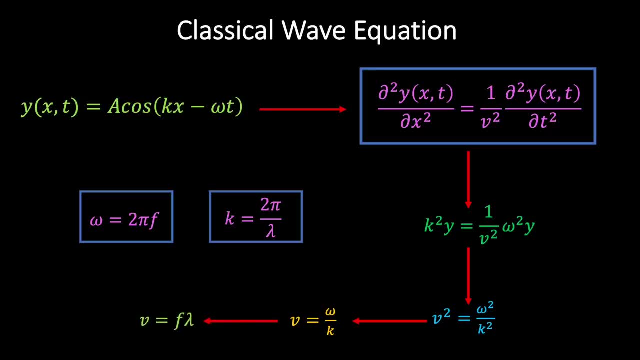 frequency and wavelength relation v equals f lambda. Now it's worth emphasising a few points at this stage. We see that the structure of the wave equation has ensured that the expected wave function is indeed a solution, and it's also ensured that we arrive at the correct relationship between velocity, frequency and 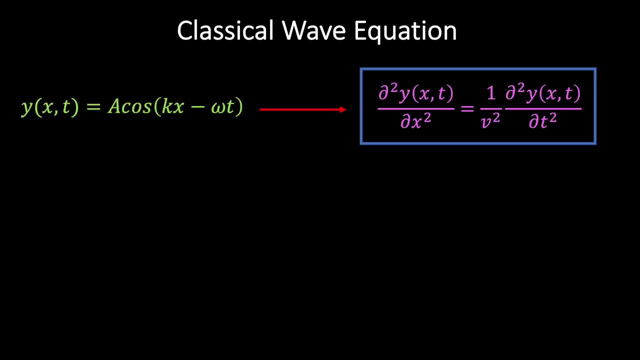 wavelength. This can ultimately be traced back to the fact that when we differentiated twice with respect to space, we got a factor of k squared, and when we differentiated twice with respect to time, OK, we got a factor of omega squared, and therefore we found that v squared equals omega squared over k. 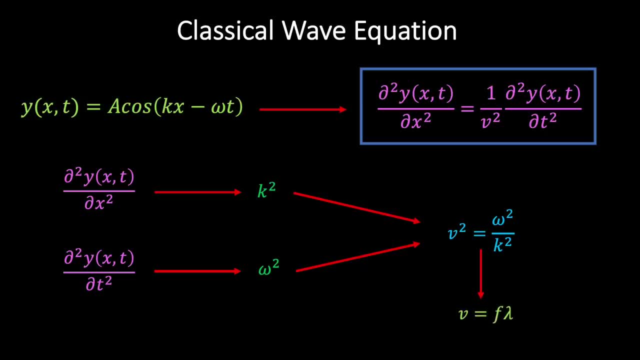 squared, from which it followed that v equals f lambda. And so, to summarise, we have seen that a wave function is a solution to a wave equation, provided that a certain relationship between frequency and wavelength holds true. And for the classical wave, we've considered: 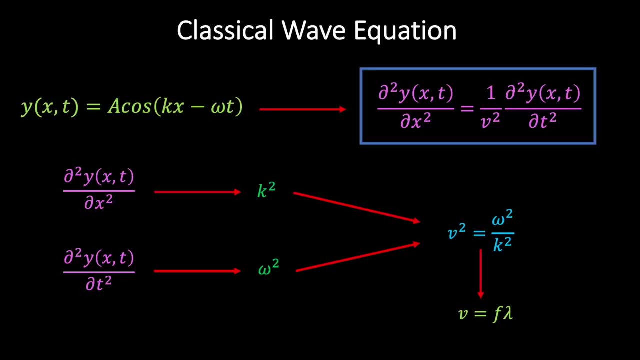 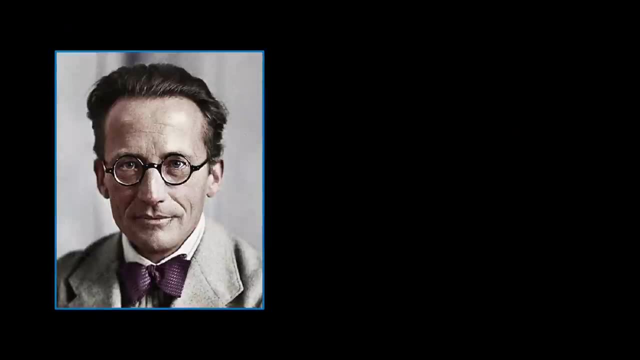 this relationship between wavelength and frequency is precisely what we expect for a travelling wave, And it was this relationship between wave function and wave equation that Schrodinger started thinking about in 1925.. If de Broglie was correct and particles behave like 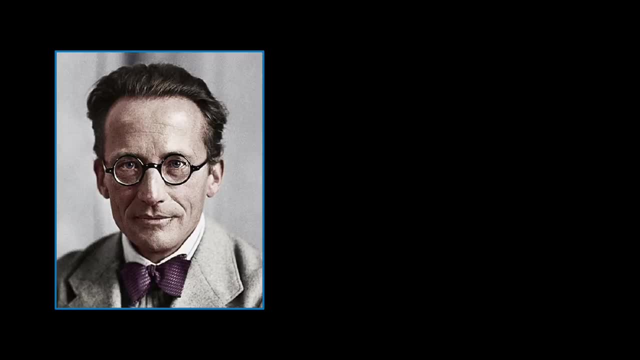 waves, then these de Broglie wave functions should be solutions to a wave equation. If so, what form should this wave equation take? Would it have the same form as the classical wave equation we've just seen? And if not, why not? Now, if a freely moving particle is a solution to a wave equation, then it should be a solution to a wave equation. Now, if a freely moving particle is a solution to a wave equation, then it should be a solution to a wave equation. 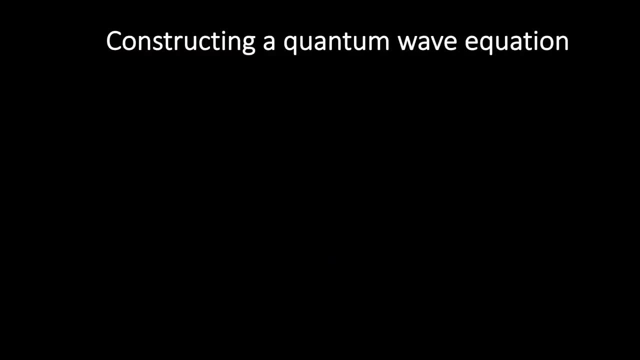 If a freely moving particle is to be described by an associated wave, then a reasonable first guess would be to suggest that the wave is described by a progressive travelling wave which, as we've already seen, can be described by the following function. This makes sense as a first guess, since this function describes a wave with fixed frequency. 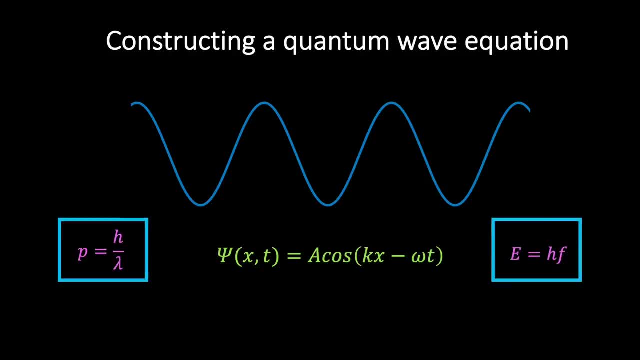 and wavelength and, according to the Einstein-De Broglie relations, if the wavelength and frequency is constant, then so is the momentum and energy, as would be expected for a freely moving particle. However, if a force were to act upon the particle, 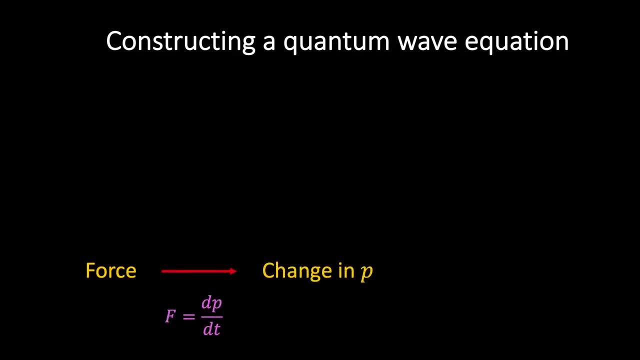 then, according to Newton's second law, the particle's momentum would change and therefore, according to the de Broglie postulate, lambda equals h over p. the wavelength associated with the particle will also change. However, the concept of wavelength is not well defined. if it changes very rapidly, It's difficult. 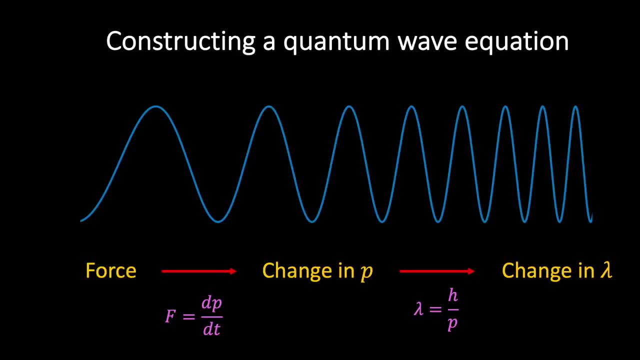 to define even a variable wavelength, since the separation between adjacent maxima is not equal to the separation between the adjacent maxima and the separation between the adjacent maxima and the separation between adjacent minima. To put this another way, if the linear momentum of 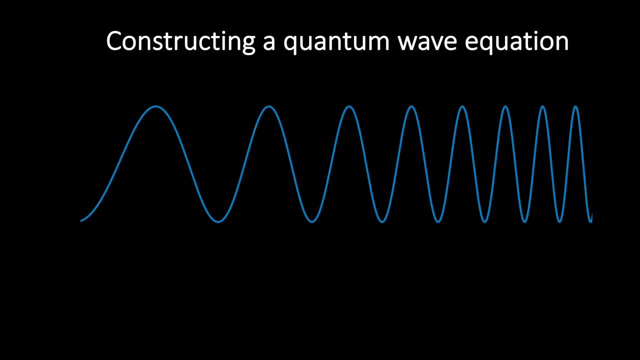 a particle is not of constant magnitude, because the particle is acted on by a force, then functions which are more complicated than a cos are required to describe the associated wave. The challenge facing Schrödinger was to develop a wave equation that could determine the wave. 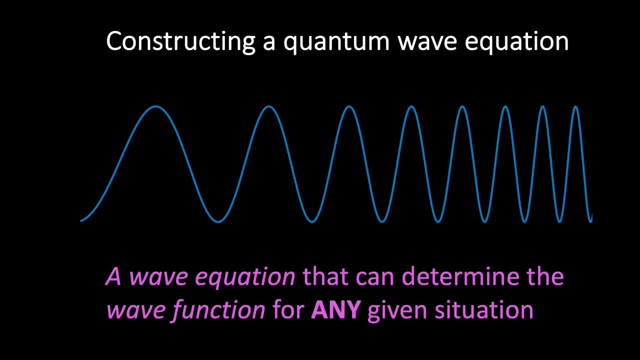 function for any given situation. In other words, Schrödinger wanted to develop a wave that tells us the form of the wave function if we tell it information about the force acting on the associated particle. And the way that we do this is by specifying the potential energy corresponding to the force. 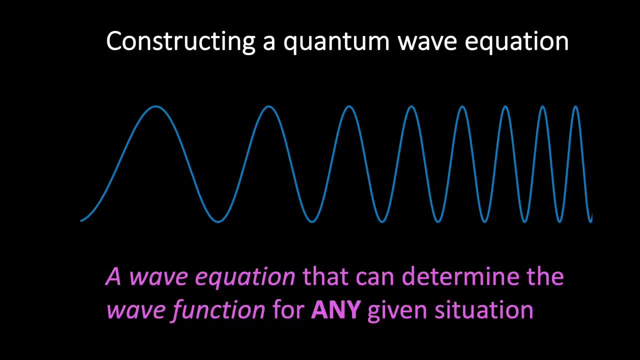 Now, as we've already seen with classical wave equation, the most common type of equation which has a function for a solution is a differential equation, And so it's a differential equation that we shall seek To help us construct a suitable quantum mechanical wave equation. 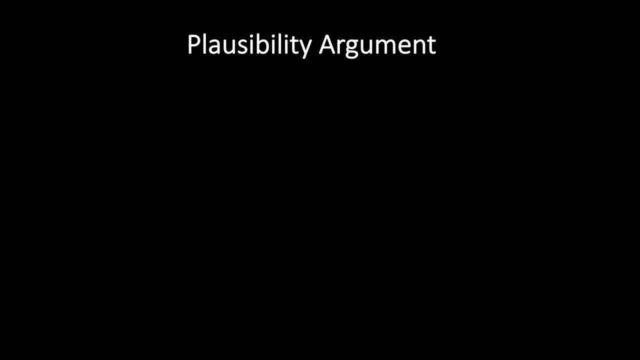 we're going to make a few reasonable assumptions. Firstly, the wave equation must be consistent with the de Broglie-Einstein postulates, which connect the wavelength lambda of the wave function with the linear momentum p of the associated particle and the frequency f of the wave function with the total energy e of the particle. 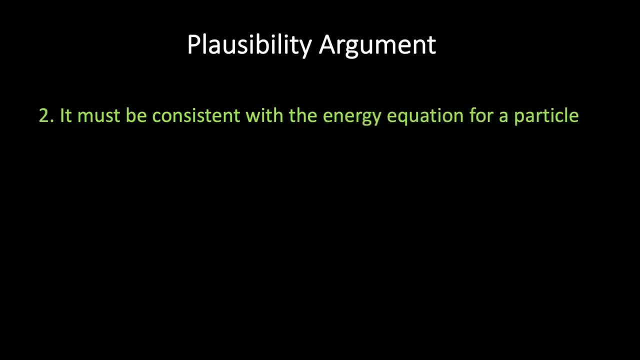 Secondly, it must be consistent with the energy equation for a particle, which states that the total energy e of the particle should be the sum of the kinetic and potential energies. Now we can write the kinetic energy, half mv, squared in terms of the momentum, as p squared over 2m. 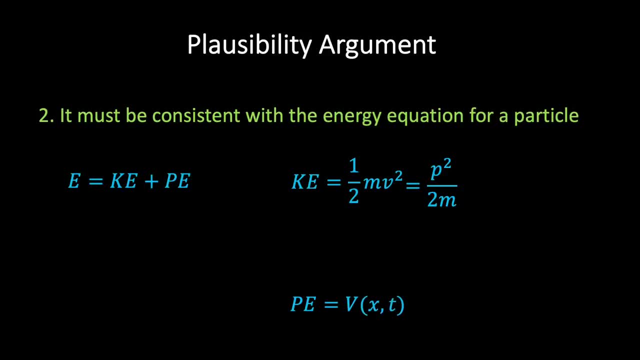 And we can write the potential energy as v of xt. As you may remember from classical mechanics, by specifying the potential energy, we are providing information about the forces acting on the particle, since the force is simply the derivative of the potential energy function. 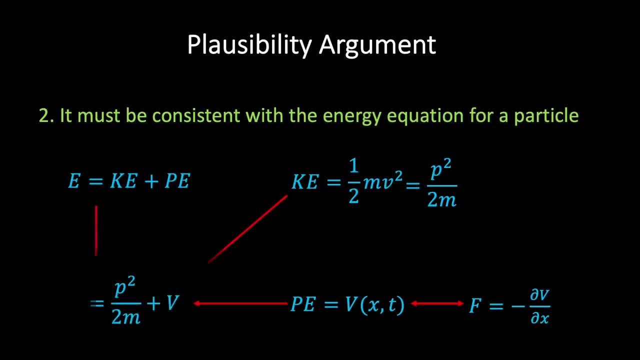 And therefore we can write the total energy of the particle as: e equals p squared over 2m plus v, where v is our potential energy function. Thirdly, our equation must be linear in the wave function, psi, That is, if psi 1 and psi 2 are two different solutions to the equation. 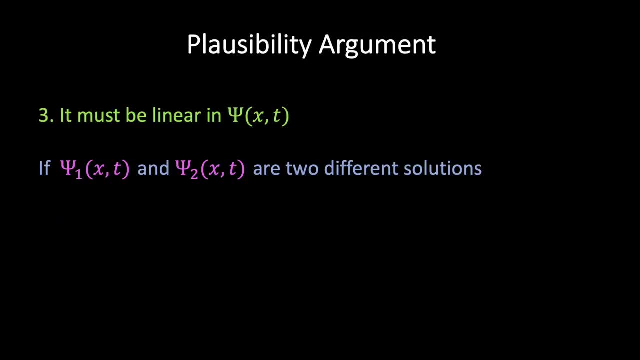 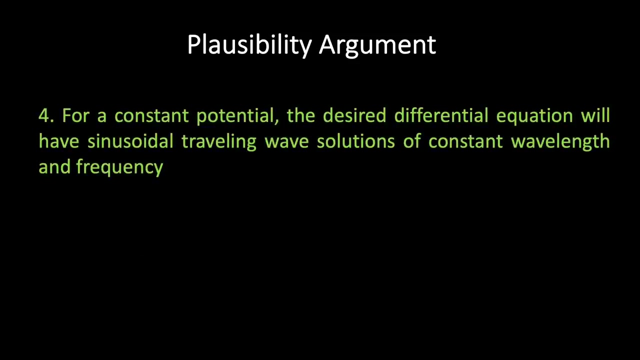 for a given potential energy, v- then any arbitrary linear combination of these solutions should also be a solution. This linearity requirement ensures that we should be able to add together wave functions to produce constructive and destructive interference patterns that are characteristic of waves, And the final assumption is that when the potential energy is constant, 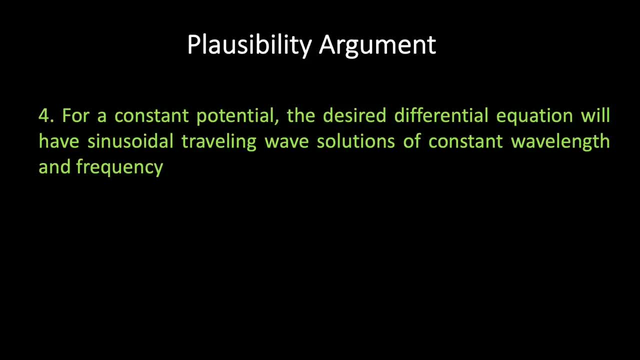 the desired differential equation should have a sinusoidal travelling wave solution of constant wavelength and frequency. This follows from the fact that if the potential energy is constant, then the force acting on the particle moving in this potential will be equal to zero, since the force is equal to the derivative of the potential energy function. 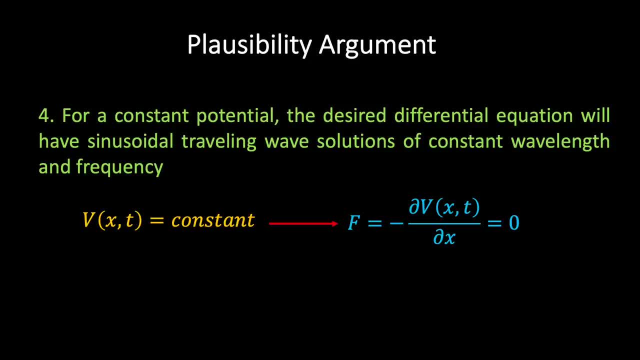 And if there is no force acting on the particle, then Newton's second law of motion tells us that the linear momentum p and the total energy e of the particle will be constant, as is the case for a freely moving particle, And we've already seen from the de Broglie-Einstein relations. 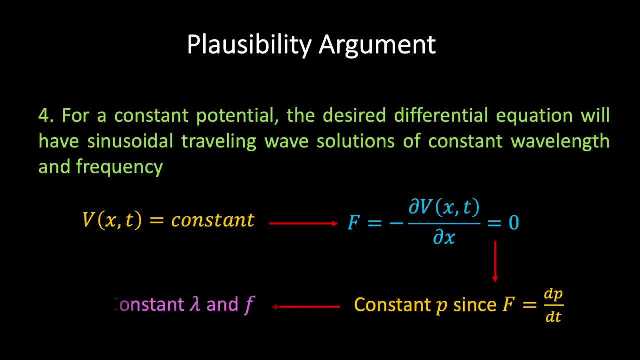 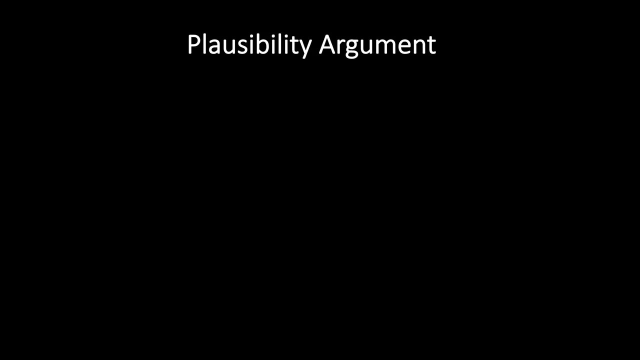 that if the momentum and energy are constant, then the associated wavelength and frequency are constant. We therefore assume that in this case, the desired differential equation will have sinusoidal travelling wave solutions of constant wavelength and frequency, as already discussed. So let's now use these assumptions to arrive at an expression for the Schrödinger wave equation. 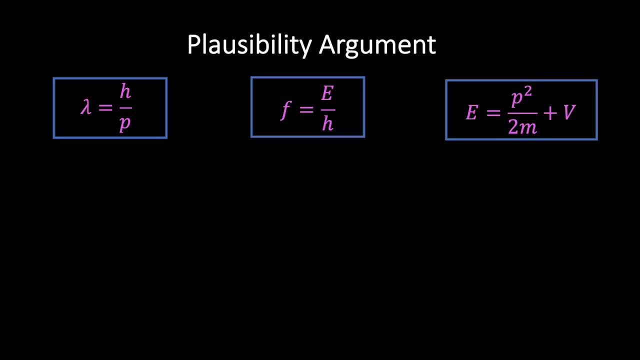 Firstly, if we rewrite the energy relation using the de Broglie-Einstein postulates, we find the following yellow expression: Now, before proceeding any further, it will prove convenient to rewrite this expression in terms of the angular frequency omega and the wave number k. 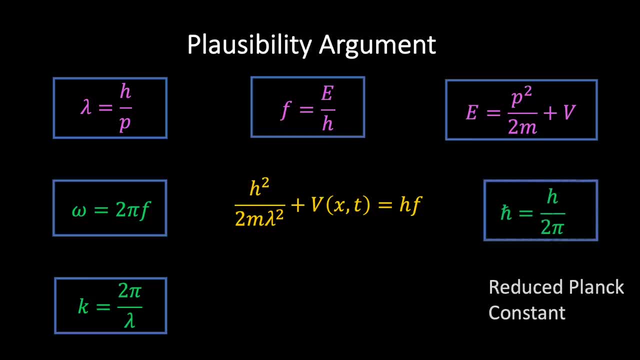 as well as the reduced Planck constant h-bar. These relations are useful because they keep variables out of the denominators of expressions and they absorb a factor of 2 pi that would otherwise appear every time we write a sinusoidal wave function. Subbing these relations into our energy expression: 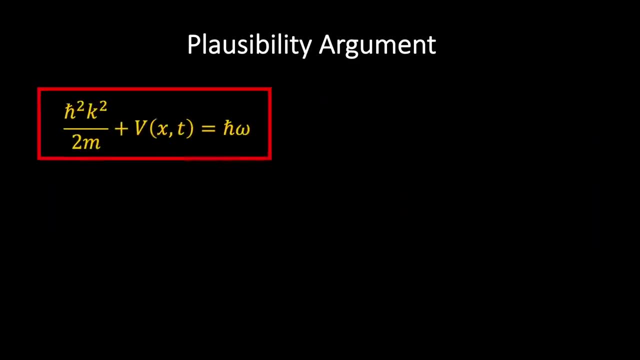 we find the following result. Notice that we have a factor of k squared on the left-hand side and a factor of omega on the right-hand side of this expression. Now, if you recall, our fourth assumption suggested that when the potential energy is constant, 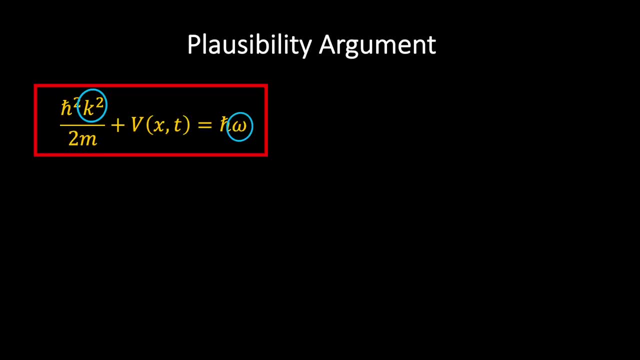 we have a freely moving particle and therefore the desired differential equation should have sinusoidal travelling wave solutions, And so we will begin by assuming that our wave function has the following form. Next, notice that when we differentiate this wave function twice with respect to x, we obtain a factor of k squared. 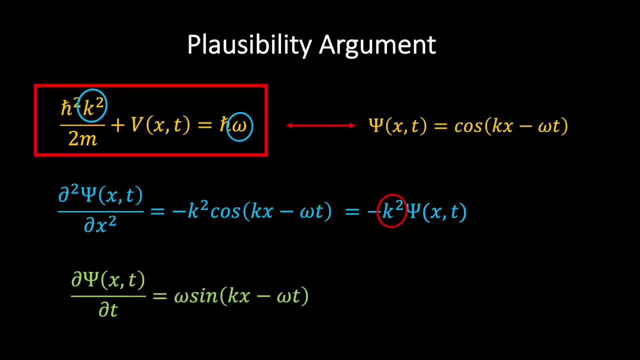 and the effect of taking the first time derivative is to introduce a factor of omega And since the differential equation we seek must be consistent with the expression in the red box, which contains a factor of k squared in one term and a factor of omega in another, 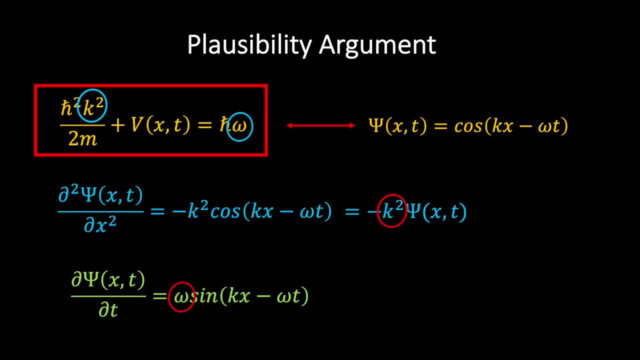 these facts suggest that the differential equation that we seek should contain a second derivative with respect to x and a first derivative with respect to time. In addition, there must be a term containing the potential energy function and, in order to ensure linearity, this term must contain a factor of the wave function. 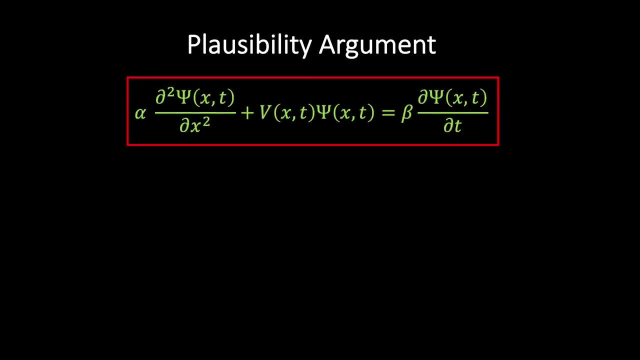 Putting all these ideas together, we are led to a differential equation of the following form, where we have introduced two constants, alpha and beta, to provide a bit of flexibility. Our job is to fix these constants by ensuring that our proposed wave function and wave equation 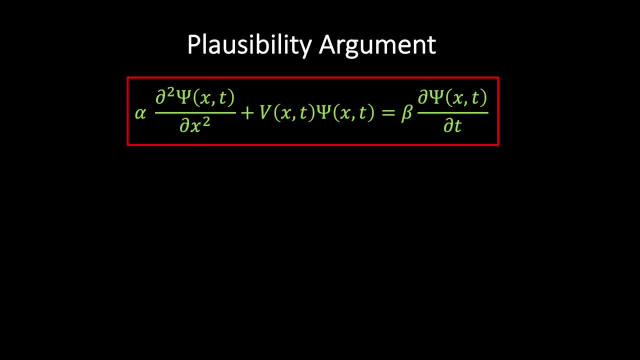 is consistent with the de Broglie-Einstein relations. Now, since we are currently assuming a freely moving particle, we will set the potential energy to a constant value. If we then sub in our proposed wave function into our proposed wave equation, we find the following result: 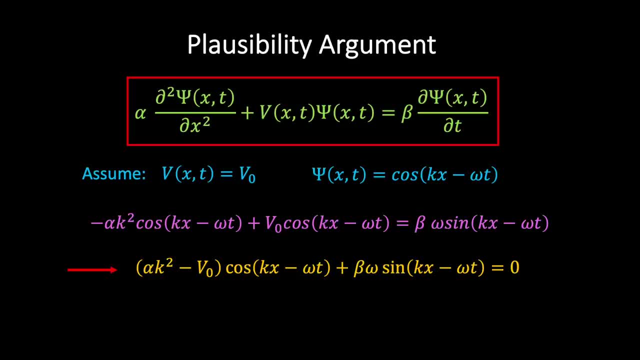 which we can then write in the following form: Now, an immediate problem with this result is that we have a mixture of sine and cosine terms, and so, in order for this equation to be satisfied, for all values of x and t requires that the coefficient of each term is separately equal to zero. 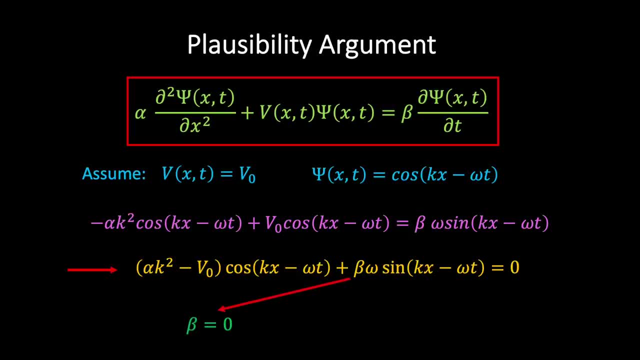 In which case we are forced to set beta equal to zero and k squared equals v naught over alpha, And we clearly see that there is no way of recovering the required de Broglie-Einstein relation. So what's gone wrong? 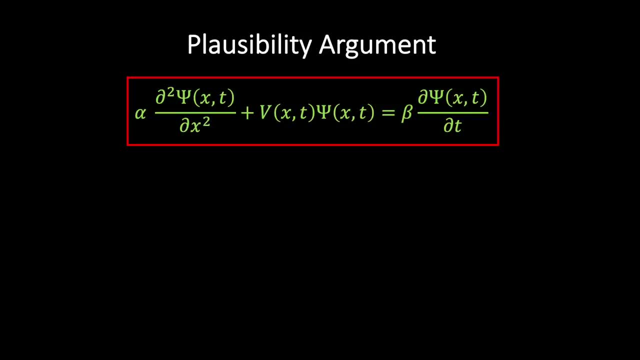 Well, part of the difficulty can be traced back to the fact that differentiation changes cosines into sines and vice versa, And since we are differentiating once with respect to time and twice with respect to space, we end up with a mix of sine and cosine terms. 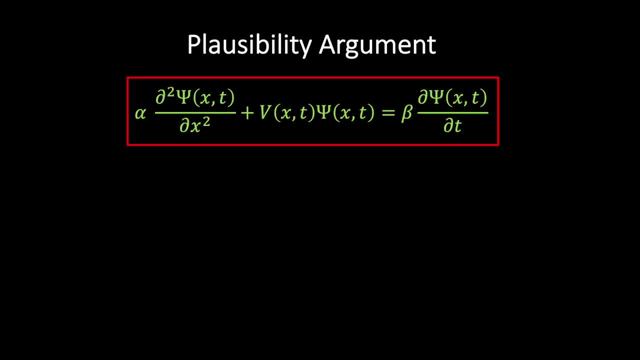 Furthermore, we've been quite restrictive with our initial choice of wave function. If you recall, we simply borrowed the wave function result from classical physics, So perhaps we should try using a combination of cosine and sine functions to specify our free particle wave function. 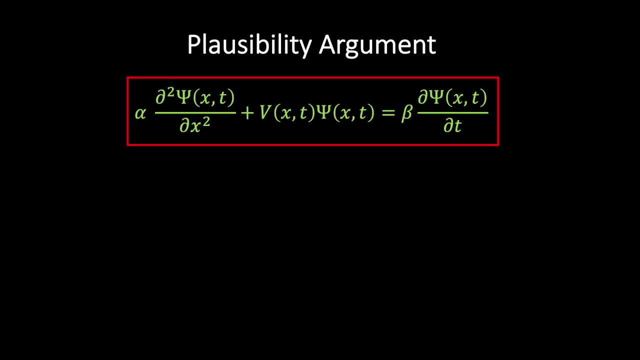 With this in mind, let's consider a more general wave function of the following form. Here, gamma is a constant, which again provides some additional flexibility. Let's now see if this more general wave function helps us get a bit closer towards our goal. 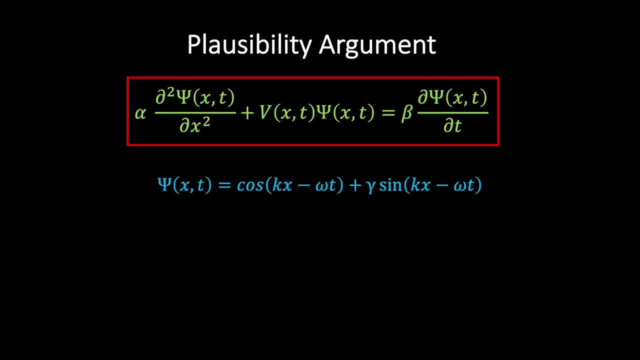 If we differentiate this function twice with respect to x, we find the following equation: And if we differentiate once with respect to time, we find the following green expression: Then, if we sub these results into our proposed wave equation, we find the following ghastly yellow result: 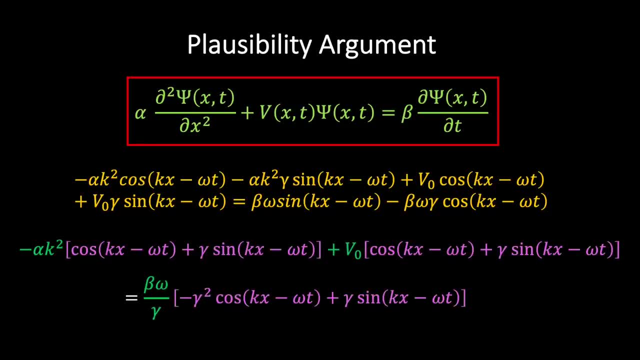 which we can rewrite in the following form: Now, hopefully, you can see that the two terms in square brackets on the left-hand side of the equation have exactly the same form as our initial proposed wave function. We also notice that the term in square brackets on the right-hand side 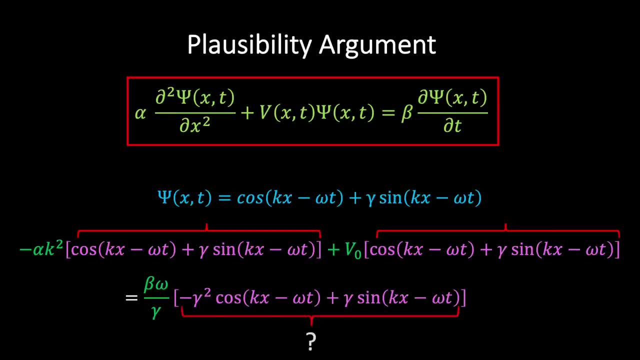 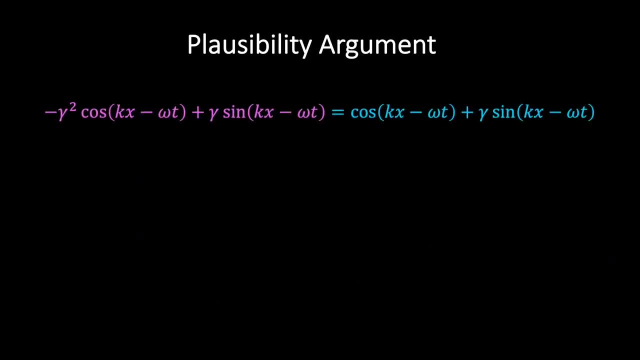 also very nearly has the same form. However, we see that the minus gamma squared term is preventing it from being exactly the same as the other terms. If we could choose gamma appropriately, then we would be able to cancel these terms from the equation and drastically simplify it. 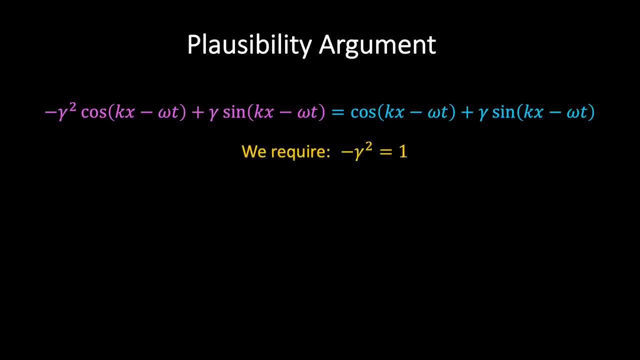 However, in order to do this, we require that minus gamma squared equals 1, and therefore gamma squared equals minus 1.. And it follows that gamma must therefore be equal to plus or minus the square root of minus 1.. Now you may, at this stage, panic. 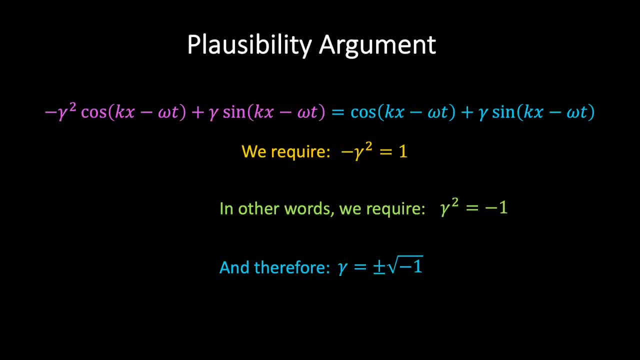 and think that something's gone terribly wrong. Surely this doesn't make sense. After all, you remember being taught at school that it's not possible to take the square root of a negative number. However, let's take this possibility seriously for a moment. 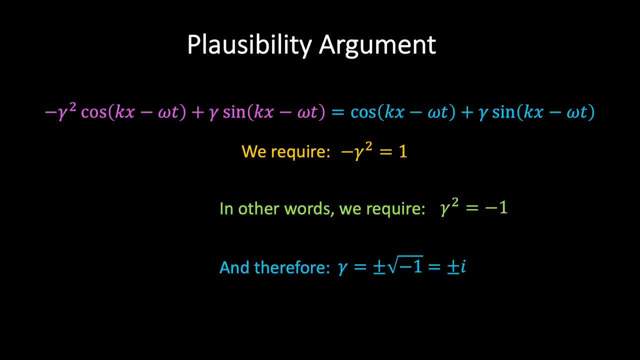 and define the square root of minus 1 as being equal to i, where i is referred to as an imaginary number, which is simply a number with the property that i squared equals minus 1.. Now, if we look back at our original equation, 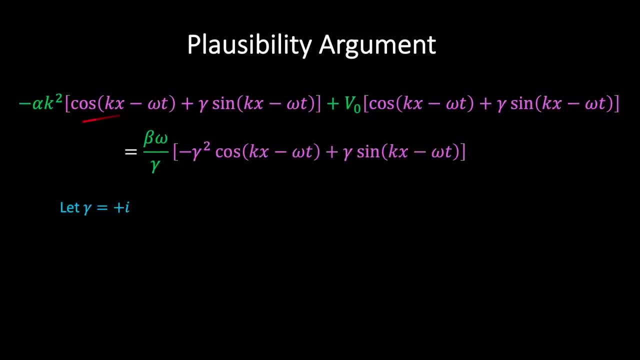 and set gamma equal to i, then we see that we can cancel square bracket terms from both sides of the equation and we then arrive at the following simplified expression: And if we then compare this with the energy-momentum relationship that we derived using the de Broglie-Einstein relation, 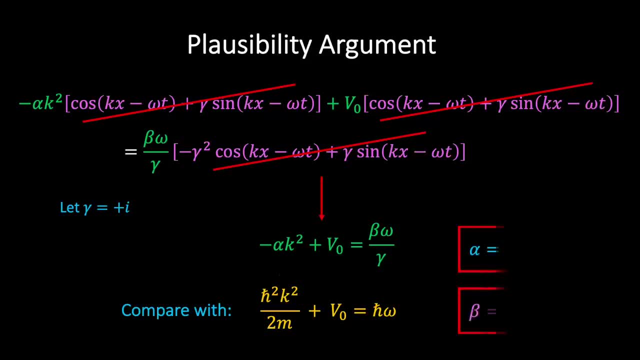 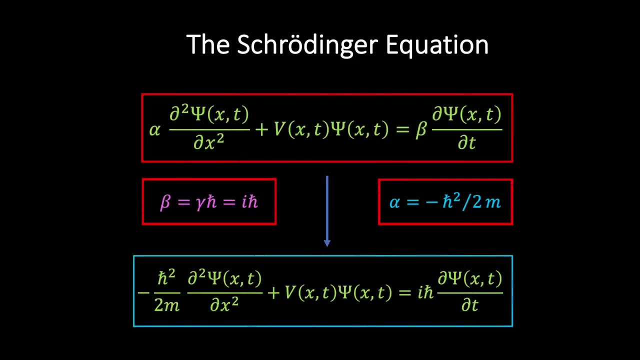 we see that we can match the two expressions if we identify alpha equals minus h-bar squared over 2m and beta equals i h-bar. If we then sub these expressions back into our proposed wave equation, we arrive at the following beautiful equation: This differential equation satisfies all four of our assumptions. 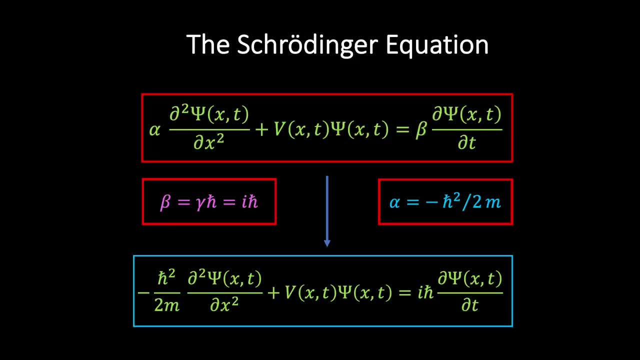 concerning the quantum mechanical wave equation. Now, it's worth emphasising that we've been led to this equation by considering the special case of a free particle with a constant potential. We will, however, postulate that the quantum mechanical wave equation has the same form in the general case. 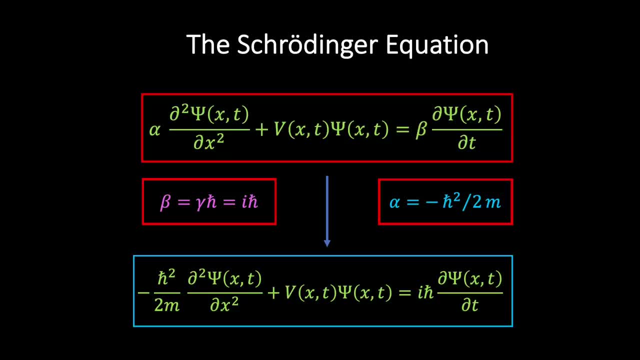 when the potential energy can vary as a function of space and time. But we cannot prove this to be true. We can, however, postulate it to be true, And the validity of the postulate will ultimately be judged by comparing its implications with experiment. 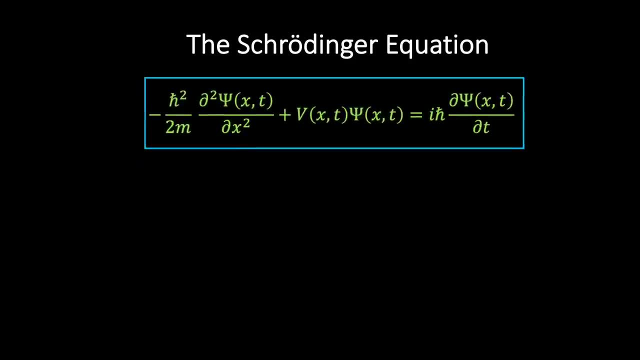 And so it seems that we've finally arrived at the desired equation: a quantum mechanical wave equation whose solutions give us the wave function which is to be associated with the motion of a particle under the influence of forces which are described by the potential energy function. v. 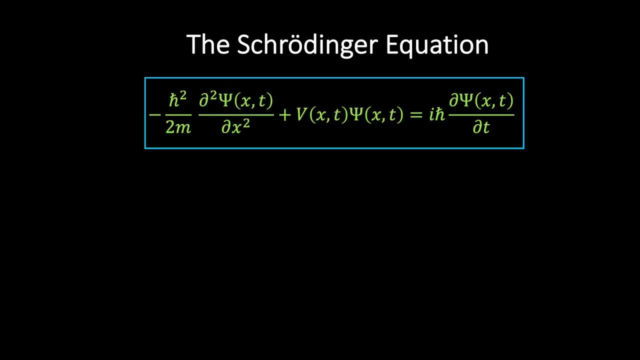 And it was this exact equation that was first obtained by Schrödinger in 1926 and which now carries his name. It's worth noting that Schrödinger was led to his equation by a more esoteric line of reasoning than the one that we've adopted here. 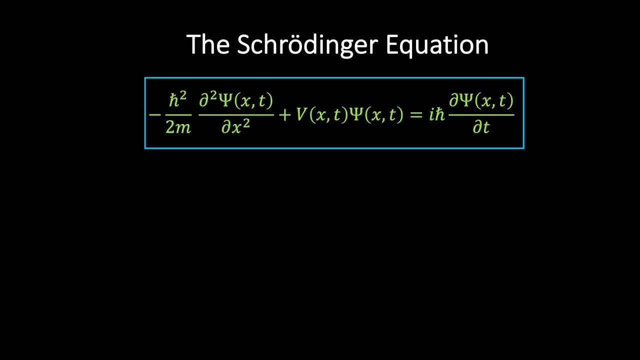 However, he was strongly influenced by the de Broglie postulate, in the same way that we have been. So what is the significance of the Schrödinger equation, and what can we use it for? Well, the basic idea is as follows. 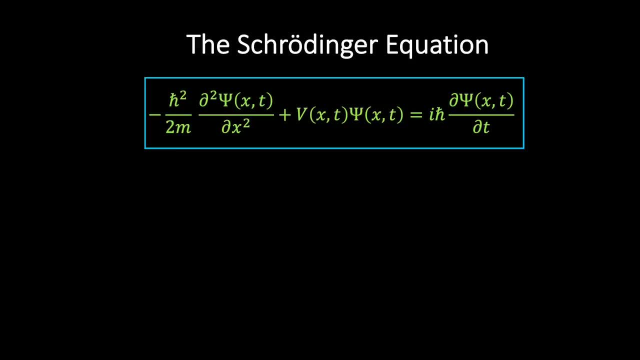 If you wish to determine the structure of the wave function associated with the particle of mass m using the Schrödinger equation, the first thing you do is to specify the potential energy function, which tells you something about the forces acting on the particle. 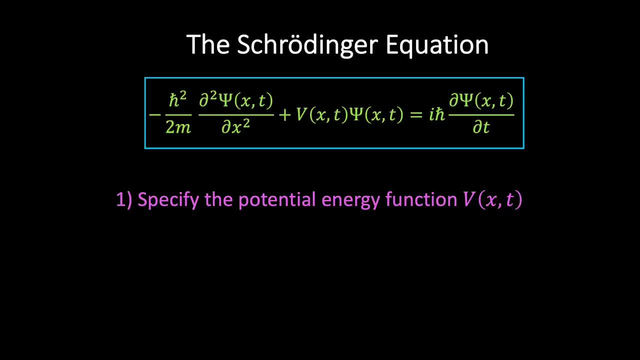 Once you've specified the potential, you then need to solve the corresponding partial differential equation to find the wave function. But what exactly does the wave function represent, And how does it relate to the particle that it's associated with? Let's now turn to this question. 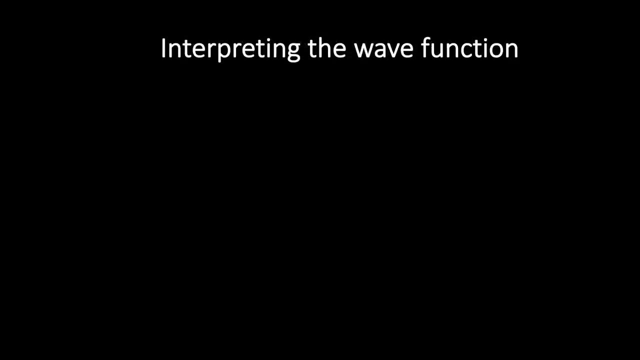 In order to answer this question, it will prove illuminating to look again at the free particle wave function that we used in our previous analysis. If you recall, we had the following expression, But we also found that this function is only a solution to the Schrödinger equation. 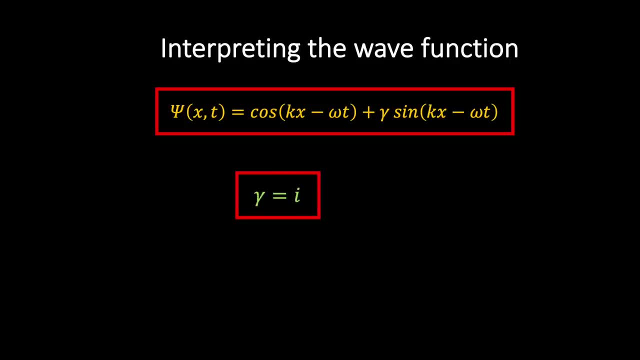 if gamma equals i And if we sub this into the wave function expression, we find the following result: We see that our wave function is a complex function, meaning that it contains the imaginary number i And, if you recall, this behaviour was forced upon us. 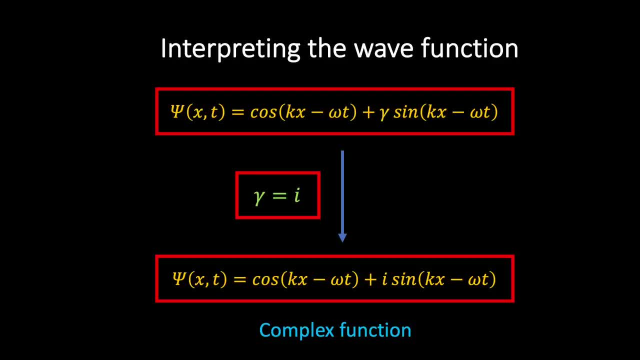 to ensure consistency with the de Broglie-Einstein postulates. Furthermore, we found that an imaginary number also appears in the Schrödinger equation itself, And this implies that, in the general case of varying potential, the wave functions which are solutions to the Schrödinger equation. 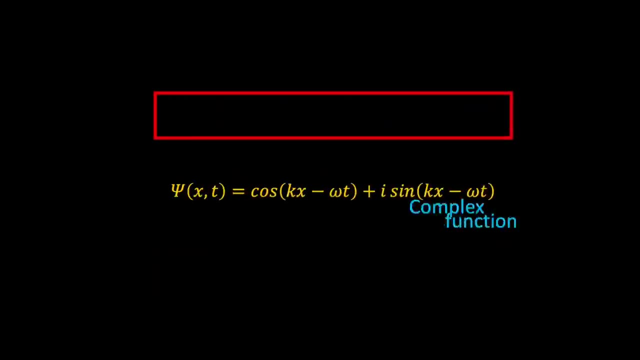 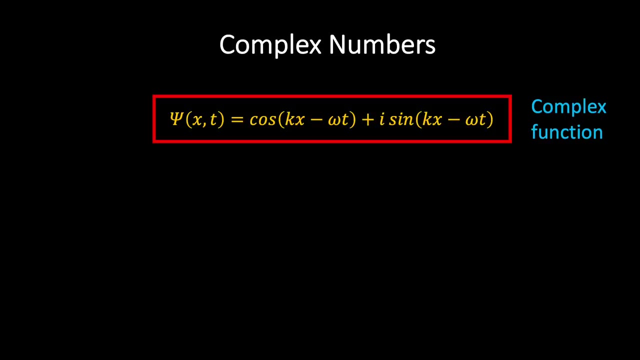 will also be complex. Now, since a general wave function of quantum mechanics is a complex function, it's worth digressing momentarily to explore complex numbers in a bit more detail. Any complex number may be written in the form: z equals a plus i b. 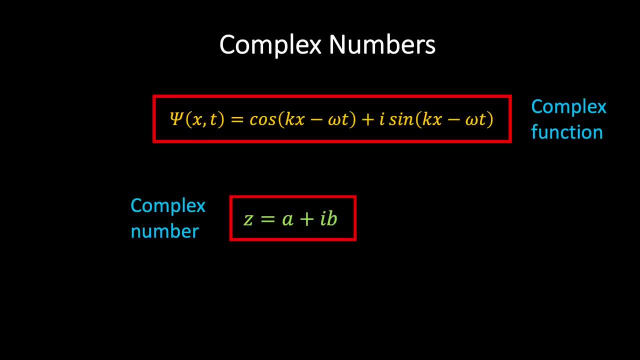 where, as we've already seen, i squared equals minus one. The number a is referred to as the real component of the complex number and the number b is referred to as the imaginary component of the complex number, And it's worth noting that both a and b are real numbers. 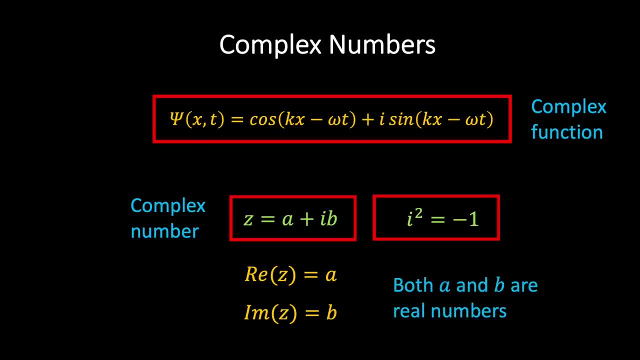 Notice that the complex wave function that we've encountered is of the form a plus i, b, and therefore it specifies simultaneously two real functions: its real part and its imaginary part. This is in contrast to a wave function of classical mechanics. For instance, a wave on a string can be specified by one real function. 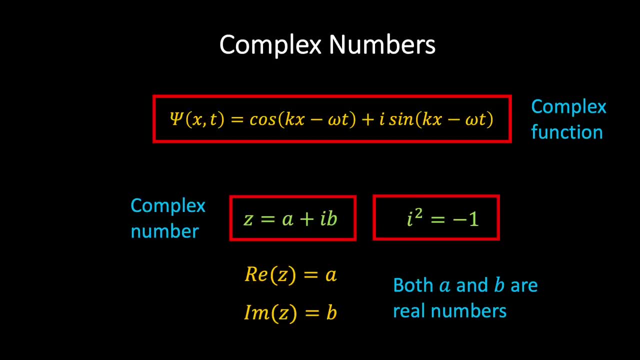 which gives the displacement of various elements of the string at various times. This classical wave function is not complex because the classical wave equation does not contain a factor of i, since it relates a second time derivative to a second space derivative. Now, one way in which we can represent a complex number: 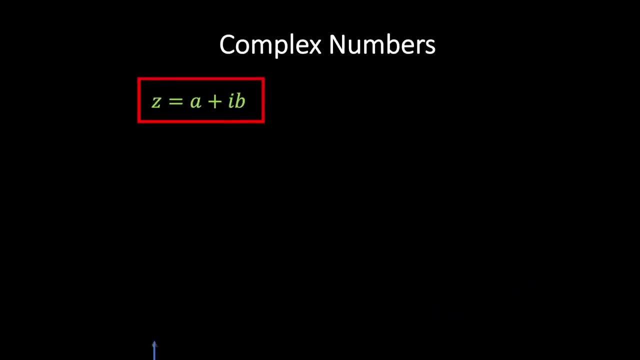 is to plot its position on a graph in which the y-axis specifies the imaginary component of the complex number and the x-axis specifies the real component. We can then plot the complex number by marking the positions a and b. Note that if we draw an arrow starting at the origin, 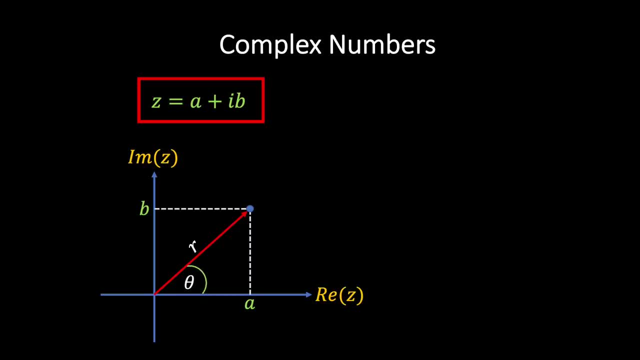 and ending at the point we plotted, then we can specify the angle theta, which is the angle the arrow makes with the real axis. If r is the length of this arrow, then we can use some simple high school trigonometry to see that the distance from the origin along the real axis 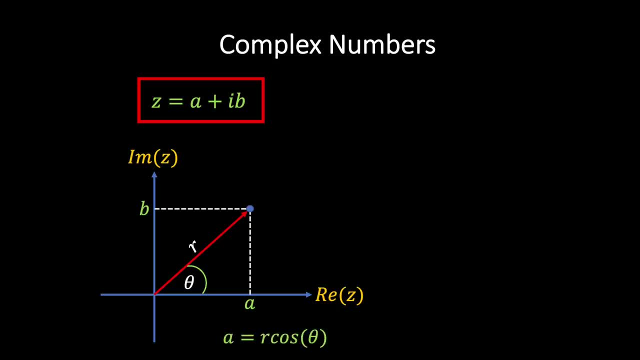 is given by r cos theta, and this is simply a, and the distance along the y-axis is given by r sin theta, which is simply b. If we then sub these expressions, along for a and b, back into the expression, z equals a plus ib. 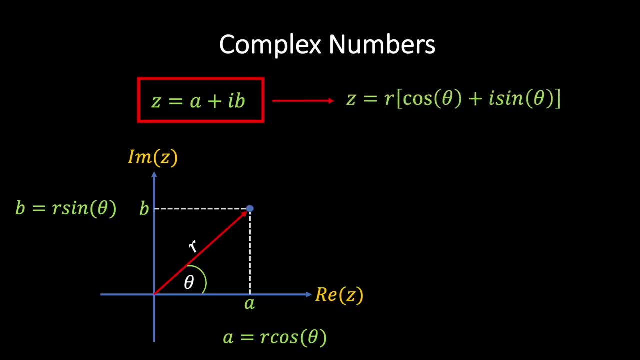 we get the following green result. Next, if we set r equals 1 and theta equals kx minus omega t, then we recover the complex wavefunction that we had before. Now, if you have a complex number of the form, z equals a plus ib. 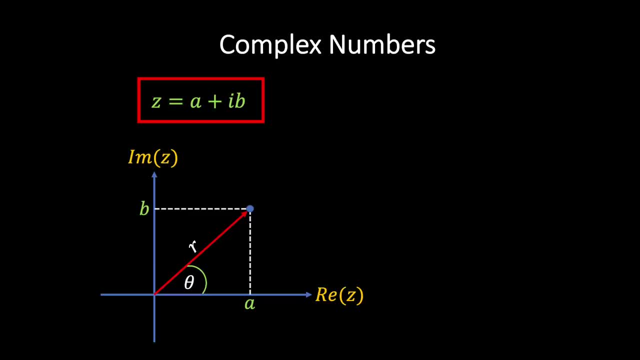 then it's possible to perform an operation on this number, which is referred to as taking the complex conjugate. This operation simply involves replacing i with minus i, and it's represented by the asterisk symbol Armed with the complex conjugate operation. 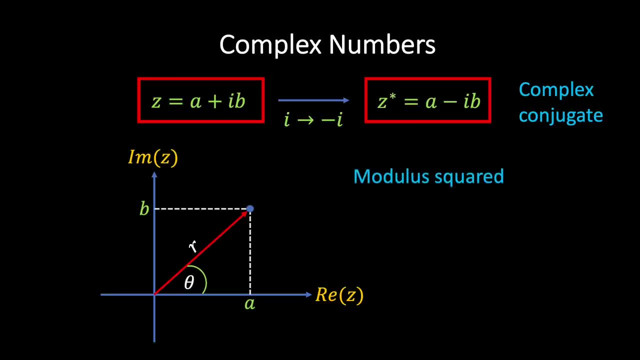 we can then calculate the modulus squared of a complex number, which involves multiplying a complex number with its complex conjugate. In our example, we see that the modulus squared of z can be written as a plus ib times a minus ib, which simplifies to a squared plus b squared. 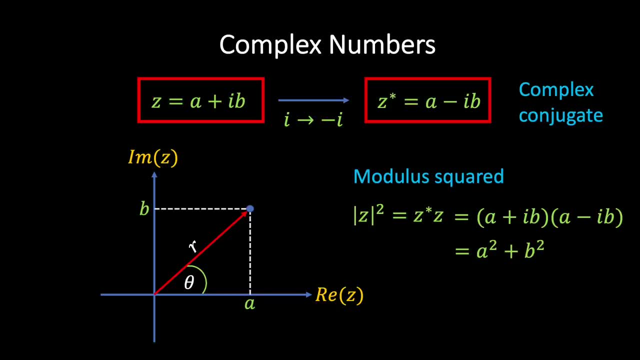 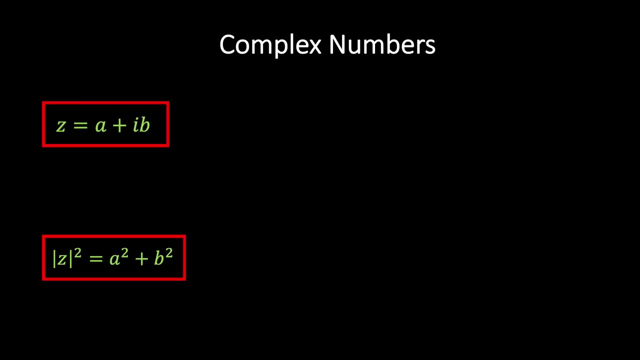 Now, the important thing to note about this expression is that the modulus squared of a complex number is a real number that can never be negative. This will have profound consequences for our interpretation of the wavefunction in what follows Now the fact that wavefunctions are complex functions. 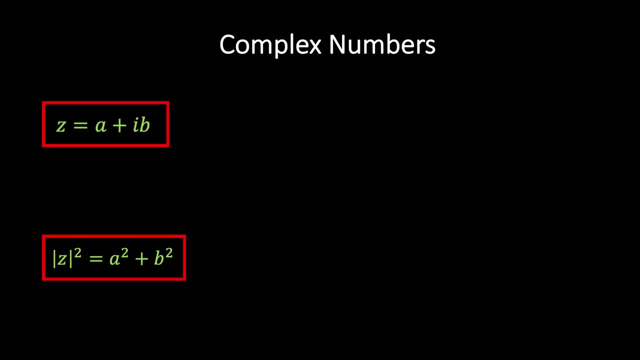 should not be considered a weak point of the quantum mechanical theory. Actually, it's a desirable feature, because it makes it immediately apparent that we should not attempt to assign a physical existence to wavefunctions in the same sense that water waves have a physical existence. 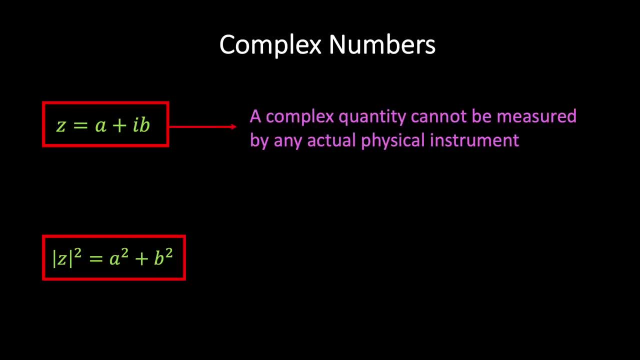 The reason is that a complex quantity cannot be measured by any actual physical instrument and therefore the quantum wavefunction is not a measurable quantity. So what does this complex wavefunction represent if it corresponds to no physical measurable quantity? After all, a particle, by its nature, is localised at a point. 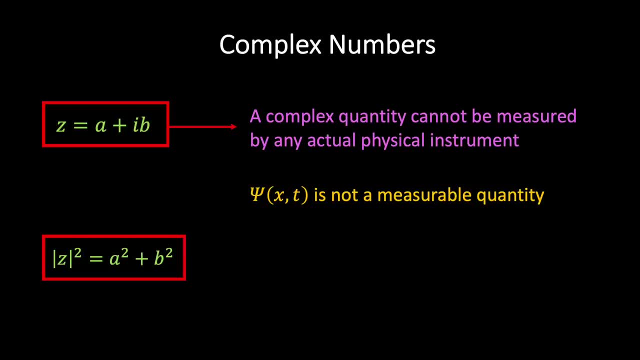 whereas the wavefunction, as its name suggests, is spread out in space. Well, a hint to answering this question lies in the fact that, as we've just seen, the modulus squared of a complex number represents a real number. So perhaps the modulus squared of the wavefunction 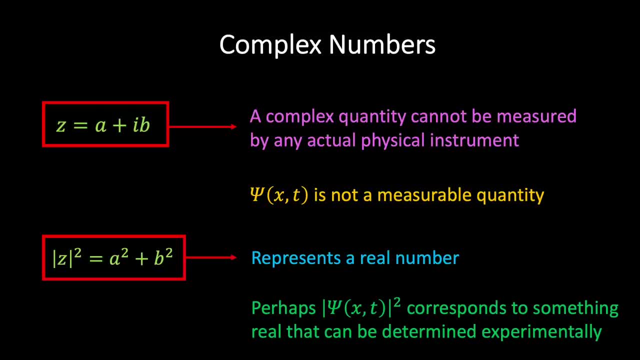 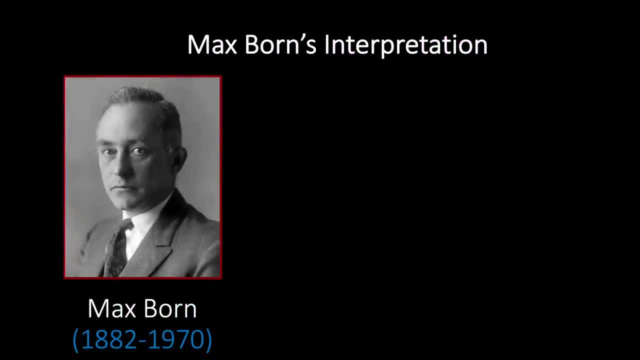 corresponds to something real that can be determined experimentally. In 1926, the physicist Max Born suggested that the modulus squared of the wavefunction represents the probability of finding a particle at a particular location in space. In other words, if at some instant in time, t 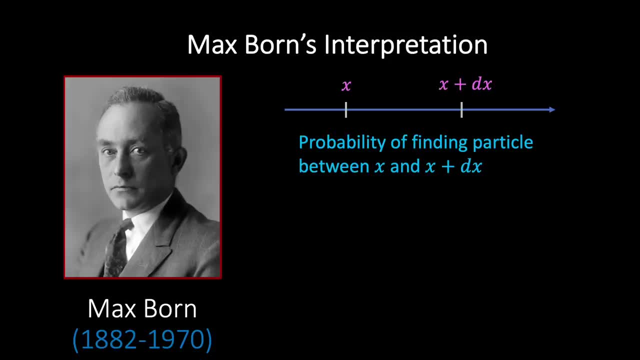 a measurement is made to locate the particle associated with the wavefunction, psi, then the probability that the particle will be found at a coordinate between x and x plus dx is given by the following green expression: where, as we've just seen, the modulus squared of the wavefunction. 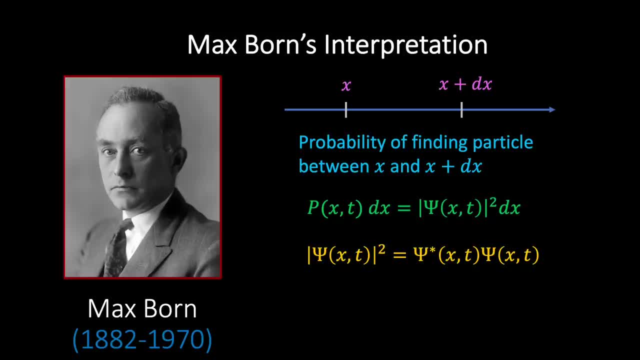 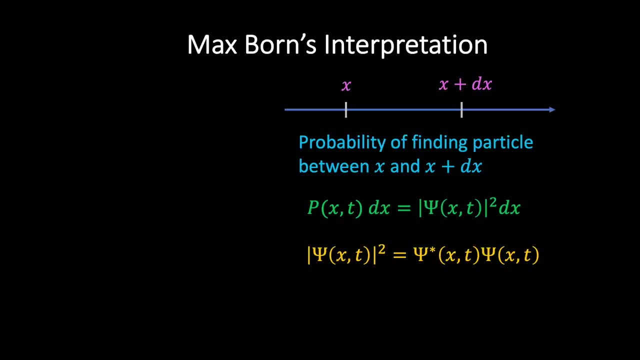 is calculated by multiplying the wavefunction by its complex conjugate. If we then want to find the probability that the particle is located within a given region, we simply need to integrate the modulus squared. So, for example, the probability of finding a particle. 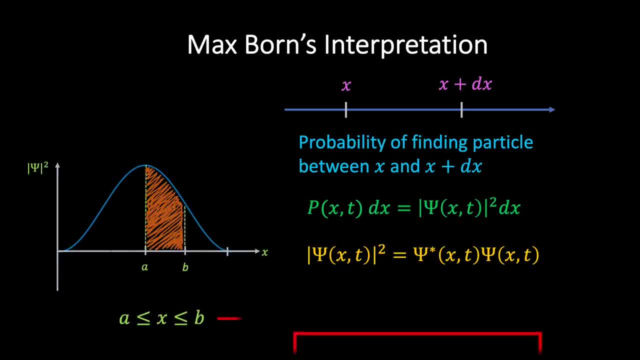 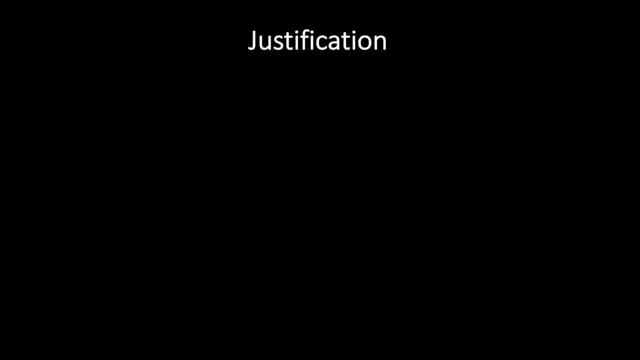 located between two points. a and b is given by the integral of the modulus squared, evaluated, with a and b as the limits of the integral. The justification of Born's postulate can be found in the following considerations: Since the motion of a particle is connected, 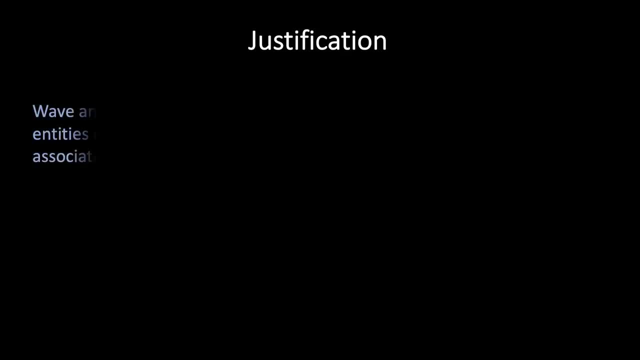 with the propagation of an associated wavefunction. these two entities must be associated in space, That is, the particle must be at some location where the waves have an appreciable amplitude and therefore the probability density must have an appreciable value, where the wavefunction has an appreciable value. 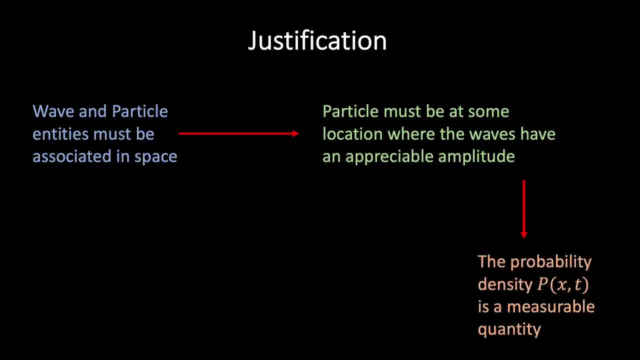 Furthermore, since the probability density is a measurable quantity, it should be a real, positive-valued number, whereas the wavefunction is in general complex And therefore it's obviously not possible to equate the probability simply with the wavefunction itself. 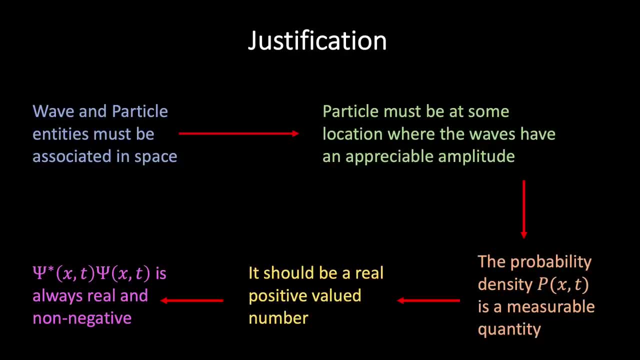 However, since the modulus squared of the wavefunction is always real and non-negative, Born had reason to believe that it referred to a measurable quantity. So what's this all telling us? Born's interpretation introduces a kind of indeterminacy into quantum mechanics. 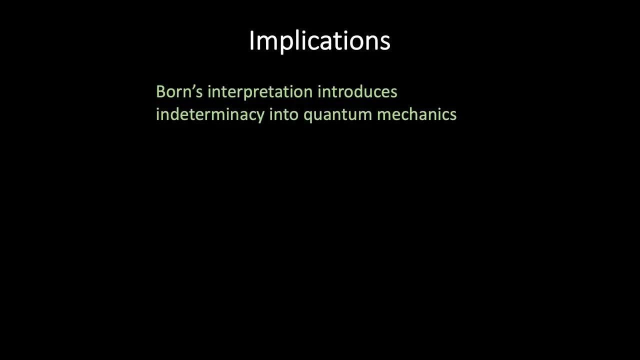 for even if you know everything the theory has to tell you about the particle, you still cannot predict with certainty the outcome of a simple experiment to measure its position. All that quantum mechanics can offer is statistical information about the possible result of measurements. This indeterminacy has been deeply disturbing. 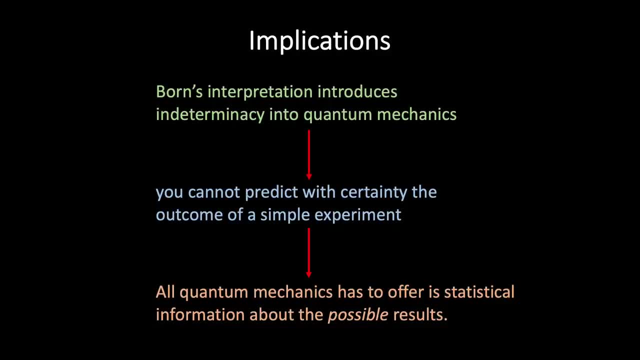 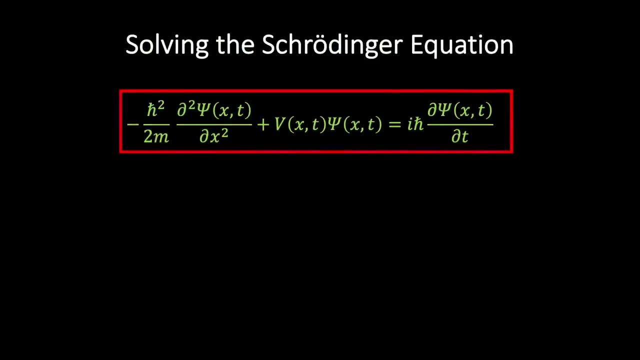 to physicists and philosophers alike, and it's natural to wonder whether it's a fact of nature or a defect of the theory itself. Now, I think you might agree that this discussion so far has been rather abstract, and so I think it would prove useful. 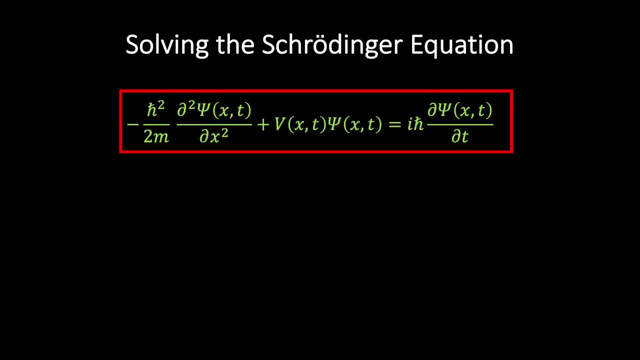 if we ground the remainder of this video in a series of concrete examples which explicitly show how the Schrodinger equation can be used to calculate various useful properties. And so our first step is to figure out how to actually solve the Schrodinger equation. 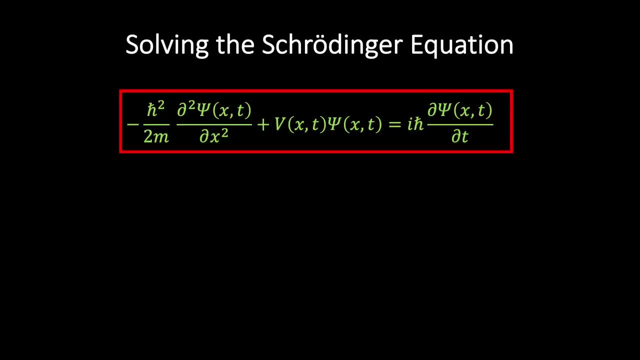 Now, the standard technique we will use is referred to as the separation of variables and involves searching for solutions in which the wavefunction can be written as a product of two terms, where the first term is a function of x alone and the second term is a function of t alone. 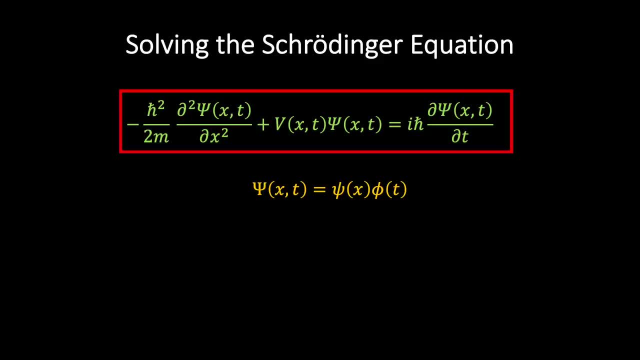 Now it's worth noting that this method is only valid if the potential energy is independent of time. But since most physicists think that physical systems of interest have potential energies of this form, the condition is not a very serious restriction. Now, if we substitute our expression for psi. 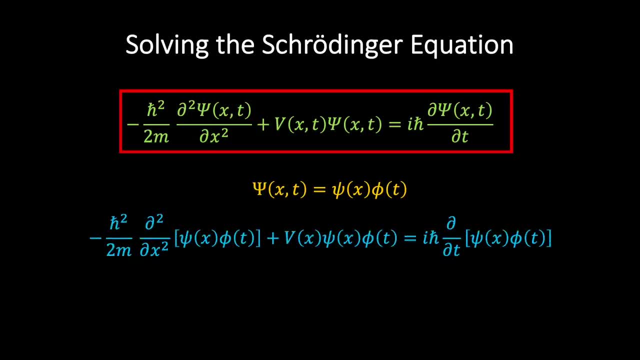 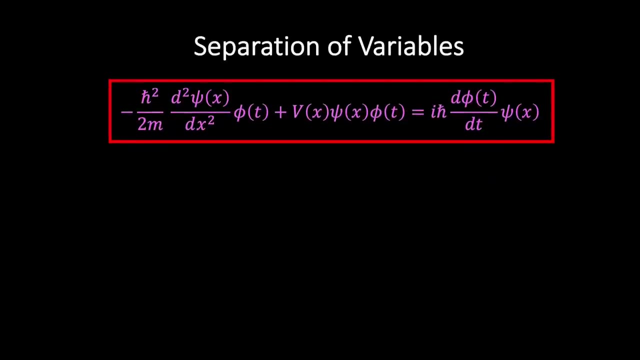 into the time-dependent Schrodinger equation, we find the following blue equation: If we then act with the derivatives on the terms inside the square brackets, we find the following purple expression: Next, we want to rearrange this expression so that all the terms involving x 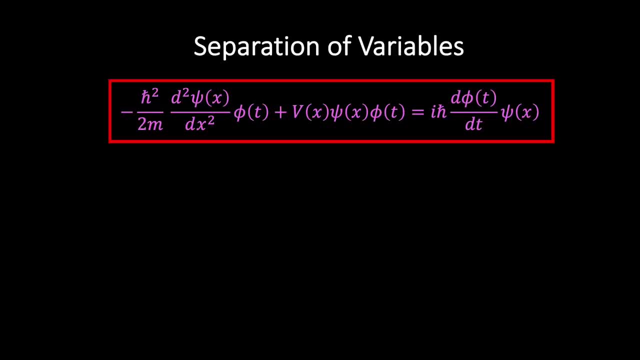 are on the left-hand side and all the terms involving t are on the right-hand side. A simple rearrangement then leads to the following yellow expression: Since the right-hand side does not depend on x, while the left-hand side does not depend on t, 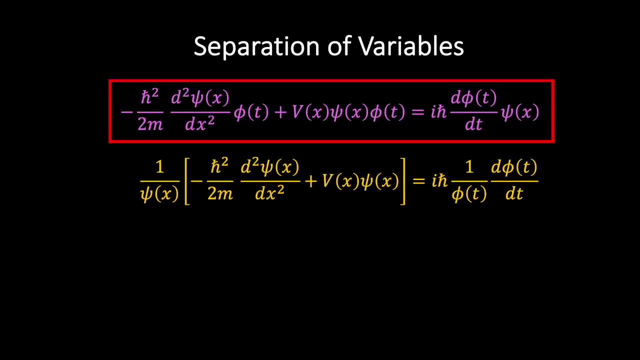 their common value cannot depend on x or t. In other words, the common value must be a constant, which we shall call k, And so we can write two equations involving k: a space-dependent equation and a time-dependent equation. The constant k is called the same. 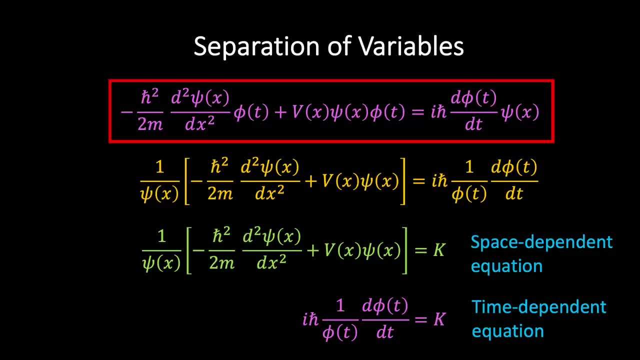 separation constant, and we see that the effect of employing this technique has been to convert the single partial differential equation involving two independent variables- x and t- into a pair of ordinary differential equations, one involving x alone and the other involving t alone. Let's now focus on this time equation. 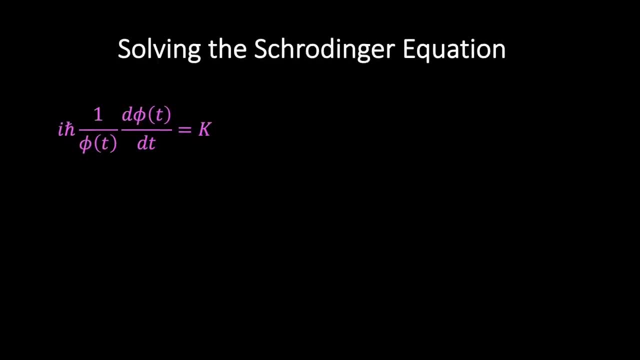 If we rearrange this expression, we find the following blue equation: This differential equation tells us that the function phi of t, which is its solution, has the property that its first derivative is proportional to the function itself. Now, anyone familiar with calculus 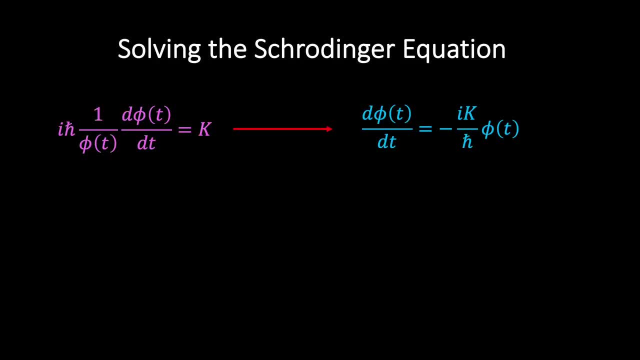 will recognise that the derivative of an exponential function gives another exponential function and therefore it follows that phi of t can be written as an exponential function. Therefore, let's assume that the solution to the differential equation has the following form: where alpha is a constant that will be determined shortly. 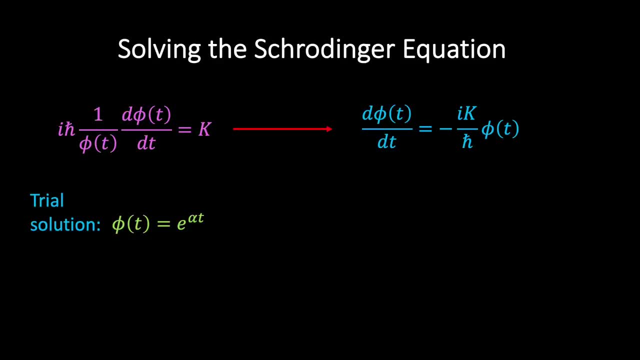 We can test whether this is indeed a solution by plugging it back into the equation, in which case we find the following expression: If we then cancel phi of t from both sides, we see that alpha equals minus i, k over h bar, and so if we sub this back into our trial solution, 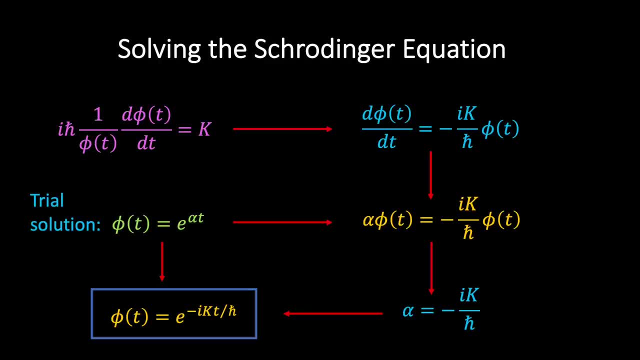 we find that phi of t is equal to e, to the minus i k t over h bar. Note that this substitution has caused the exponential to become complex, since it contains a factor of i in the exponential. Now, at this stage, it will prove illustrative. 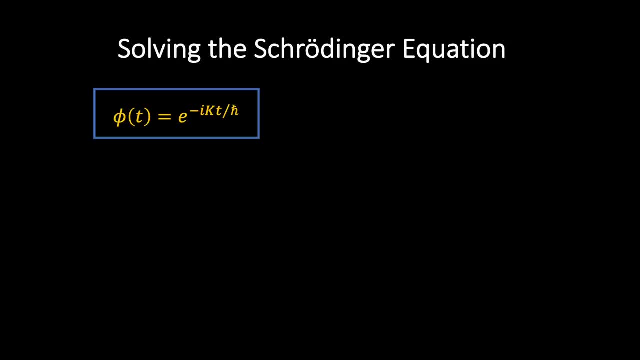 to rewrite this expression in an alternative but identical form by making use of Euler's famous equation, which links complex exponentials with trigonometric functions. Applying Euler's equation to our specific example, we find the following expression: and if we reintroduce the factors of 2, pi. 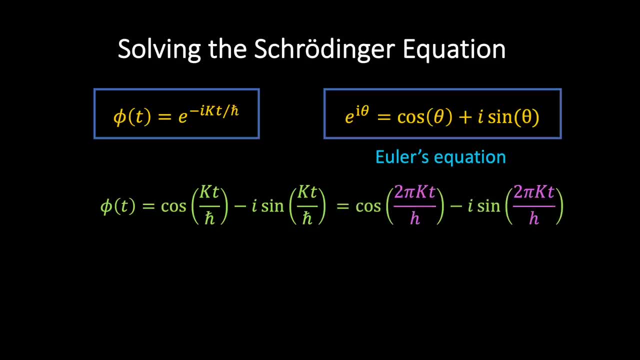 we find the following Now. the benefits of rewriting phi in this equation in this way is that we see explicitly that phi of t is an oscillatory function in time and we can read off the angular frequency immediately and we see that omega equals 2 pi k over h. 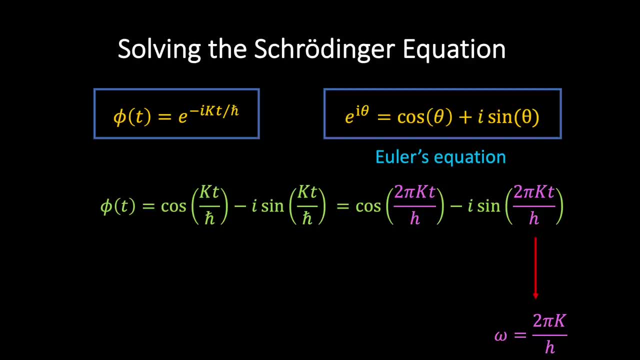 We also know that the angular frequency omega is related to the frequency of oscillation f, by the equation, omega equals 2 pi f, and therefore we see that the constant k is related to the frequency f, by the relation k equals h f. Now this might all seem a bit tedious. 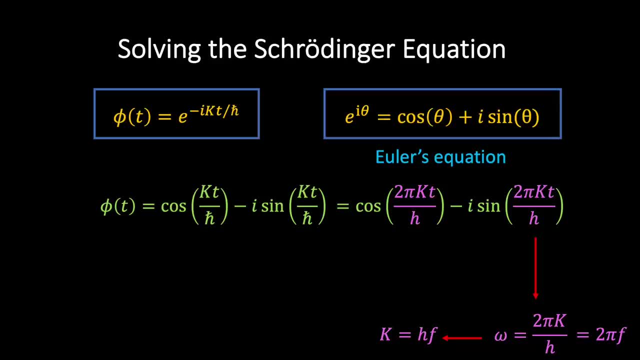 and pointless, until you remember that, according to the de Broglie-Einstein relation, the energy of a quantum particle is related to its frequency by the relationship e equals h, f, And so we see that the separation constant k must in fact be equal to the energy e. 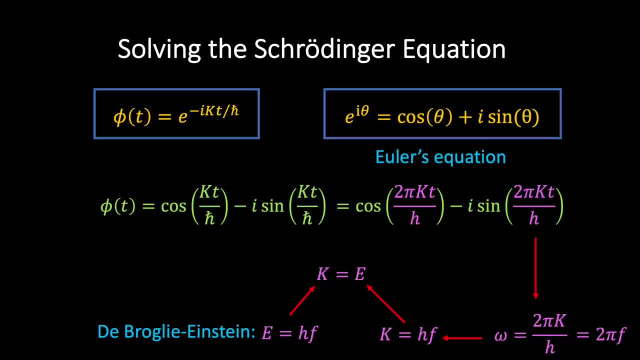 Now, I don't know about you, but I think that that's a very neat result, And so we can finally write that phi of t is equal to e, to the minus i times e times t divided by h bar. Okay, so now that we've figured out a solution, 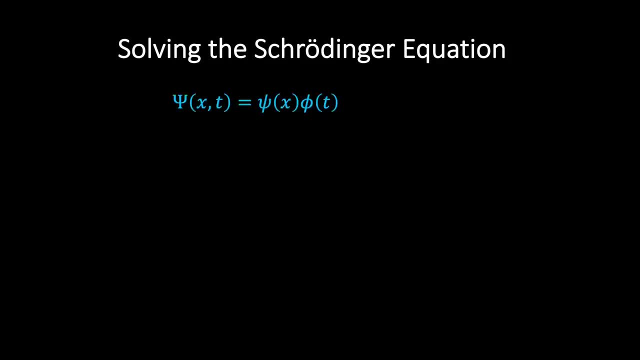 for the time-dependent part of the equation. let's sub this back into our general expression we started with. Our next task is to solve the space-dependent equation and find out what psi of x is. To begin with, let's sub in: k equals e. 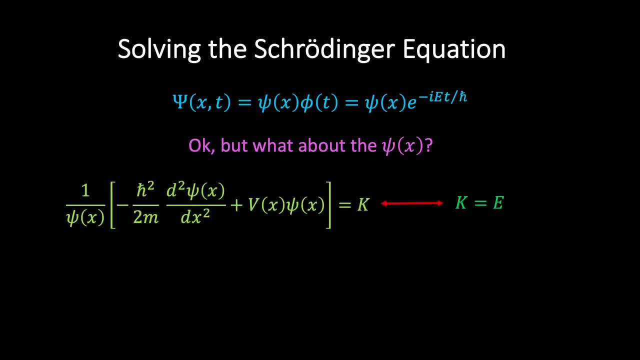 into the space equation we obtained earlier. Next, if we rearrange the term slightly, we find the following expression: This equation is referred to as the time-independent Schrodinger equation because the time variable t does not enter the equation. The solutions of this equation determine: 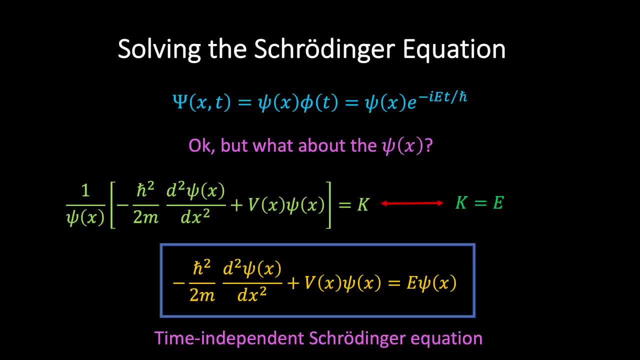 the spatial dependence of the general wave function and are referred to as eigenfunctions, which in German means characteristic function. Once the eigenfunctions are determined, we can then reintroduce the time dependence by multiplying by the time factor e to the minus i e t over h bar. 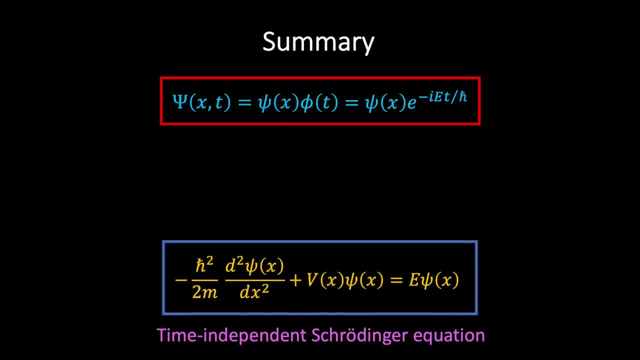 So, in summary, the separation of variables approach has led us to the conclusion that the eigenfunction psi of x, which specifies the space dependence of the wave function, is a solution to the time-independent Schrodinger equation. Furthermore, we have seen that the time dependence 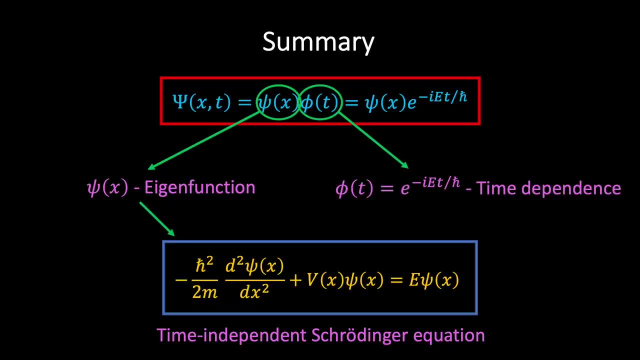 of the wave function is governed by the term phi of t equals e to the minus i e t over h bar, where e is the total energy of the particle in the system. Now that we've sketched the general equation and the general procedure, 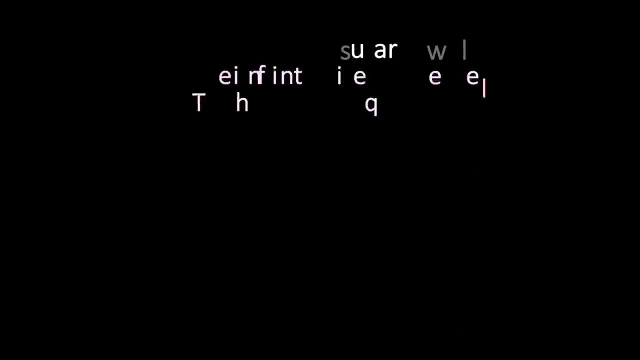 let's apply this approach to a specific example. To begin with, we're going to consider a situation in which a particle is confined to a one-dimensional box of width a, such that the particle is free to move around inside the box, but it's unable to escape. 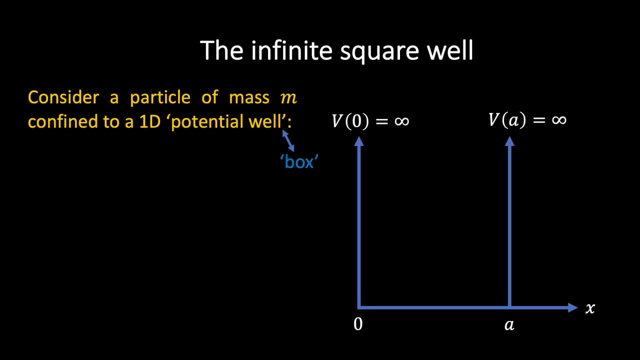 This example is often referred to as the infinite square. well Now, although this may seem like a slightly strange and contrived example, it's worth considering, since it serves as a wonderfully accessible test case for all the fancy quantum mechanical machinery that comes in a more advanced course in quantum mechanics. 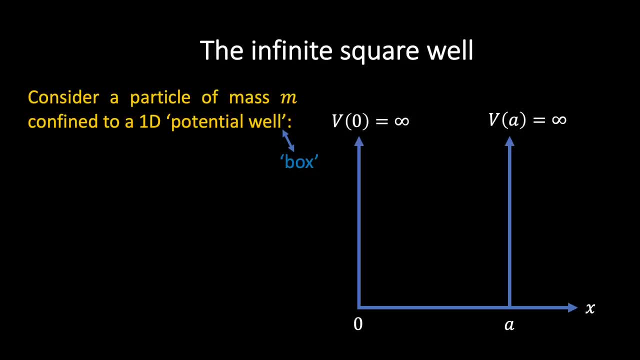 We can represent this situation by specifying the potential energy in the following manner. The first thing to notice is that outside the box, the wave function must equal zero, since the probability of finding the particle outside the box is zero. However, inside the box, where v of x equals zero, 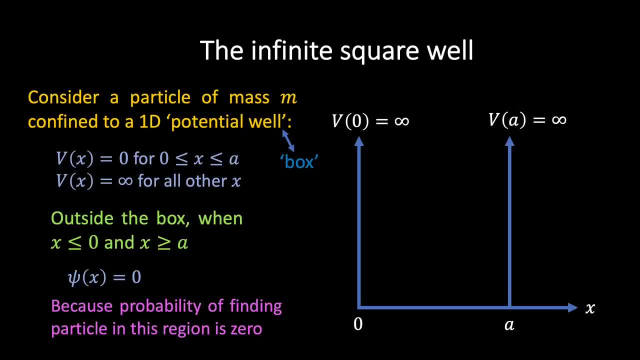 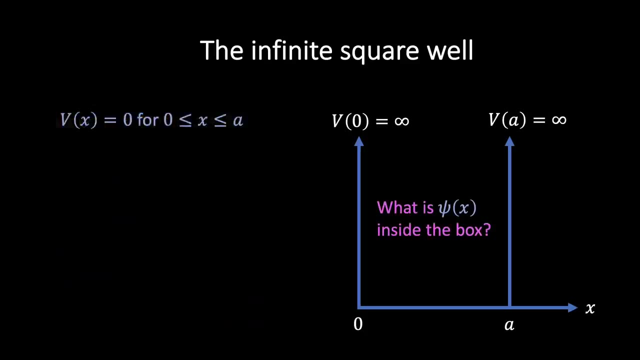 the particle is completely free to move, except at the two ends- x equals zero and x equals a, where an infinite force prevents the particle from escaping. So the natural question arises: what form does the wave function take inside the box? To answer this question, we simply need to solve: 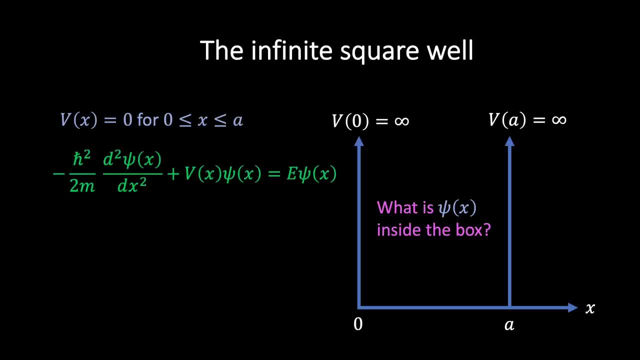 the time-independent Schrodinger equation inside the box. Since we know that the potential energy is zero inside the box, the time-independent Schrodinger equation simplifies to the following yellow equation: We can then rearrange this expression and write it suggestively in the following form: 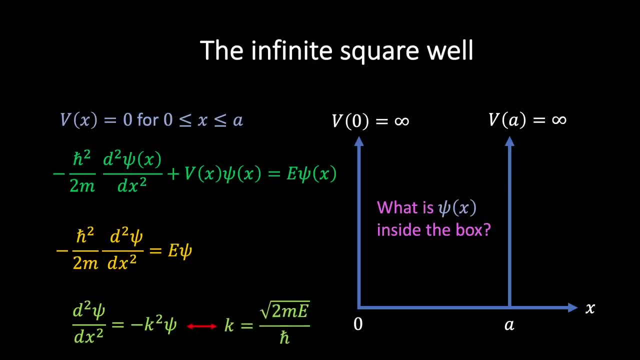 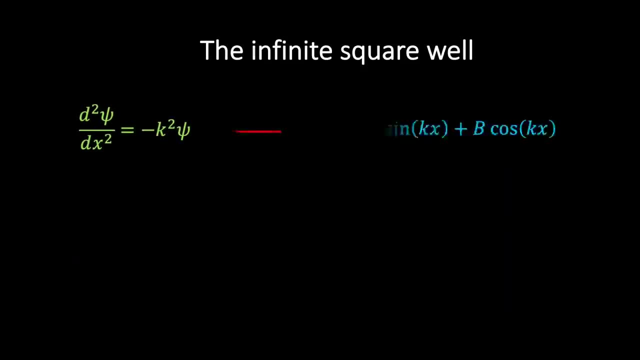 where we have defined k as the square root of 2m e over h bar. Now, the general solution to this equation takes the following form: where a and b are arbitrary constants, as can be verified by substituting the expression back into the equation. 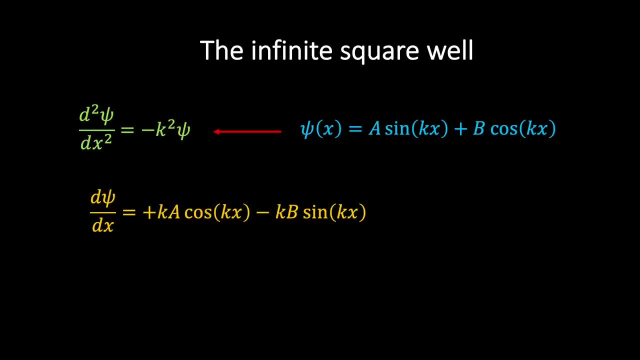 in which case we have that d psi by dx equals the following yellow expression: and if we differentiate again with respect to x, we find d2 psi by dx squared equals the following purple expression, which is simply equal to minus k squared psi, as required: 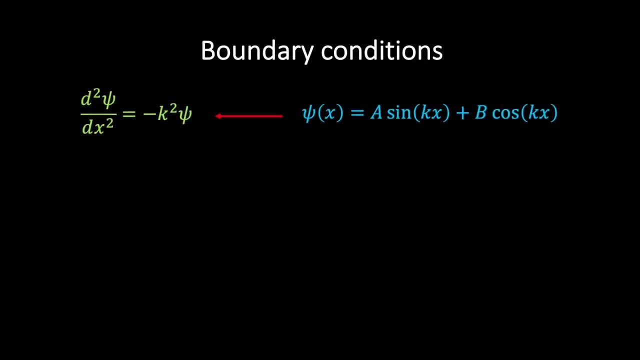 We can fix the constants a and b by considering the boundary conditions of the problem. In the case of the infinite square-well potential, we know that psi of x equals zero outside the box, and we also know that psi of x is not equal to zero inside the box. 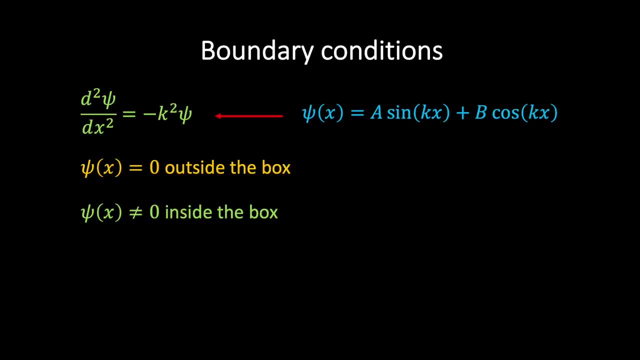 In order to meaningfully interpret the wavefunction as a probability density function, we require that the wavefunction is continuous. In other words, we require that the function changes smoothly from where it's zero to where it's non-zero. Therefore, continuity of the wavefunction at the edges of the box. 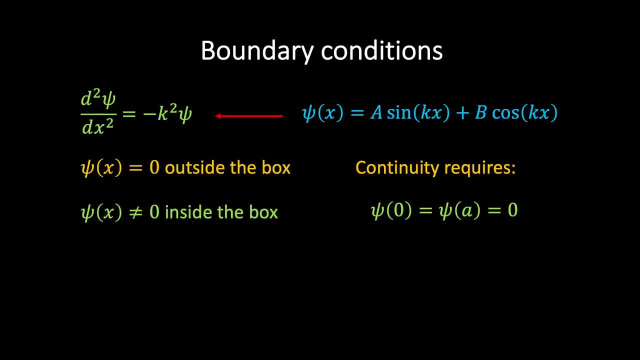 requires that psi of zero equals psi of a equals zero. So what does this tell us about a and b? Firstly, when x equals zero, we find that a sine zero plus b cos zero equals b, and therefore b must be equal to zero. 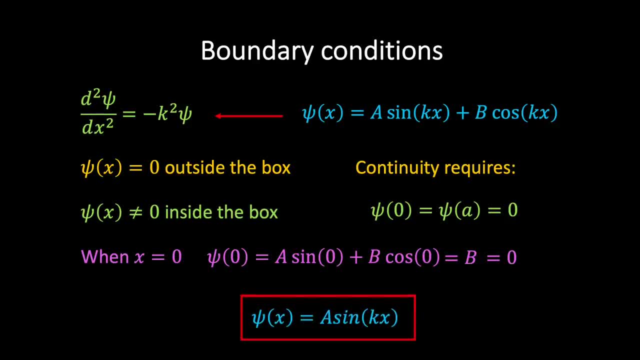 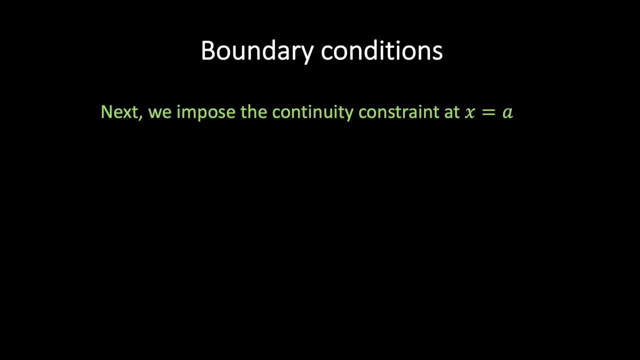 And so, finally, we can write: psi of x equals a sine kx. Next, we impose the continuity constraint at x equals a, and therefore we have that psi of a equals a sine ka, and this must be equal to zero. And so we see that either a equals zero, 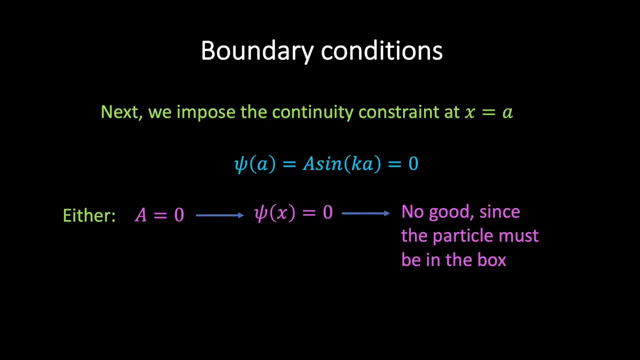 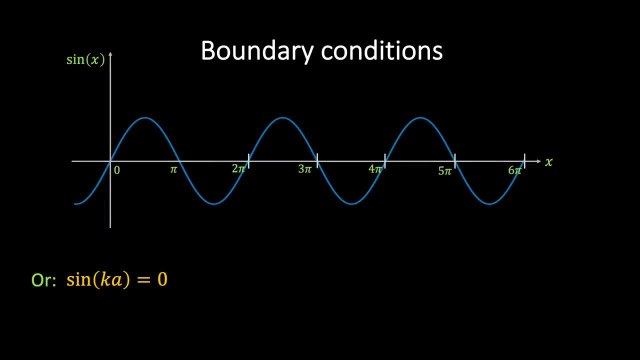 in which case we are left with the trivial solution: psi of x equals zero, or else we have that sine of ka equals zero. Now we know that the sine function is equal to zero whenever the argument of the function is equal to an integer multiple of pi radians. 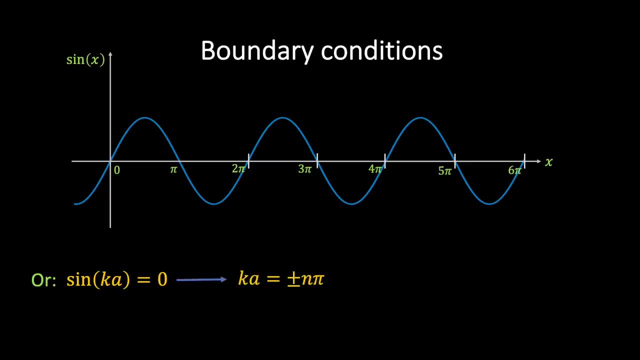 In other words, we can write: ka equals plus or minus n times pi, in which case we can define: k equals n pi over a for integer values of n. Note: we do not need to include the negative values of k, since sine of minus x equals minus sine of x. 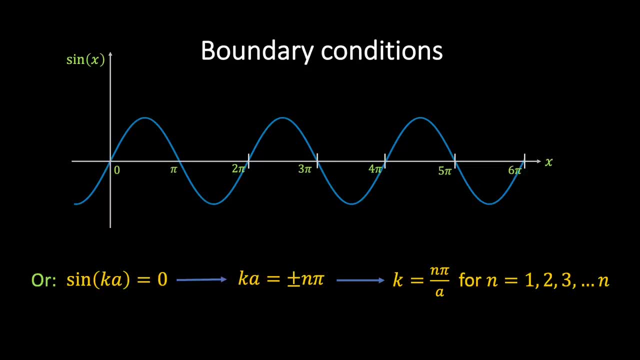 and we can simply absorb the minus sign into the constant a. Also, note that we should not have included n equals zero, because that would again imply that psi of x equals zero for all values of x. So, armed with this boundary constraint on k, 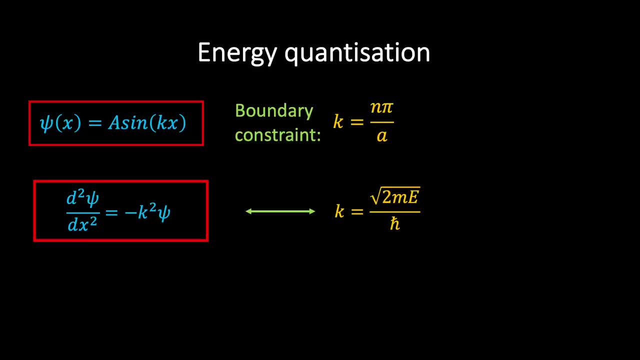 we can then combine this with the fact that k equals the square root of 2me over h bar. to write n pi over a equals the square root of 2me over h bar, And if we rearrange this for the energy e, we find the following expression: 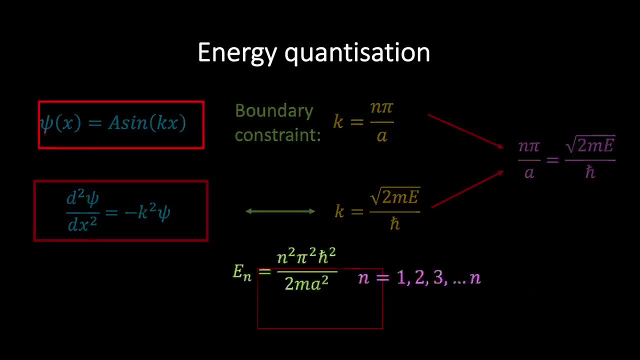 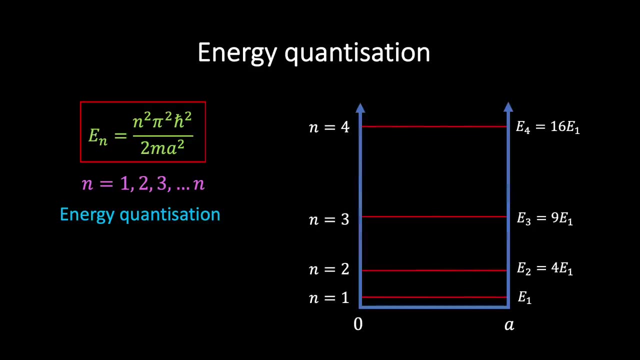 So what exactly is this telling us? Well, the first thing that we notice is that the particle energy has become quantized and can only take certain discrete values depending on the value of n, with each different value of n corresponding to a different energy. 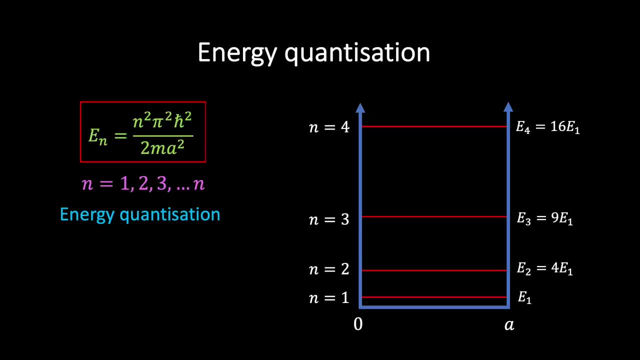 And in turn this corresponds to a different eigenvalue. We also notice that the lowest possible energy state is not zero, as would be the case in classical physics. Rather, the ground state energy is given by the following expression: This is a general feature of quantum mechanical systems. 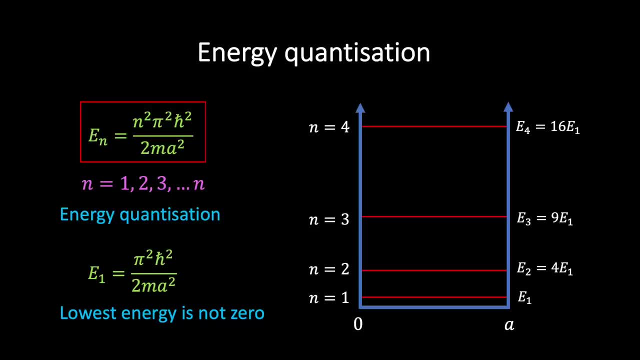 and can be understood in terms of Heisenberg's uncertainty principle which, roughly speaking, says that whenever you confine a particle to a region of space, there is an inherent uncertainty in the particle's momentum and therefore its energy. It is this quantum uncertainty 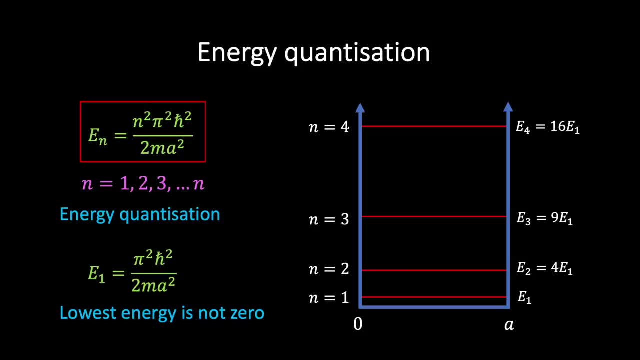 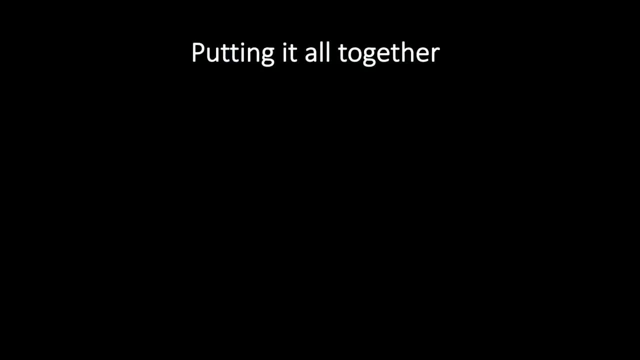 that gives rise to the non-zero ground state energy when a particle is confined to a region of space. We are now in a position to combine all of the results that we've derived so far and bring everything together. If you recall, we derived an expression for the eigenfunction psi of x. 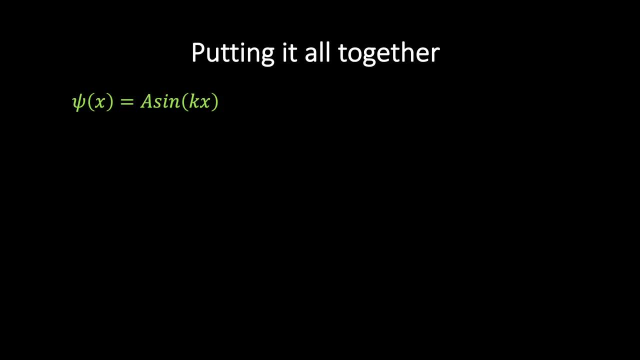 when we solved the time-independent Schrodinger equation. If we now sub in the boundary condition constraint equation into our eigenfunction expression, we find that the nth eigenfunction is given by the following expression: If we sketch the first few eigenfunctions, we see that they look exactly the same. 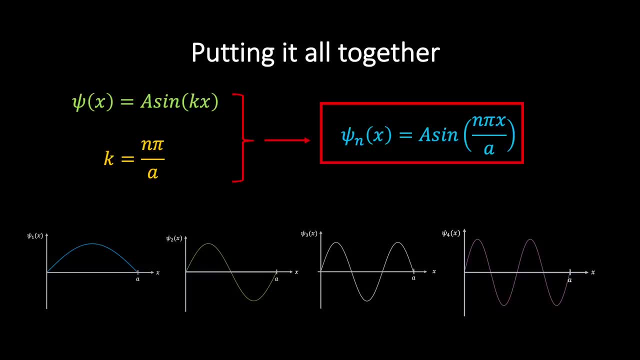 as the standing waves in a string of length. a. The lowest energy state corresponding to psi 1 of x is referred to as the ground state, and those states whose energy increase in proportion to n squared are called excited states. Once we have specified the eigenfunctions, 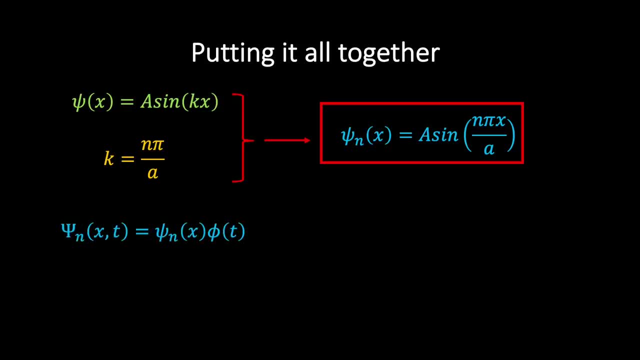 we can construct the full wavefunction solution of the time-dependent Schrodinger equation for any value of n, and, as we've already seen, we can write this in the following form where the time dependence is now manifest. And so for our particular particle-in-a-box example, 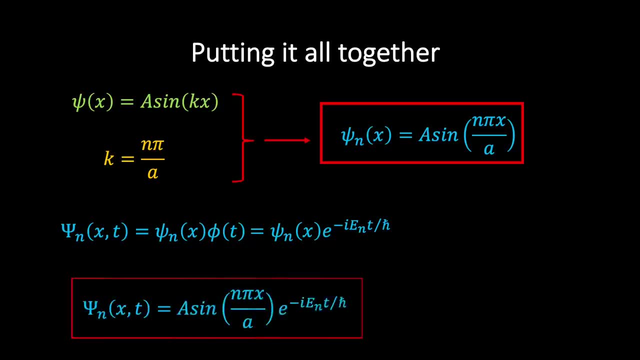 we find that the wavefunction of our particle is given by the following blue expression, where here en refers to the energy of the nth eigenstate. We see that we've managed to determine an expression for the wavefunction up to an overall constant, a. 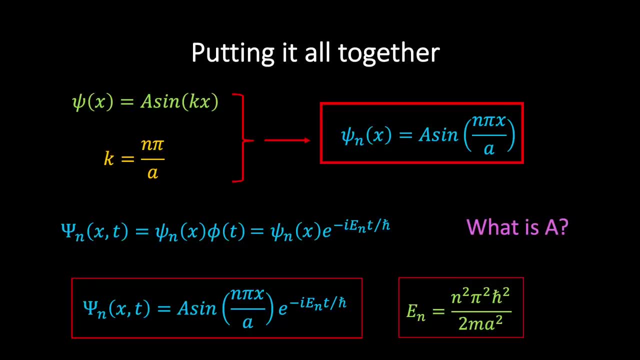 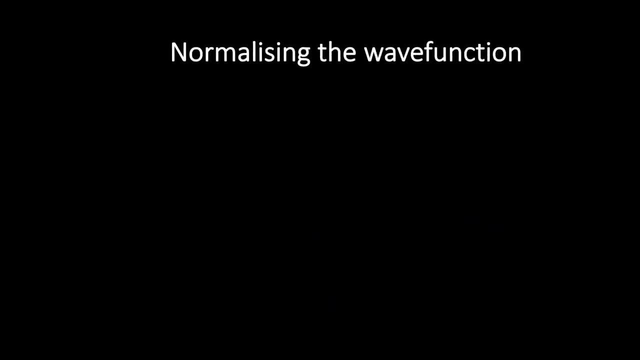 But that leaves an obvious question: What value does a take, and can we determine this? Well, thankfully, the answer is yes, and to do this we simply use Born's probability rule which, if you recall, says that the probability of finding a particle in a region, 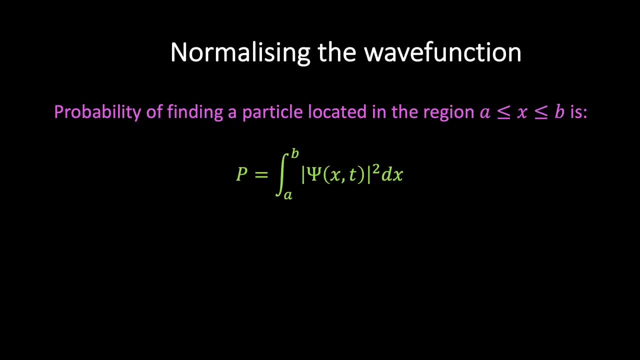 is given by the integral, with respect to x, of the modulus squared of the wavefunction. Now, in the example of a particle confined to the box, we would expect the probability of finding the particle inside the box to be exactly equal to 1,. 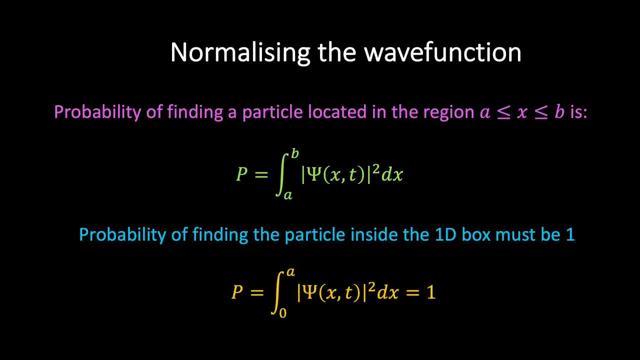 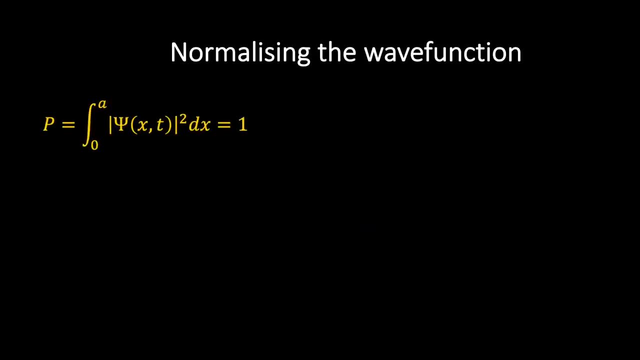 and therefore we can write the following green expression for the probability. Our task is to now evaluate this integral. To do so, we recall that the modulus squared of the wavefunction involves multiplying the original wavefunction by its complex conjugate, and if we do this, we find the following result: 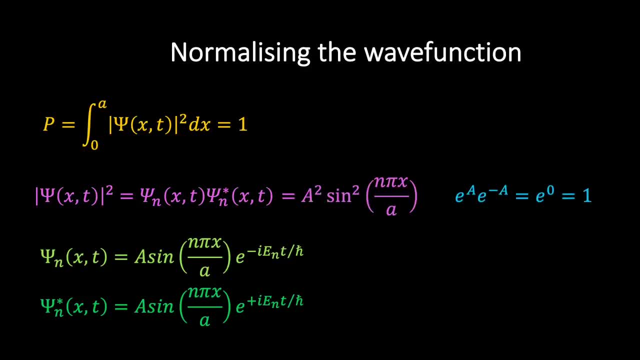 where we have used the rule of exponents to simplify our expression, and so we see that our requirement that the probability of finding the particle in the box must be equal to 1 simplifies to the following constraint In order to evaluate this integral: 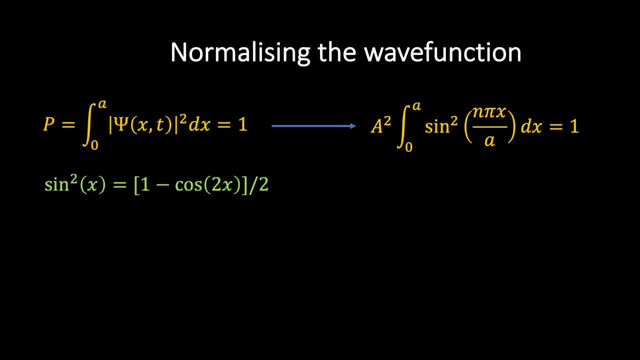 we use the trigonometric identity sine: squared of x equals 1 minus cos of 2x all divided by 2, and this allows us to rewrite the integrand in terms of cosine as follows. If we then write this as two separate terms: 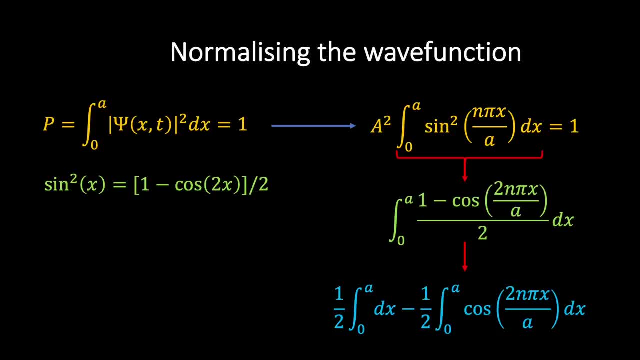 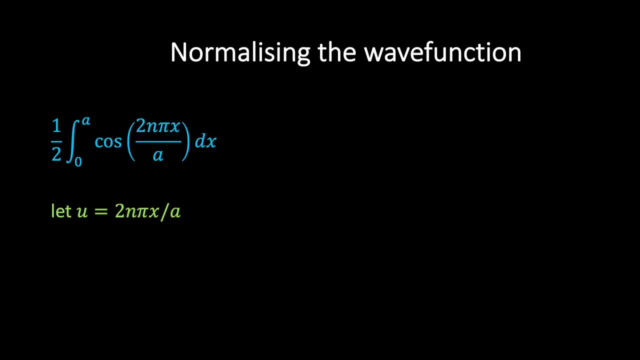 we find the following blue expression: The first term can be integrated immediately, in which case we find the following simple result: But what about the second term? For this slightly trickier term, we let u equal 2n, pi x over a. 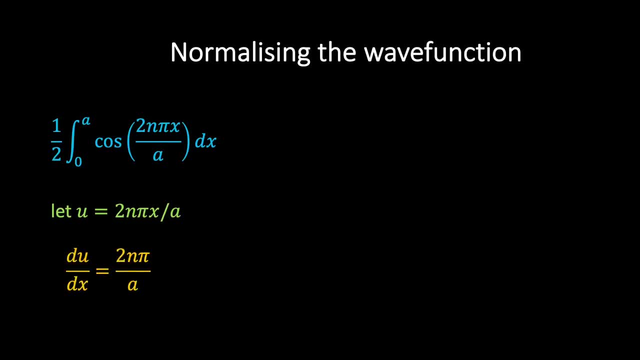 in which case du by dx equals 2n pi over a, and so we can write: du equals 2n pi over a times dx. It then follows that we can rewrite our integral in the following form: in terms of u, And if we evaluate this, 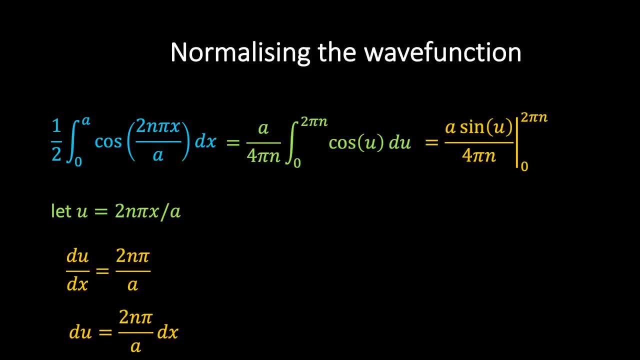 we find the following yellow expression: When we insert the limits, we see that we get two terms. and the second term is 0 for all values of n, since sine of 0 equals 0. And so we are left with just the first term. 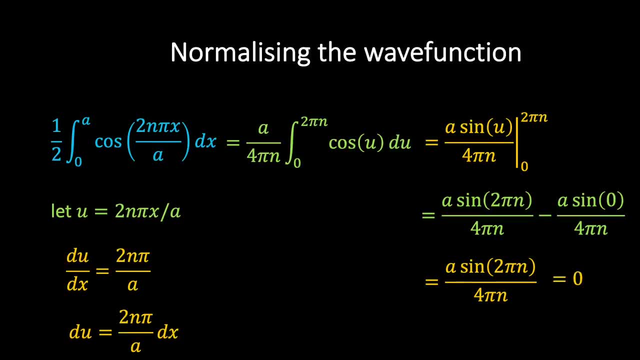 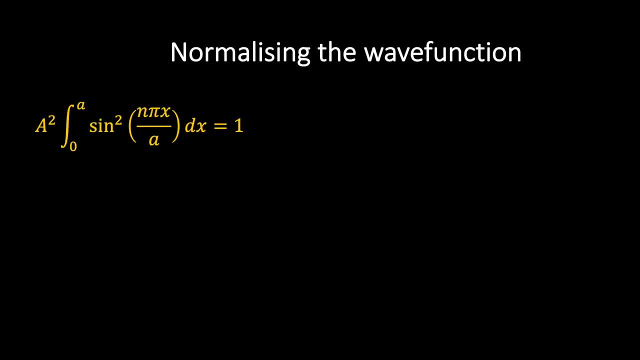 which is also equal to 0 for all integer values of n. And so, if we go back to our original expression, we see that after the duster sequence, we have the following constraint: And therefore a equals the square root of 2 over little a. 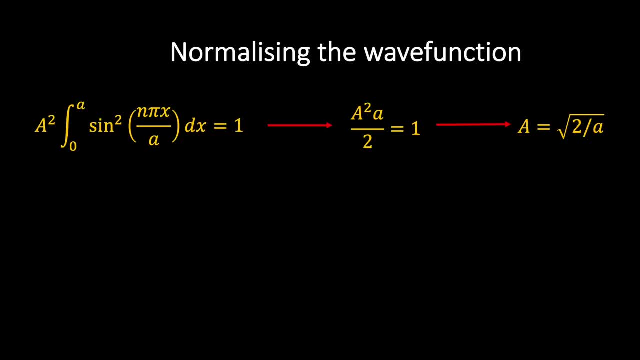 And therefore inside the box. the wavefunction for the nth quantum state is given by the following expression, And this is our final answer: The process that we've just gone through of determining the wavefunction coefficient to ensure that the total probability of finding the particle somewhere in space is 1. 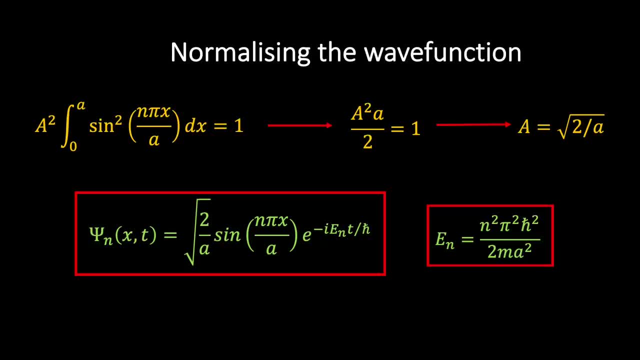 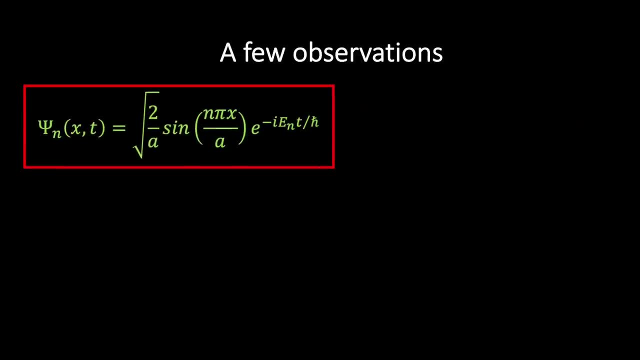 is referred to as normalising the wavefunction. Now, there are a couple of key points that are worth mentioning at this stage. Firstly, a wavefunction of this form describes what is known as a stationary state, because the modulus squared of the wavefunction 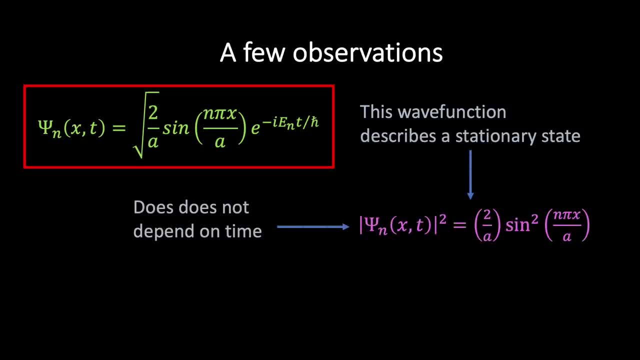 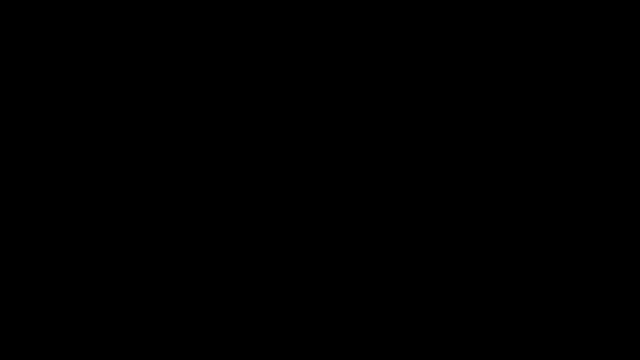 does not depend on time, which means that the probability does not change with time. We also note that such a stationary state has a sharply defined energy corresponding to each value of n, and we'll have more to say about this point later. If we plot the modulus squared, 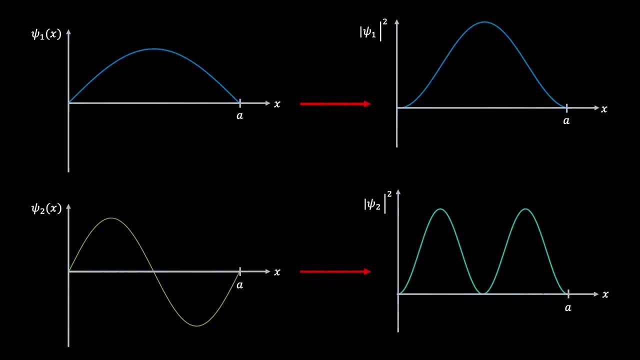 of the wavefunction for each value of n. then we can visualise where we are most likely to find the particle within the box for each different eigenstate. For example, we see that in the ground state our particle in a box is most likely. 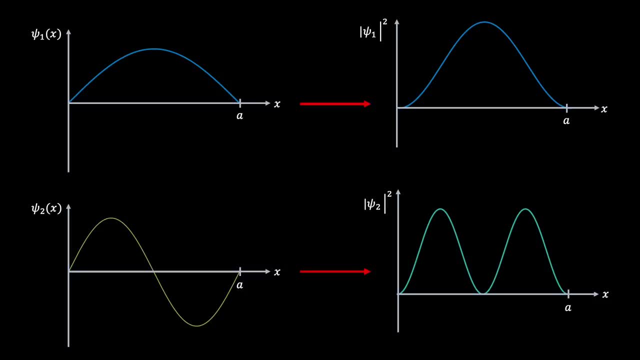 to be found in the middle of the box, since this is where the modulus squared of the wavefunction peaks and therefore this is where the probability of finding the particle peaks. Whereas in the n equals 2 state, we see that there is actually now 0 probability. 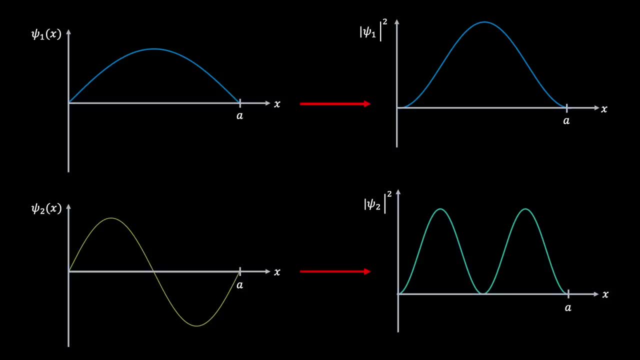 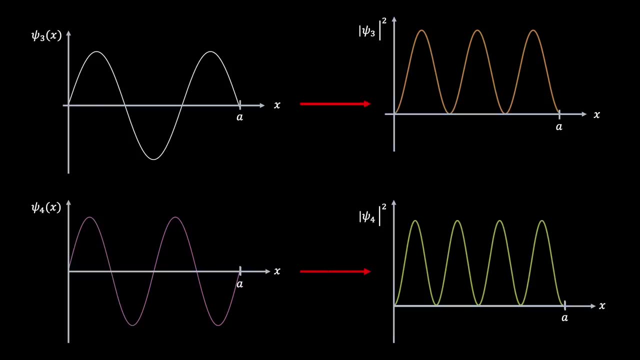 to find the particle in the middle of the box. We see that as n increases, the quantum mechanical probability, density oscillates more and more and in the limit that n approaches infinity, the oscillations are so compressed that no experiment could possibly have the resolution to observe the oscillations. 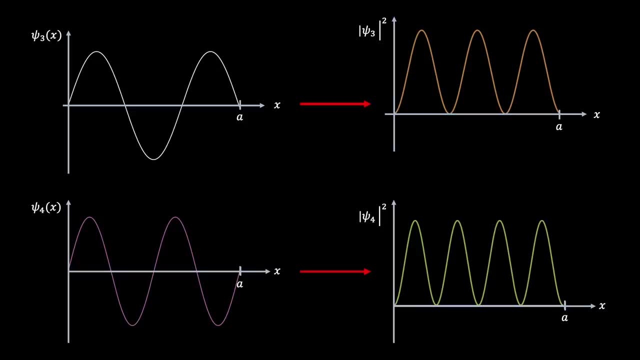 and in this limit the particle will have equal probability of being found at any location within the box. Furthermore, the fractional separation of the eigenvalues approaches 0 as n approaches infinity. so in that limit the discreteness of energy cannot be resolved. 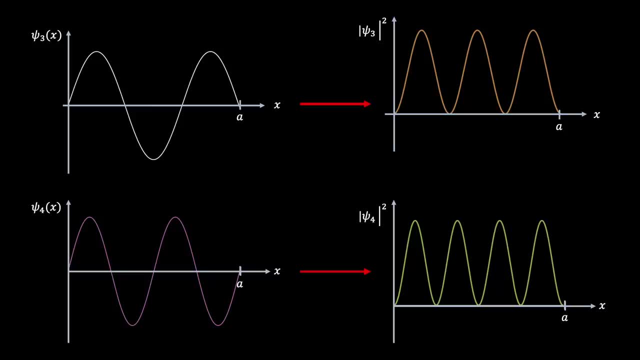 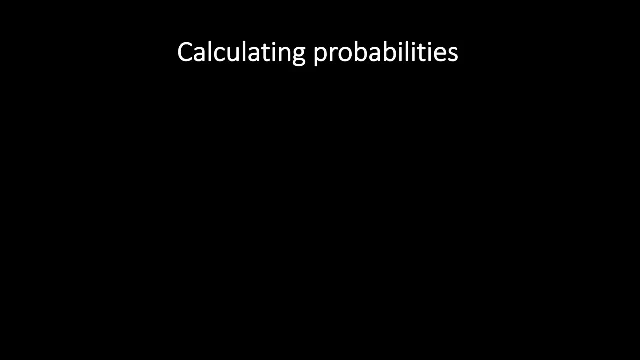 and it appears as if the energy of the particle varies continuously. And so we see that the quantum mechanical predictions approach the predictions of classical mechanics in the limit of large quantum number or high energy. Now, once we've fully normalised the wavefunction, 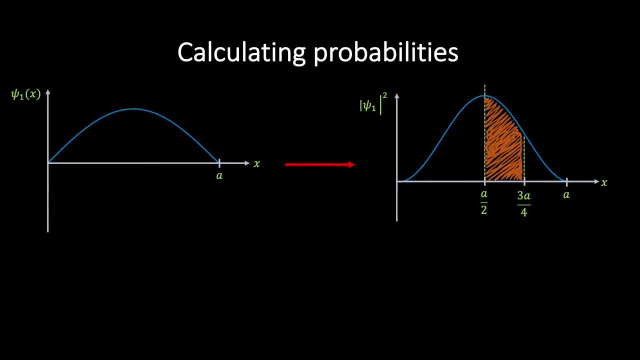 we can calculate the probability of finding a particle in a given energy state in a particular region of space. To do this, we simply need to integrate the modulus squared of the corresponding wavefunction over the region of space that we're interested in, For example, suppose I wanted to calculate 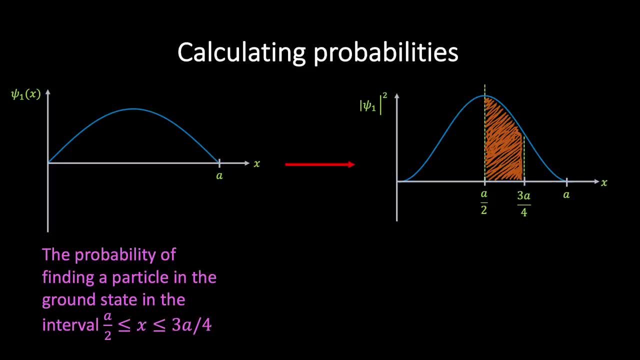 the probability of finding a particle in the ground state in the following interval. In this case, I would simply need to calculate the integral of the modulus squared of the normalised wavefunction between a over 2 and 3a over 4.. In order to evaluate this integral, 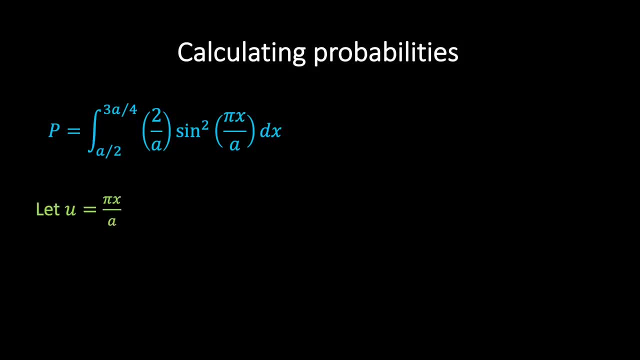 we will change variables and let u equal pi x over a, in which case we have that du equals pi over a dx. If we then sub this back into our integral expression, we find the following result: Next, we use our favourite trigonometric identity. 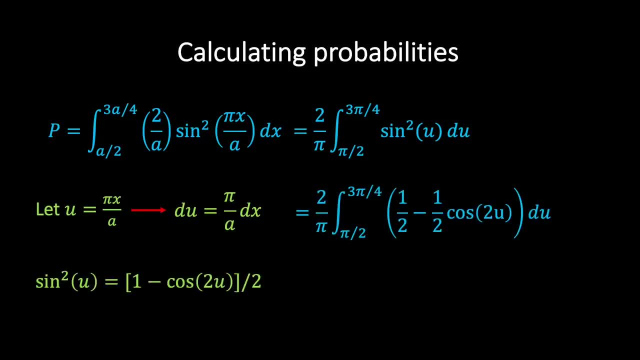 to re-express our integral. If we then carry out the integral and sub it in the limits, we find an answer of a quarter plus 1 over 2 pi, which is roughly equal to 0.41.. And so we see that the probability of finding 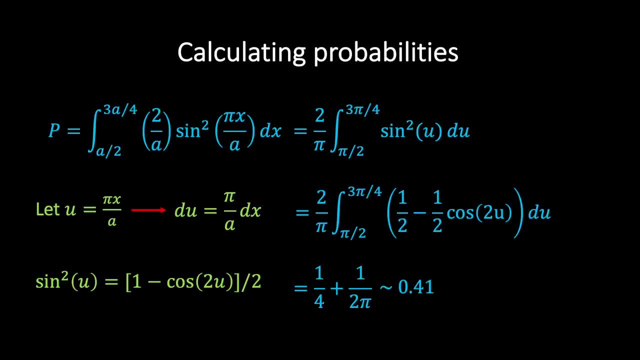 our particle within this region of the box has been successfully determined by calculating the integral of the modulus squared of the normalised wavefunction. And so we see that once we've normalised the wavefunction, we can calculate the probability of finding a particle in any particular region of space. 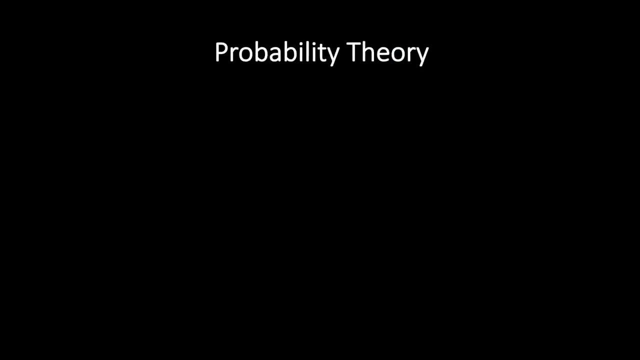 OK, but what else can we do? Well, as we've already seen, according to Born's probabilistic interpretation of the wavefunction, the outcome of a measurement in quantum mechanics is a random variable with many possible values. Because statistics plays such a fundamental role? 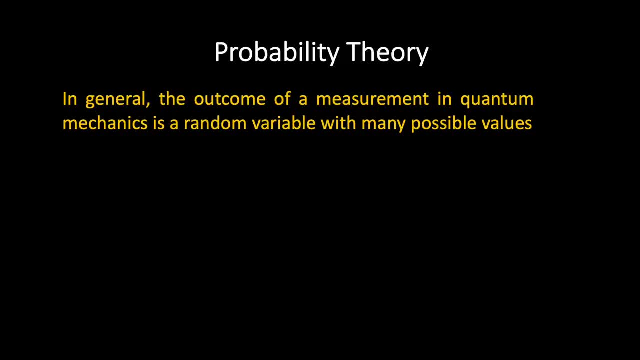 in quantum mechanics, it's worth briefly digressing to introduce some probability theory and notation, And I will do so in the context of a simple example. Imagine a group of 12 people whose ages are as follows: If we let n of x represent the number of people, 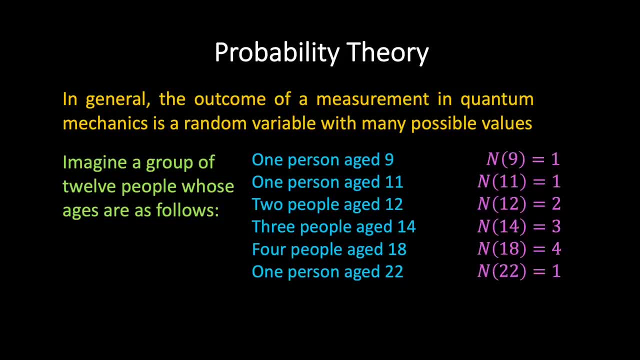 of age x, then we can write the following list of information: The total number of people in the room is then given by the sum of these terms. Now, if you were to select one individual at random from this group, then the probability that this person's age would be. 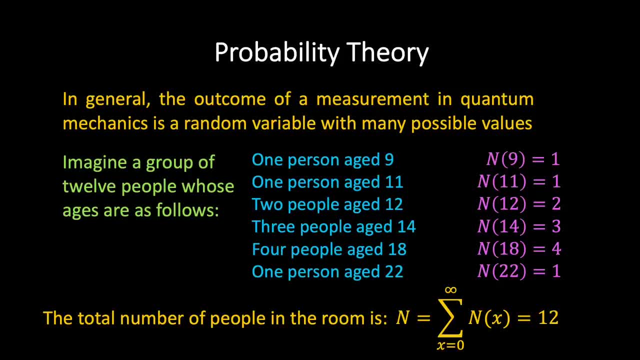 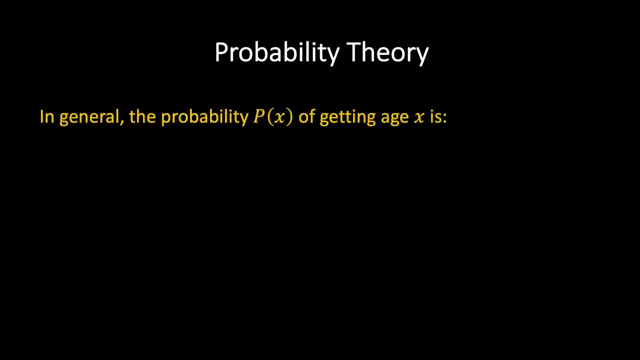 for example 9, would obviously be 1 in 12, because there are 12 possible choices, all equally likely, of whom only one individual has that particular age. It follows that if p of x is the probability of getting age x, 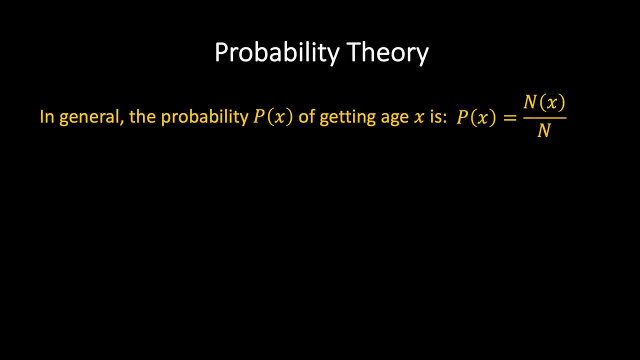 then in general we can write: p of x equals n of x divided by n. For example, the probability of selecting a person whose age is 12 would be: p of 12 equals 2 over 12, which is equal to 1. sixth. 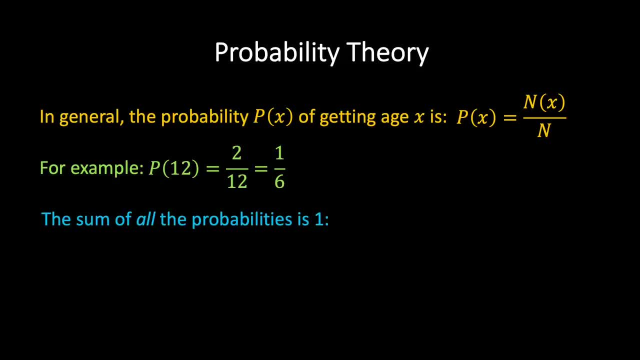 It should hopefully be obvious that the sum of all the probabilities must be equal to 1, since the person you select must have some age, And so we can write the sum of p of x from x equals to 0 to infinity is equal to 1.. 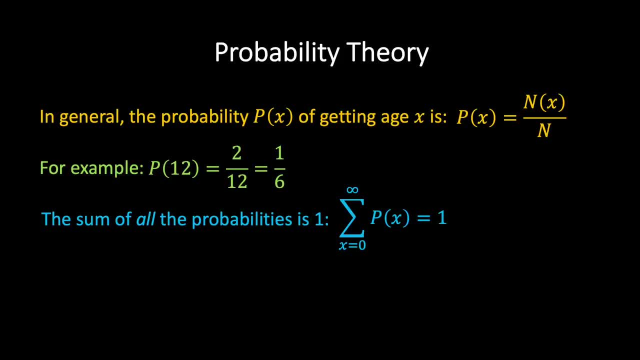 Now, if we wanted to calculate the mean or average age, we would simply add together all the ages and divide by the total number of people, and we can write this in the following way, which, if we evaluate, returns the number 15.. 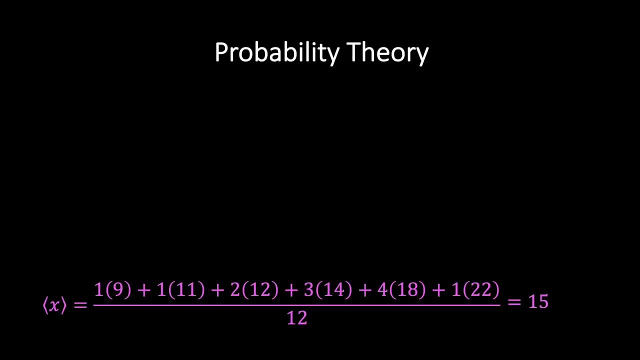 It follows that, in general, the average value of x is then given by the following expression: Notice that there need not be anyone with the average age In our example. no one happens to be 15 years old Now in quantum mechanics, 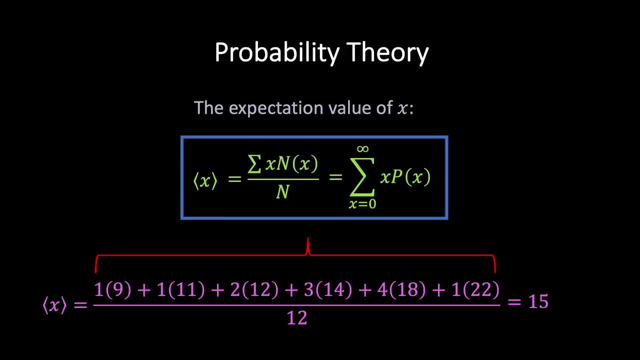 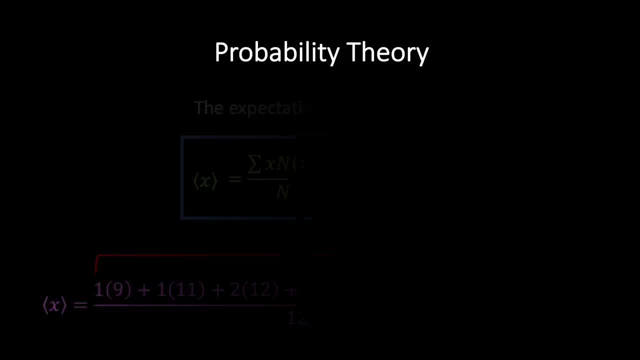 the average is usually the quantity of interest and in this context is referred to as the expectation value, and we'll have more to say about this later Now. in general, the expectation value of some function of x is given by the following expression: 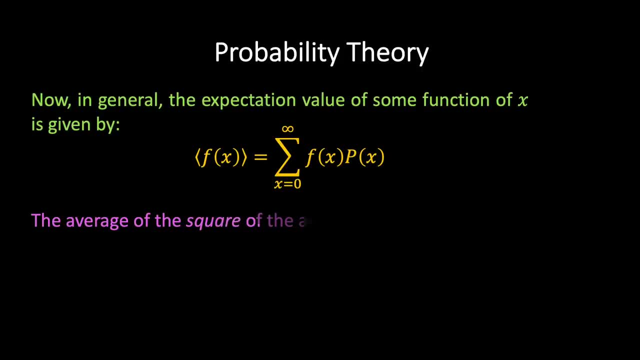 So, for example, if we wanted to calculate the average of the square of the ages in the group, then we would write this in the following form: Now, it's perfectly possible that two sets of data may have the same mean value, but in one set. 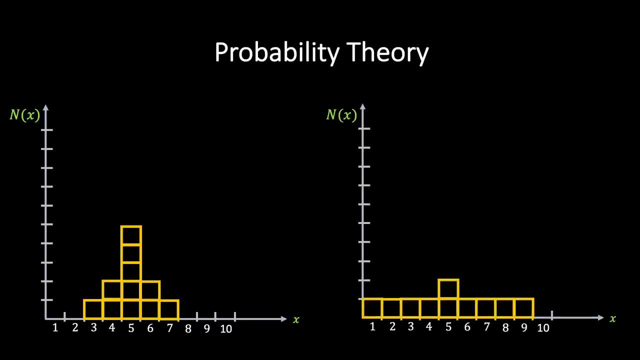 the data could be clustered around the mean value, and in the other set the data may be more spread out. Consider the following two histograms: The first is sharply peaked around the average value, whereas the second is broad and flat. Now it would be useful, therefore. 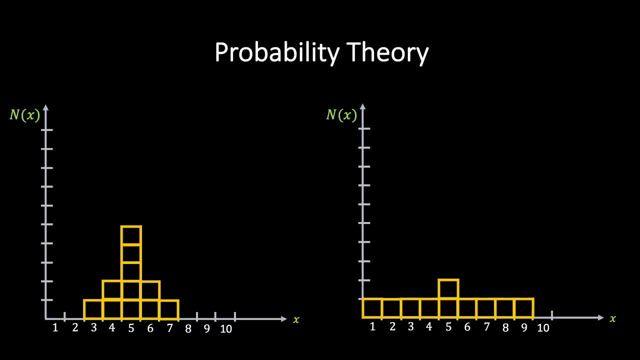 to have a numerical measure of the amount of spread in a distribution with respect to the average. Now it might seem like an obvious way of doing this would be to see how far each individual is from the average, In other words, calculate delta. x equals x minus. 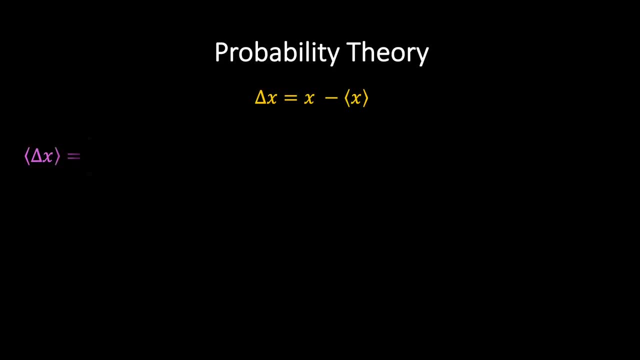 the expectation value of x and then compute the average or expectation value of the difference. However, if we do this, then we see that the expectation value is equal to zero. Now the conventional way to get around this problem is to square delta x before averaging. 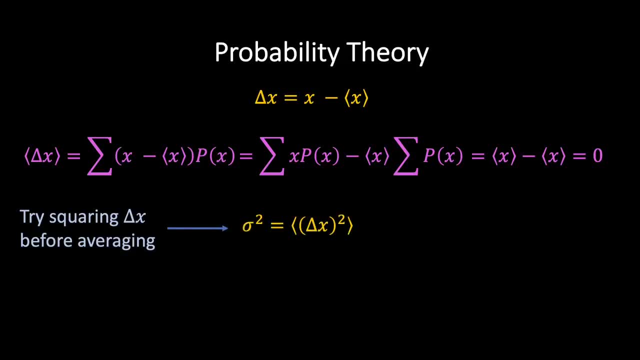 in which case we have the following expression: Here: the quantity sigma squared is referred to as the variance of the distribution, and sigma itself is called the standard deviation, which is the customary measure of the spread of the distribution around the average value. Now, before we move back onto quantum mechanics, 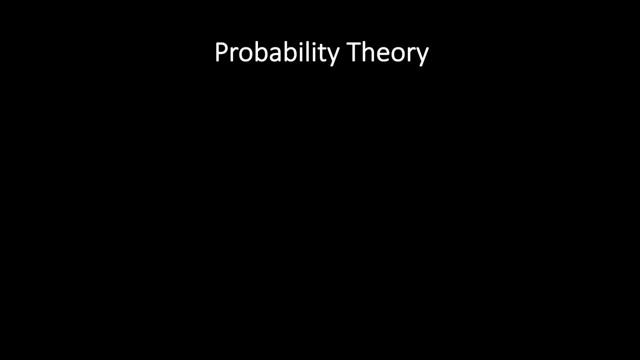 there is a useful theorem on variances which we'll need later. so let's take a moment to digress. If we take the expression for the variance and write it explicitly in terms of delta x and then expand out the bracket, we see that we can rewrite each term. 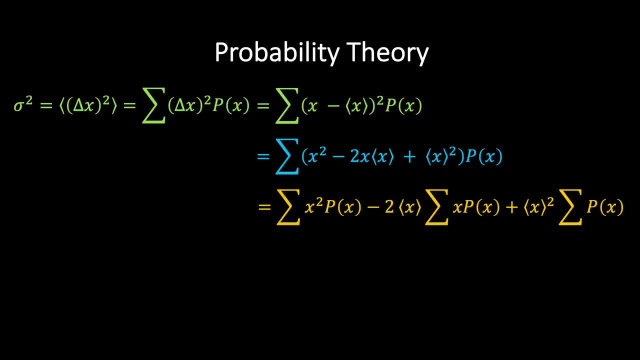 explicitly in terms of the probability p of x. and then we see that everything simplifies and we find that the variance can be written as the difference between the average of the square of x and the square of the average of x. Then, if we take the square root, 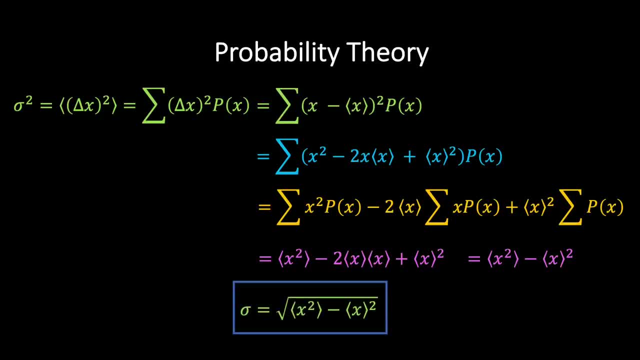 we obtain an expression for the standard deviation itself And we note that since sigma squared is clearly non-negative from its definition, then this result implies that the expectation value of the square of x is greater than or equal to the expectation value of x all squared. 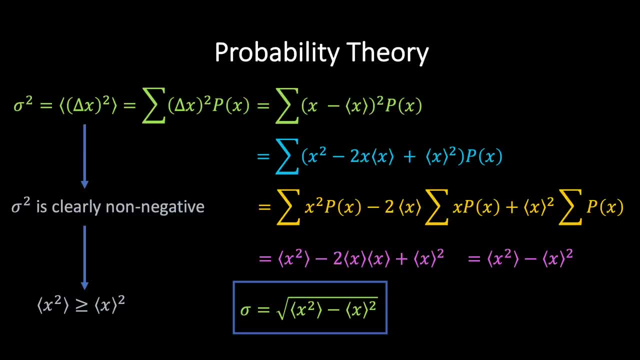 and the two are equal only when sigma equals zero and the distributions have no spread at all. It's worth noting that the standard deviation in the variable x is often referred to as the uncertainty in x, and we will return to the importance of this concept. 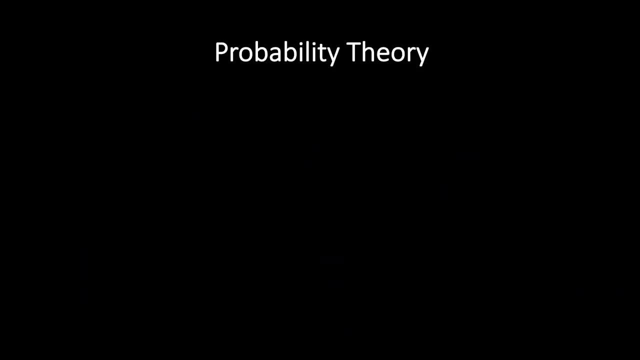 later in the video. It's worth noting that in our example, we specified the age of each individual as an integer and this therefore represented a discrete variable, But it's simple enough to generalise this analysis to continuous distributions When applying this to our example of age. 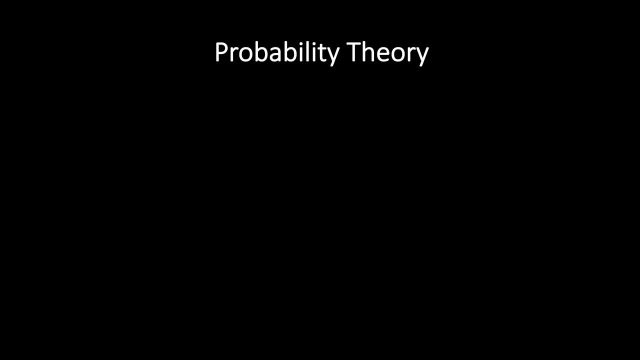 the sensible thing would be to specify the probability that an individual's age lies within some interval, say, for example, the probability that their age lies between 16 and 17.. It follows that the probability that some individual chosen at random has an age that lies between x and x plus dx. 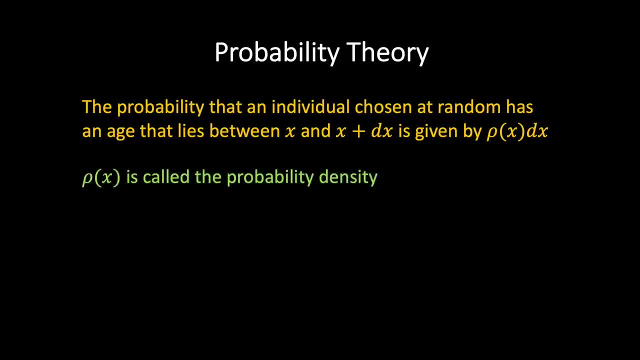 is given by rho of x- dx, where rho of x is called the probability density. It follows that, in general, the probability that some variable x lies between a and b is given by the integral of the probability density and the rules that we obtained for discrete variables. 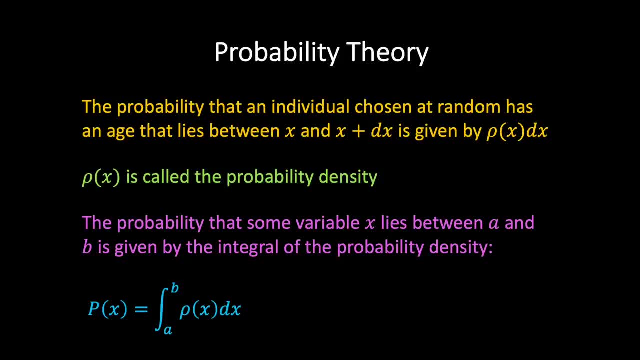 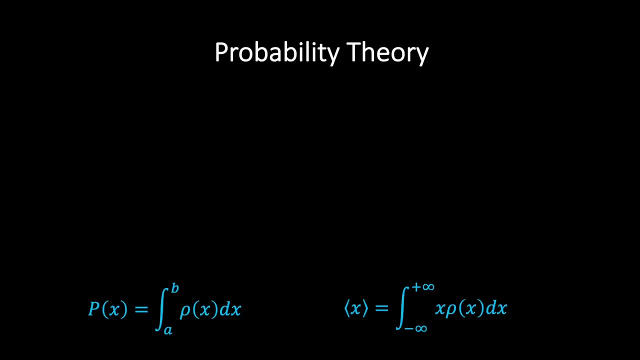 carry over in an obvious way. For example, the expectation value of a continuous variable is given by the following expression: Now we can see immediately how these results in probability theory translate into quantum mechanics. We've already seen that in quantum mechanics the probability of finding a particle in a region of space 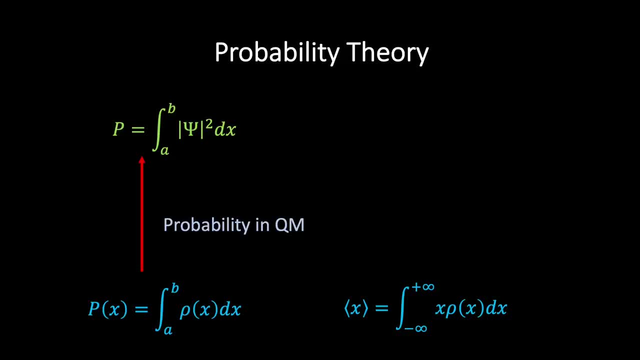 is equal to the integral of the modulus squared of the wave function, and so we see that the modulus squared of the wave function can be interpreted as the probability density function, which is how it's often referred to, Likewise the expectation value of a particle's position in quantum mechanics. 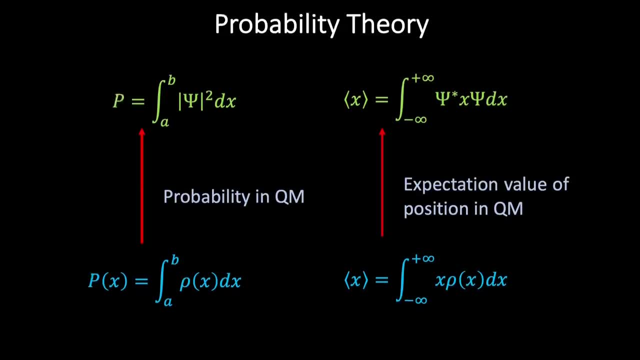 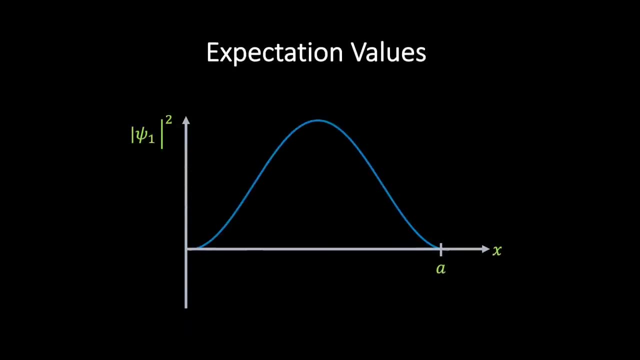 is given by the following integral. Let's now consider how this discussion of probability theory applies to the quantum mechanical example of the position of a particle in the ground state of the infinite square world potential. In principle, the expectation value of the position of the particle. 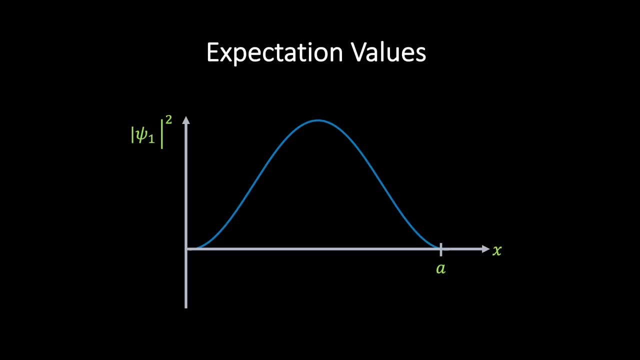 can be found by taking the average result of measurements on an infinite ensemble of identically prepared systems. Alternatively, as we've just seen, we can calculate the expectation value using the probability density function, which is simply the modulus squared of the wave function. 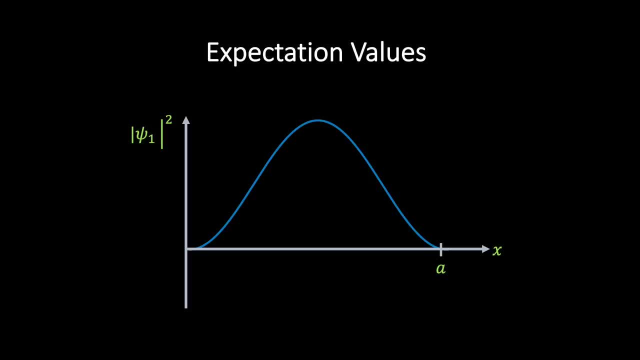 If we look at the plot of the modulus squared as a function of position, it certainly suggests that the most likely location to find the particle is in the centre of the box. But let's check this explicitly with a calculation using our newly developed probability theory. 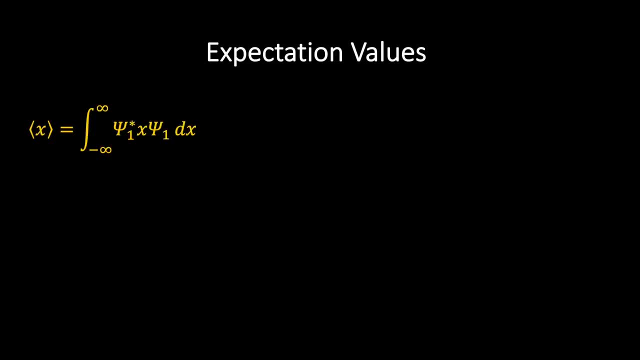 To begin with, we write an expression for the expectation value of position in terms of the ground state wave function. If we then write this in terms of the energy eigenstates, we see that the time dependence drops out and we're left with the following purple expression: 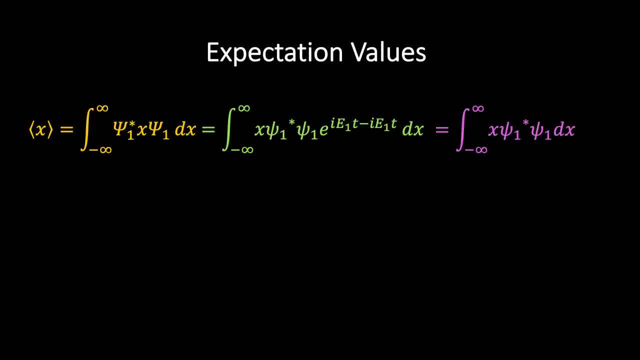 This is telling us that the expectation value of the position does not depend on time, but is a constant value. If you recall from our earlier analysis, the ground state eigenfunction is given by the following yellow expression And if we sub this into our expectation value equation: 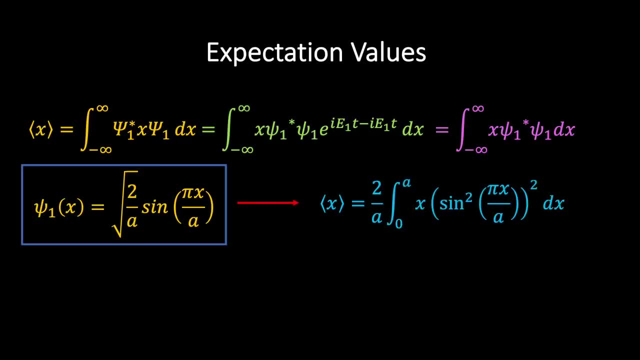 we find the following blue equation: If we then make use of the same trigonometric identity that we used earlier, we can get rid of the sine squared term. and we find the following yellow expression: Next, we will evaluate each integral in turn. 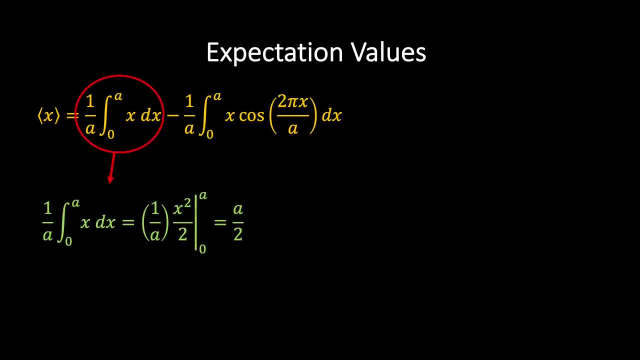 The first integral is simple enough and we find that it evaluates to a over 2.. The second integral is a little bit trickier and involves integrating by parts. Now, if we set f equal to x, then we immediately see that df equals dx. 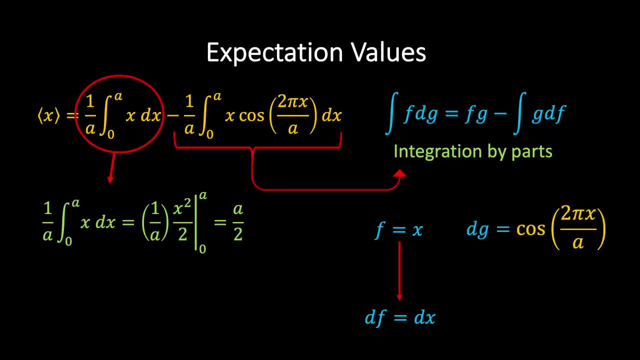 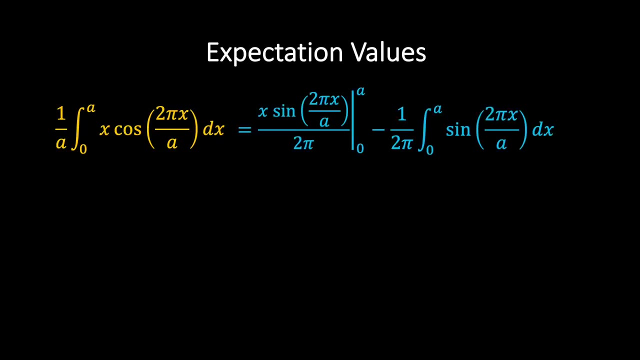 And if we identify dg with cos 2 pi x over a and integrate, we find that g equals a sine 2 pi x over a all divided by 2 pi. If we then plug these results back into our integral, we find the following blue expression: 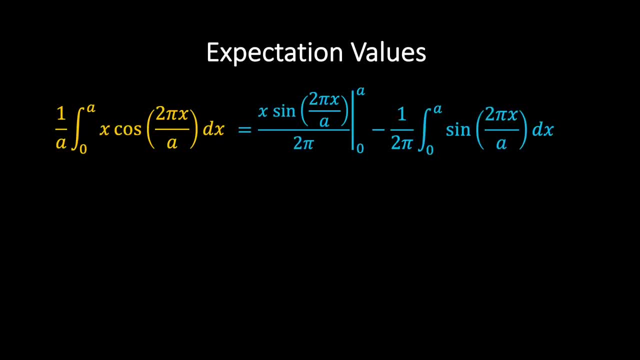 Now we immediately see that the first term in this expression vanishes and we're left with just the second term. We can integrate this expression by changing variables and letting u equal 2 pi x over a, in which case du equals 2 pi over a dx. 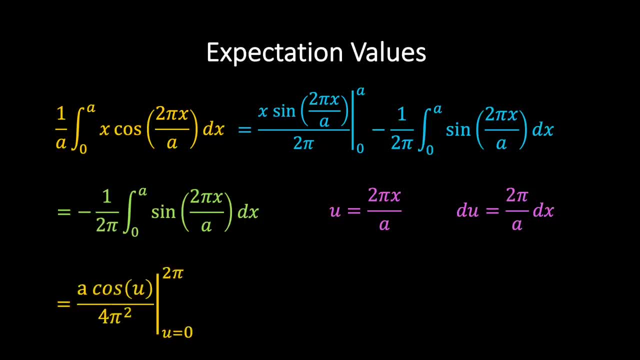 If we then perform the integration, we find the following result: which evaluates to 0.. And so, when the dust has settled, we see that the expectation value of the position of our particle in a box is simply equal to a over 2.. 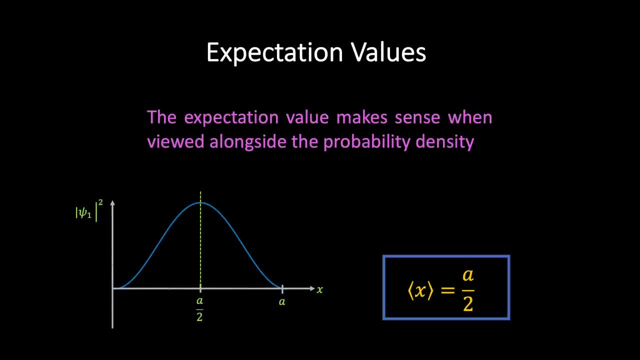 And this is precisely the result that we might have expected based on the plot of the modular squared of the wave function. Furthermore, we see that the expectation value of the position is a constant that does not depend on time. This is a characteristic feature of stationary states. 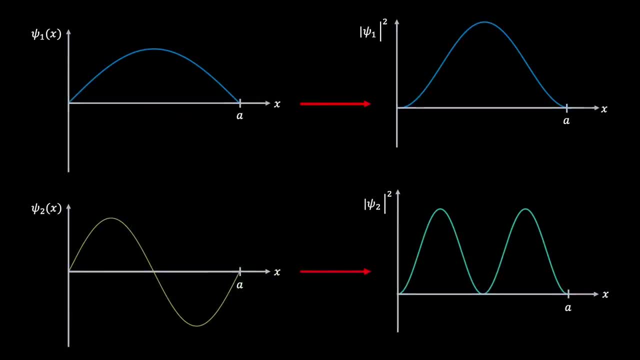 as we've already mentioned. Now, another feature of so-called stationary states is that they have a definite energy, and it's worth taking the time to show you this explicitly, If you recall the spatial shape of the wave function and therefore the spatial shape. 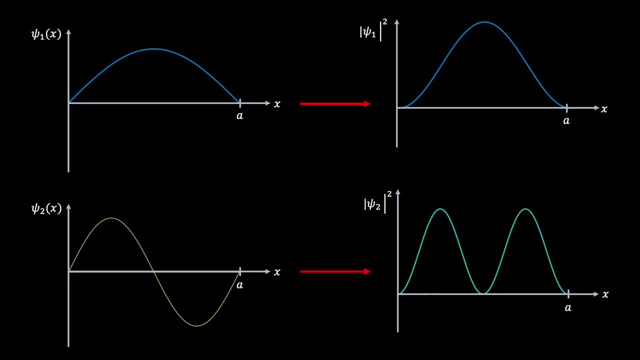 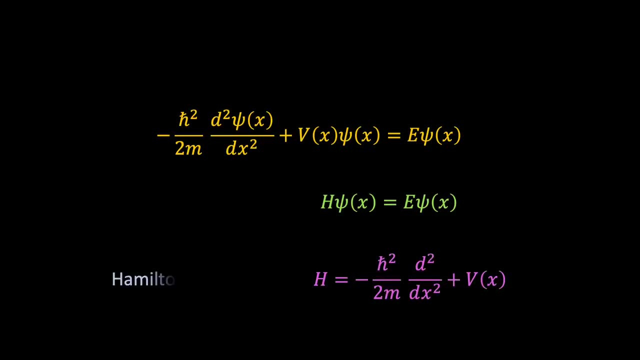 of the modular squared of the wave function is governed by the time-independent Schrodinger equation, which you will often see written in the following form: where h is referred to as the Hamiltonian operator. This equation is called the energy eigenvalue equation and, as we've already mentioned, 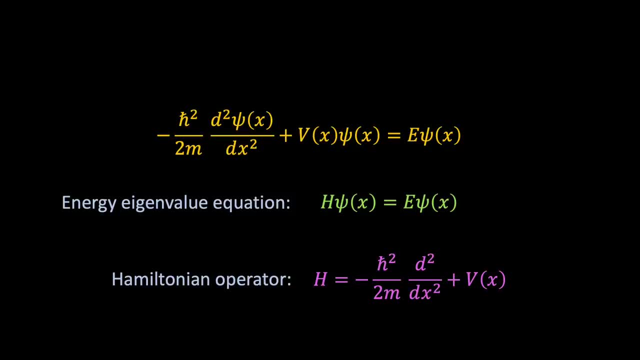 the function psi of x is referred to as the eigenfunction of the Hamiltonian with energy eigenvalues. Now, anyone who has studied eigenvalue equations in linear algebra will be familiar with this terminology. In practice, as we have seen, with the infinite square world potential, 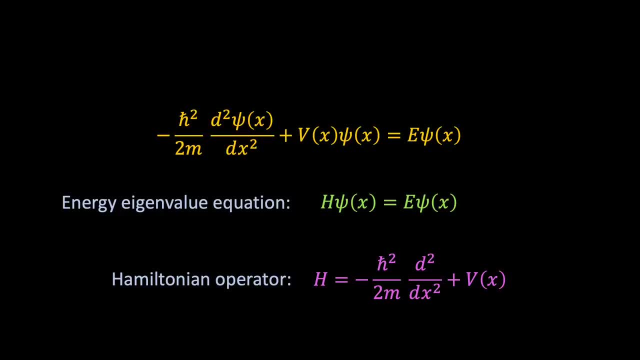 there are many eigenvalues and many eigenfunctions. An eigenfunction of the Hamiltonian operator is a very special mathematical function. When the complicated Hamiltonian operator acts upon a general function, you might expect a total mess. However, when the Hamiltonian operator 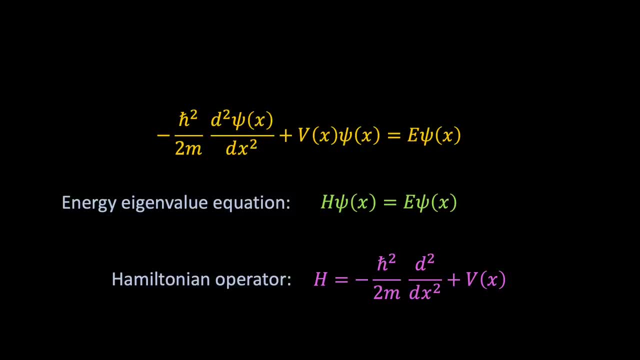 acts upon an eigenfunction, it gives the exact same eigenfunction back, only this time it's multiplied by the energy of the quantum state. Let's now use some of the probability theory we developed earlier to show that a wave function of this form represents a state with a sharply defined energy. 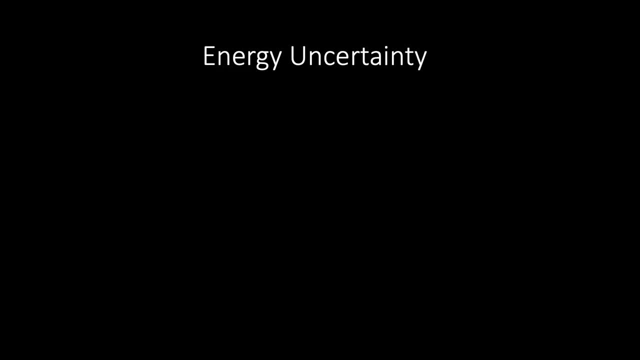 So how do we do that? Well, in general, when the energy of a quantum system is measured, the outcome is uncertain. The degree of uncertainty in the energy can be specified by calculating the standard deviation of the energy which, as we've already seen, 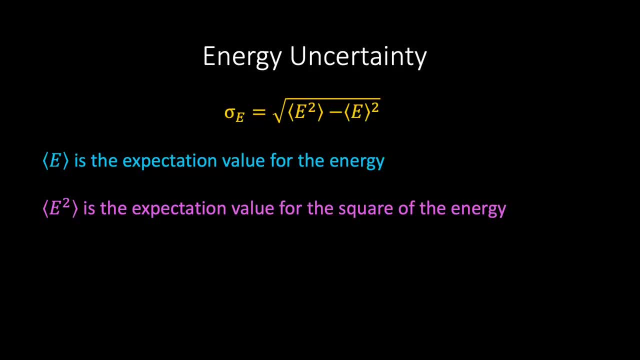 takes the following form. Now, the expectation value of the energy for a particle with a normalised wave function is given by the following integral, where we have sandwiched the Hamiltonian operator between the complex conjugate of the wave function and the wave function itself. 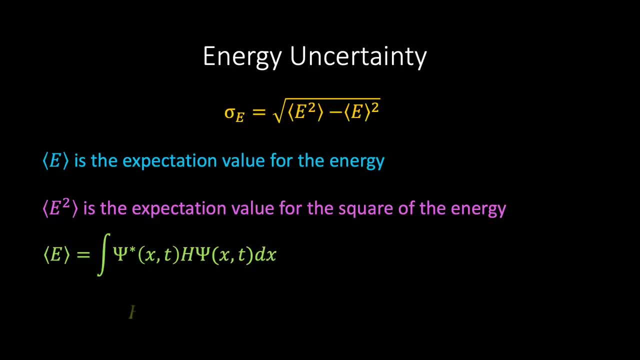 If we then simply use the energy eigenvalue equation, we see that the expectation value expression simplifies and is equal to e, where we've used the fact that the integral of the modulus squared inside the box is simply equal to 1, and so we see that the expectation value 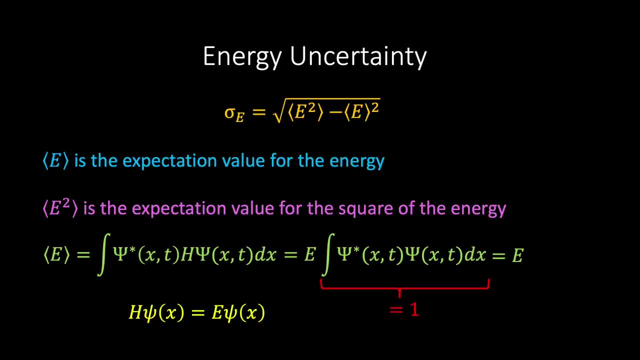 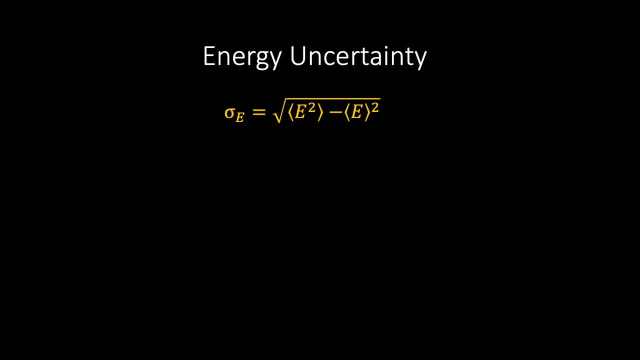 of the energy is simply equal to e. Now, if psi is an eigenfunction of the Hamiltonian, it's also an eigenfunction of the product of the Hamiltonian with itself, And so it follows that the following relationship is true. We can then use this to find the expectation value. 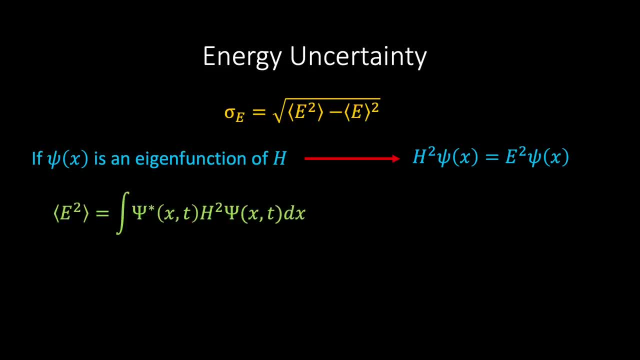 of the energy squared, which is given by the following equation: And if we use the eigenvalue equation, we see that this simplifies to e squared. And so if we combine our results, we see that the standard deviation in the energy 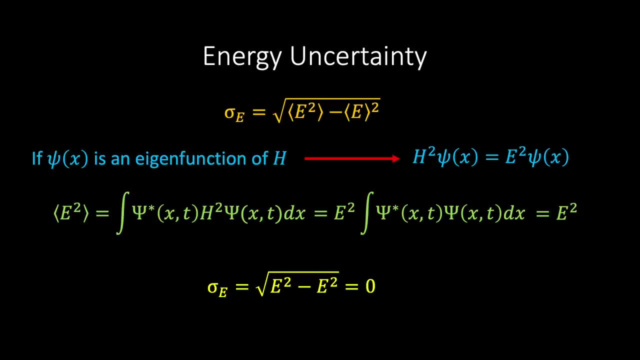 aka the uncertainty in the energy is exactly zero. So what does this mean? This is telling us that the result of an energy measurement is certain to be e when the wavefunction is an eigenfunction of the Hamiltonian operator with eigenvalue e. 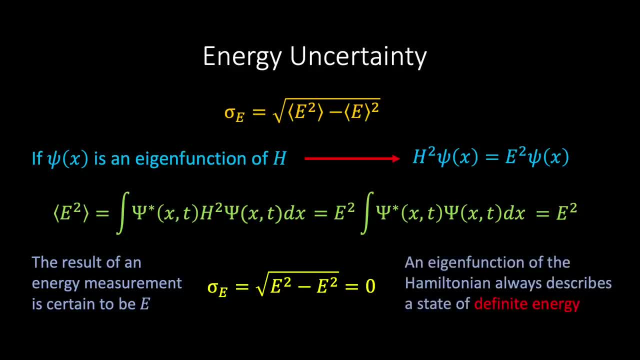 And so we conclude that an eigenfunction of the Hamiltonian always describes a state of definite energy, and these states of definite energy are exactly the stationary states that we mentioned earlier, when we said that the probability density does not change with time. Now, at this stage, 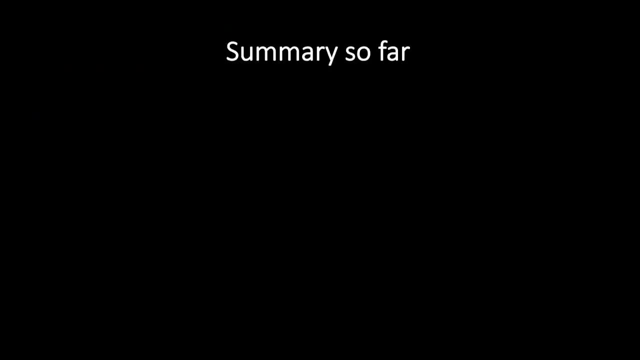 it's probably worth taking a moment and summarising some of the key points we've covered so far. We began by writing down the general time-dependent Schrodinger equation, which describes a particular quantum mechanical system. once we've specified the potential energy function, 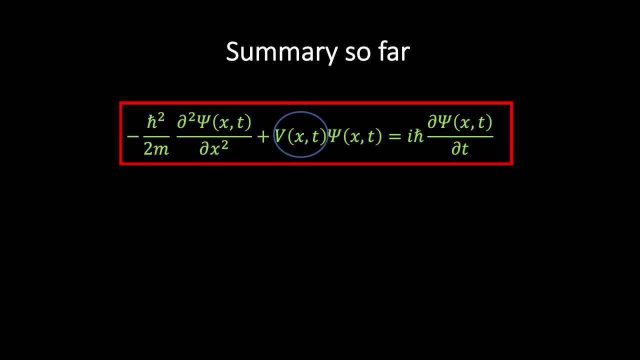 We found that if the potential energy is time-independent, then we can use the separation of variables approach and write the general wavefunction as a product of two terms: one involving space and one involving time. This then allowed us to rewrite the Schrodinger equation. 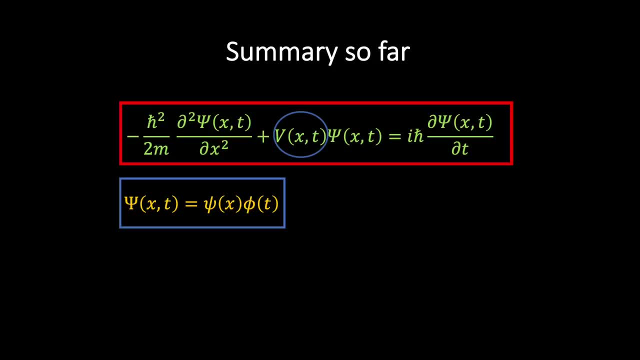 as two separate differential equations, one involving only spatial coordinates and one involving only time coordinates. By solving the time equation, we found that the time-dependence can be described by an exponential function of the following form, where e represents the corresponding energy of the state. 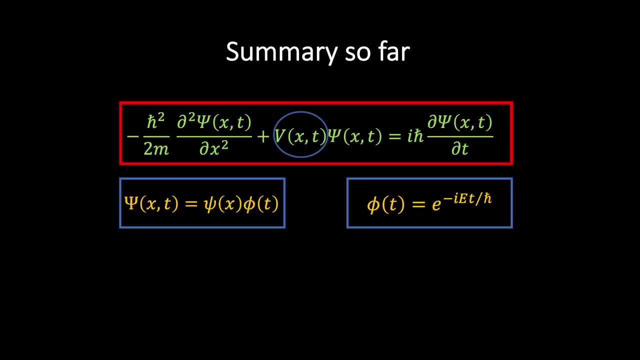 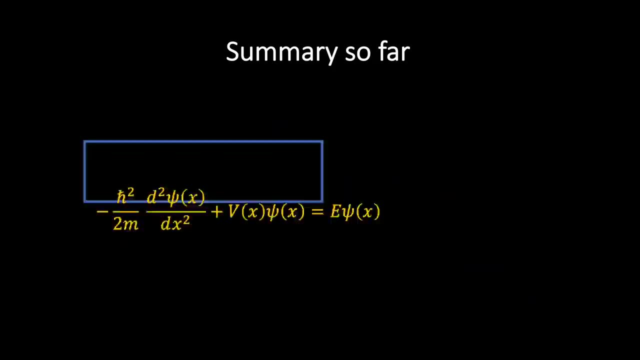 On the other hand, the spatial equation, which is aptly named the time-independent Schrodinger equation, was found to take the following form: Next, we saw that the time-independent Schrodinger equation can be written as an energy eigenvalue equation: 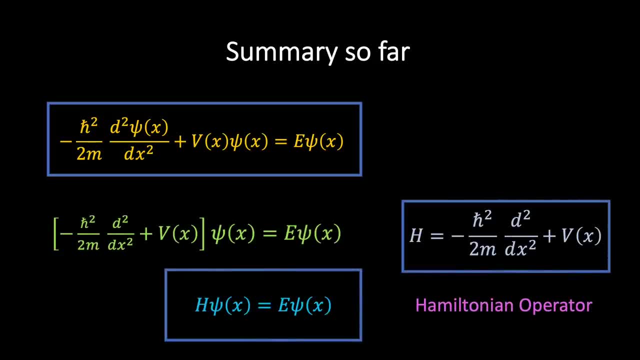 involving the Hamiltonian operator, and that the eigenfunction solutions of this equation describe stationary states in the sense that all probabilities and expectation values are independent of time and the energy uncertainty of these states is zero, so that the energy of each state is well defined. 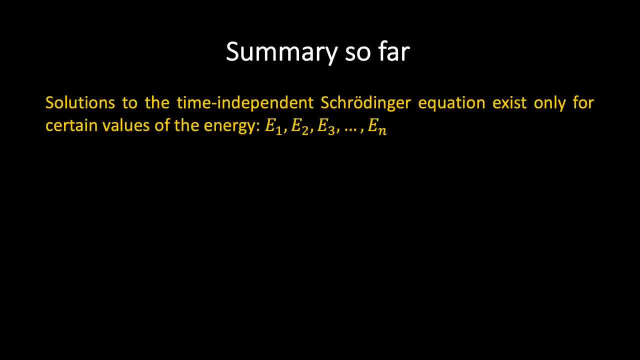 We also found that acceptable solutions to the time-independent Schrodinger equation exist only for certain discrete values of energy, and these energies are precisely the energy eigenvalues that we've already referred to, and corresponding to each eigenvalue is an energy eigenfunction. 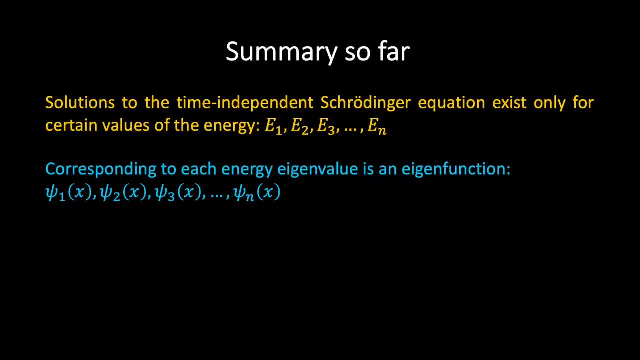 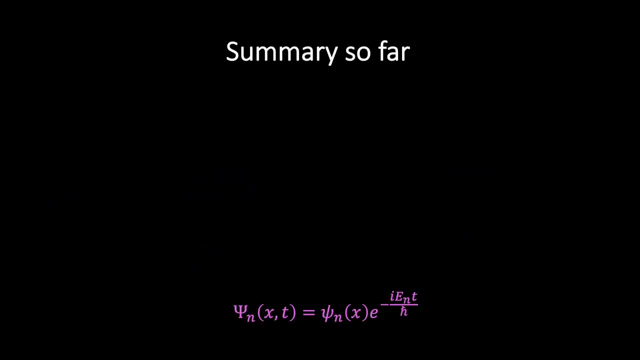 which is a solution to the time-independent Schrodinger equation. for a given potential energy function For each eigenvalue we can construct the corresponding wavefunction by simply tacking on the time-dependence The index n, which takes on successive integral values. 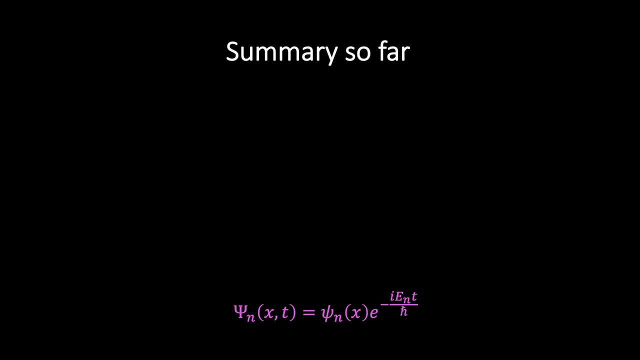 and which is employed to designate a particular eigenvalue. eigenfunction and wavefunction is called the quantum number. If this system is described by the wavefunction psi subscript n, it's said to be in the quantum state n and each of these quantum state wavefunctions. 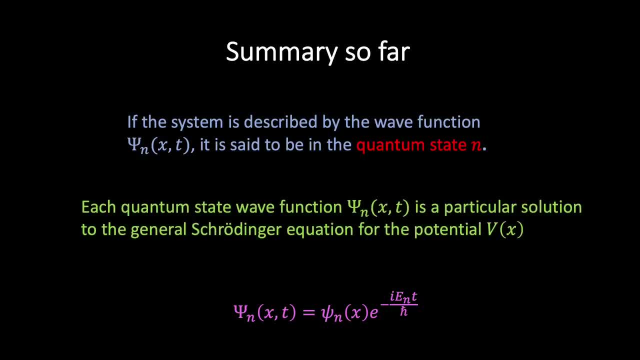 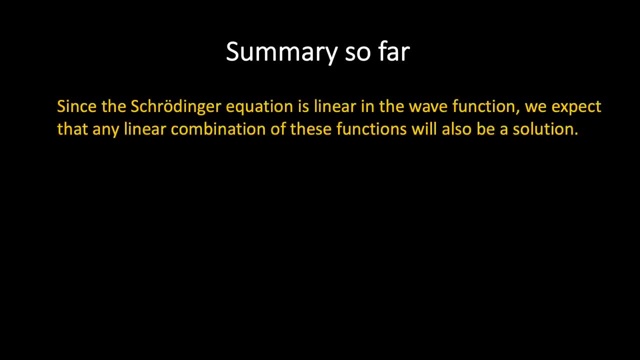 is a particular solution to the general Schrodinger equation for a given potential energy function. Now, since the Schrodinger equation is linear in the wavefunction, we expect that any linear combination of these wavefunctions will also be a solution to the Schrodinger equation. 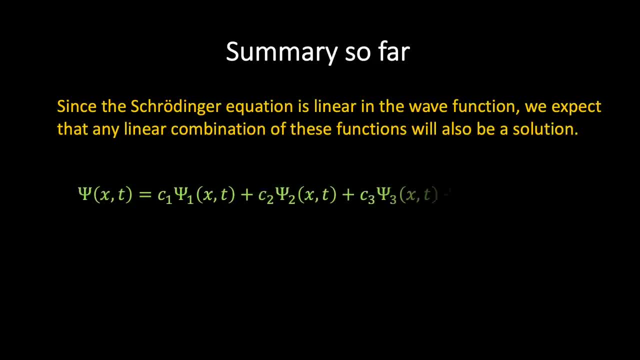 In other words, we should be able to write an expression of the following form, and this should also be a solution to the Schrodinger equation. In fact, this expression gives the most general form of the solution to the equation for a given potential function. 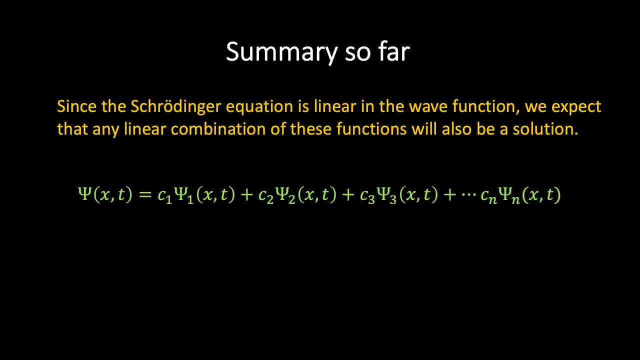 and this is often referred to as a linear superposition of quantum states. Its generality can be appreciated by noting that it is a function which is composed of a very large number of different eigenfunctions combined in proportions governed by the constant c. So once we've found 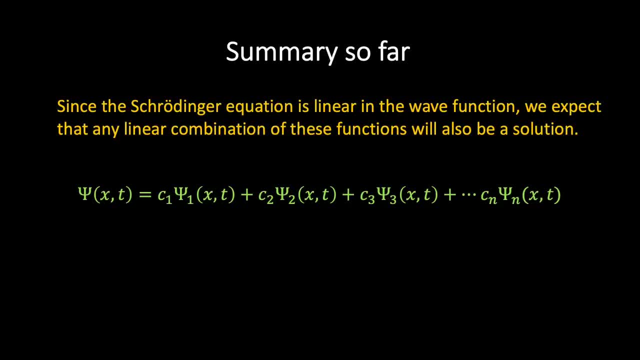 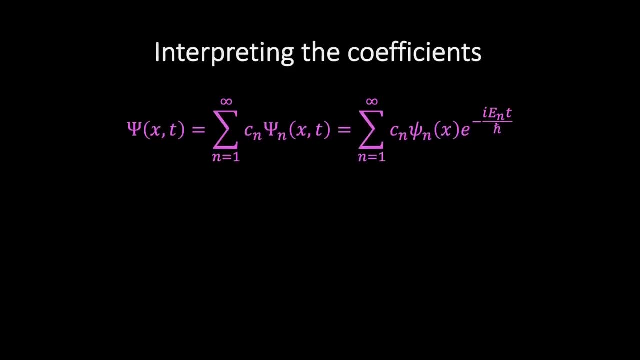 the separable eigenfunction solutions of the time-independent Schrodinger equation, we can immediately construct a more general solution of the following form: Now you may be wondering what the coefficients c, subscript n, represent physically. To find out, we're going to have to work. 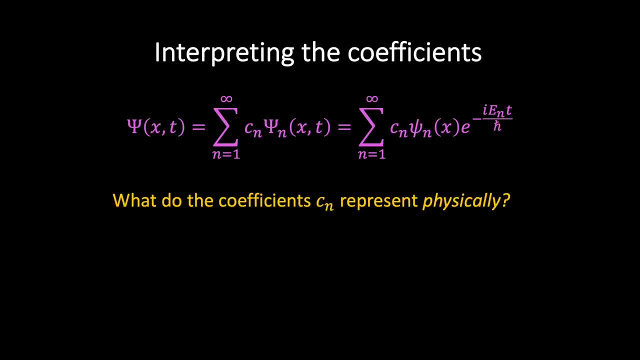 through a few calculations. so buckle up. Let's begin by normalising the general wavefunction expression which, as you now know, requires that the integral of the modulus squared of the wavefunction is equal to 1.. For our general wavefunction, 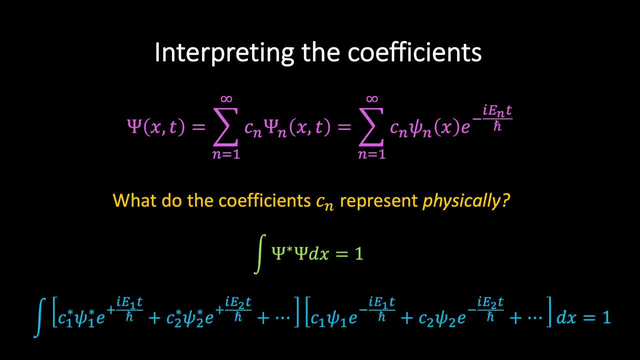 we need to then evaluate the following integral. Now, hopefully you can see, by staring at this expression long enough, that when we multiply out the square brackets, this integral will contain two types of terms. Firstly, there will be cross terms involving different energy eigenstates. 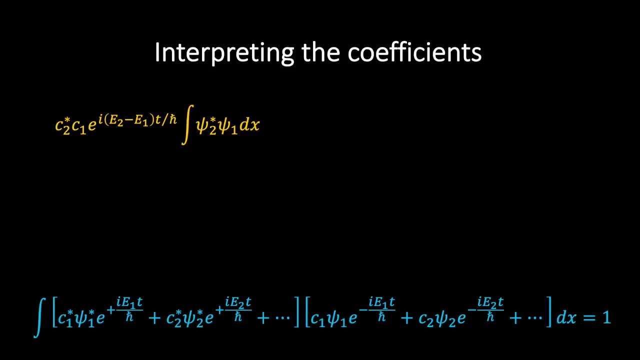 and these terms will have the following form: In this particular example, we see that we have the complex conjugate of the n equals 2 eigenstate being multiplied by the n equals 1 eigenstate. Secondly, there will be terms of the following form: 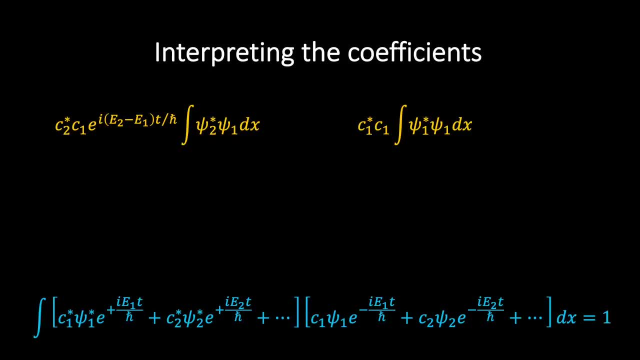 which involve the same eigenstate. So how do we deal with these integrals? Well, the second type of integral is easy to evaluate, since we can use the normalisation condition, which tells us that the integral of the modulus squared of an energy eigenstate. 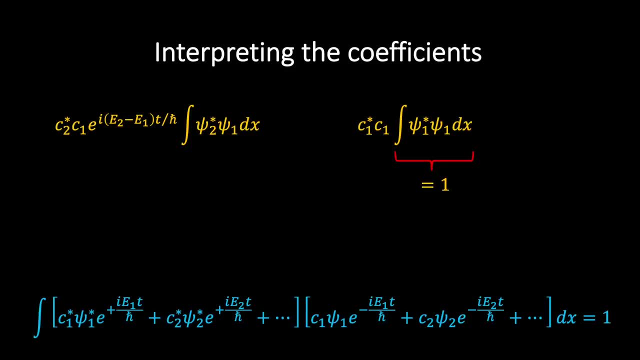 is simply equal to 1.. And so we can write this particular term as simply the modulus squared of the coefficient c1, and therefore, in general, we will find the following result: But what about the first type of integral, which involves cross terms? 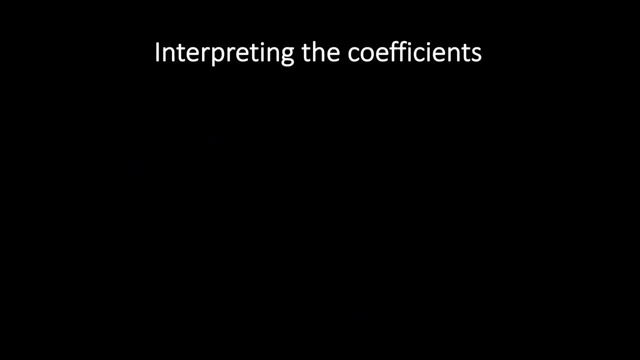 How do we evaluate this? Well, we can in fact show that all of these cross term integrals will vanish, and to do that, let's consider a general cross term integral of the following form, where m and n take on different integer values. 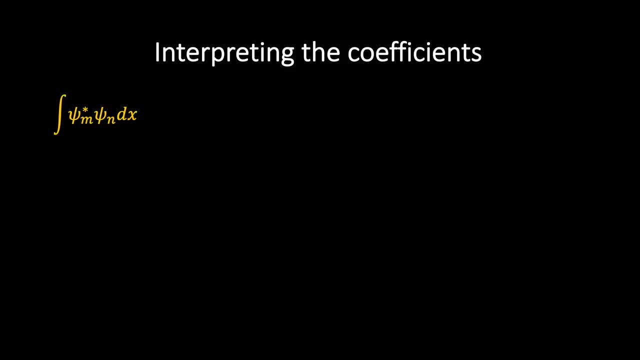 Next, if we sub in the expressions we derived earlier for the energy eigenstates for a particle in a box, then we find the following yellow expression: We can simplify this expression by the integral, by rewriting the product of sign terms using the following well-known trigonometric identity: 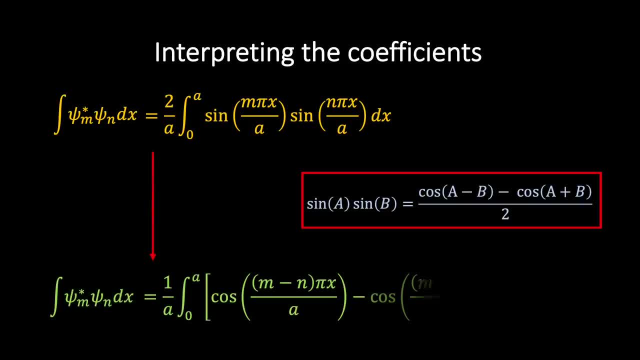 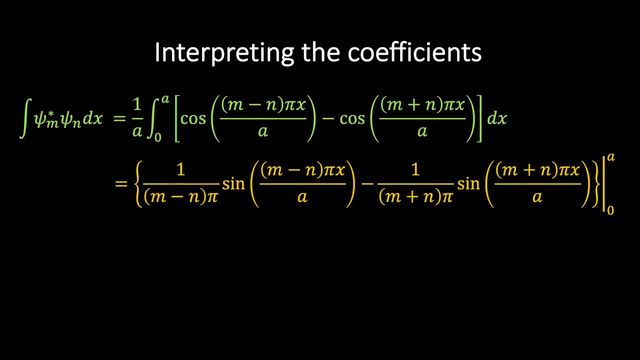 in which case we find that our integral takes the following form: If we then evaluate this integral, we find the following slightly intimidating expression. But if we then sum in the limits of the integral, we find something slightly more compact and we can in fact see: 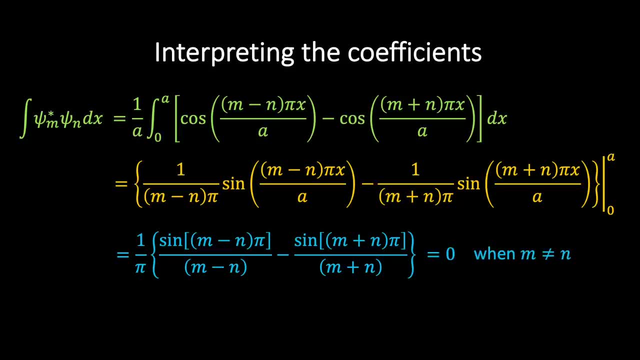 that this is equal to 0 when m is not equal to n, since in this case we will have an integer multiple of pi inside each of the sign terms and therefore the whole integral will be equal to 0.. This condition is often referred to. 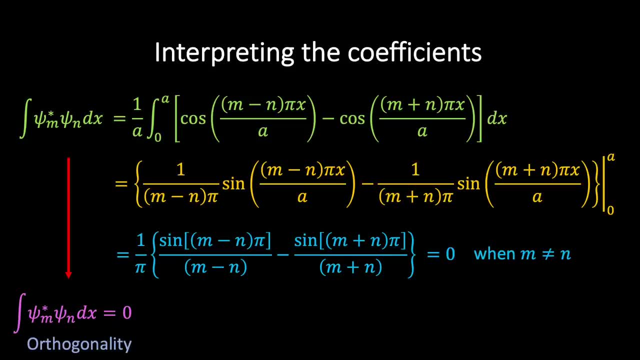 as orthogonality, and the two different eigenstates represented by m and n are said to be orthogonal to each other. Now it's worth noting that this argument does not work when m equals n. In that case, we have to use the normalisation condition. 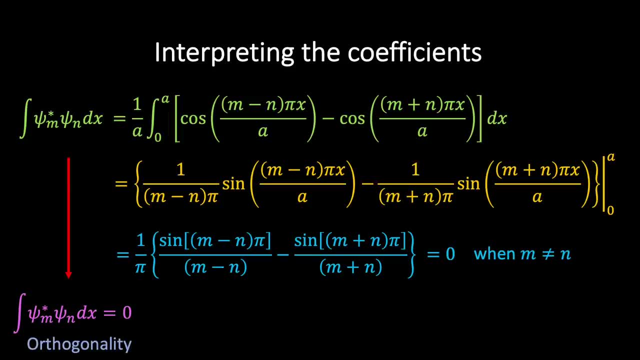 which tells us that when m equals n, the integral will be equal to 1.. In fact, it's customary to combine both orthogonality and normalisation into a single statement, which takes the following form: Here, delta m n is referred to as 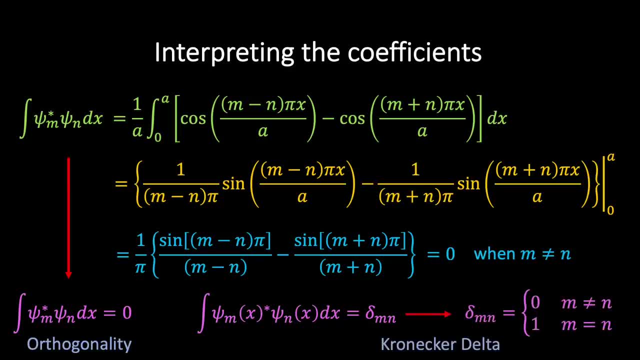 the Kronecker delta and is defined by the fact that when m equals n, it's equal to 1, and when m is not equal to m, the Kronecker delta is equal to 0.. And finally, we say that the eigenstates 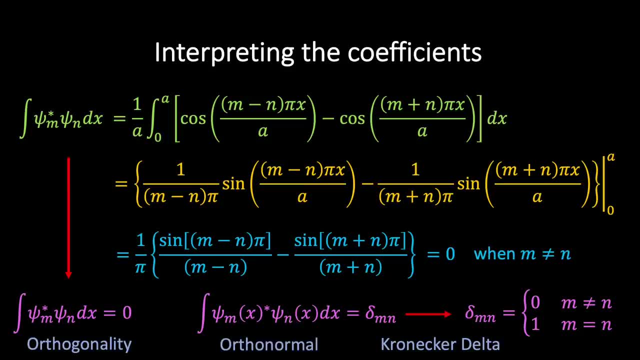 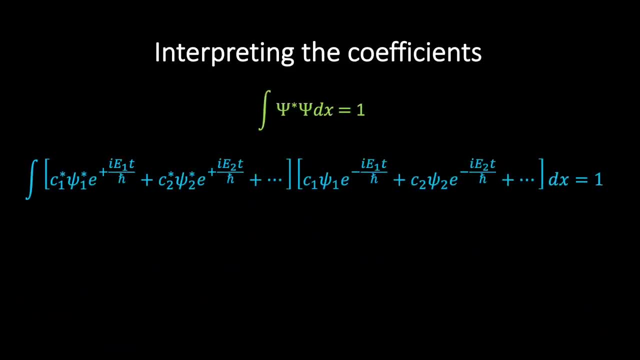 satisfying this condition are orthonormal. And so, after that slight detour, let's return to the job at hand, which was to normalise our general wavefunction. And we now see that, armed with the orthogonality relation, 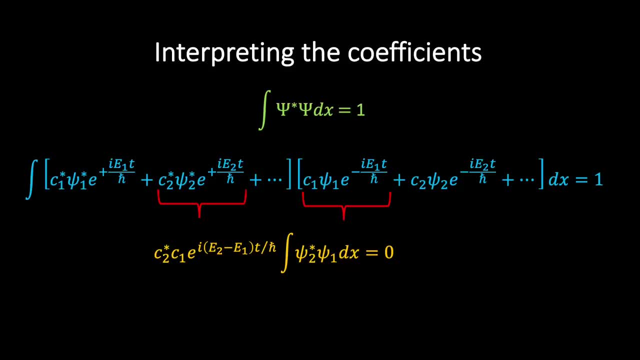 that the cross terms will vanish because the eigenstates are orthogonal to each other and terms involving the same eigenstate will not vanish due to the normalisation condition. And so it turns out that, in order to normalise our general wavefunction, the coefficients must satisfy. 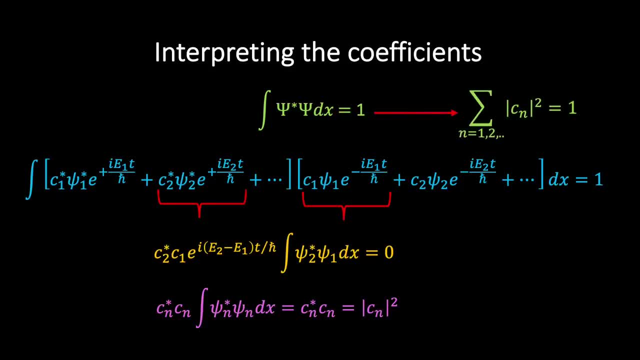 the following condition: OK, but this still doesn't tell us what the coefficients actually represent. To gain a bit more insight, let's calculate the expectation values for the energy and energy squared corresponding to this general wavefunction. As we've already seen, 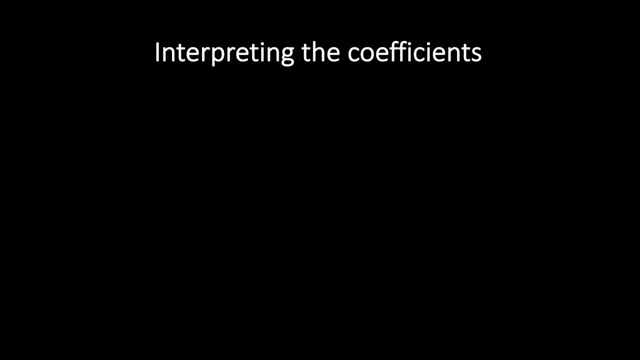 we can calculate the expectation value of the energy using the following green equation: And. we can calculate the expectation value of the energy squared using the following yellow equation. Now, in order to evaluate these integrals, when the wavefunction is a superposition of eigenfunctions, 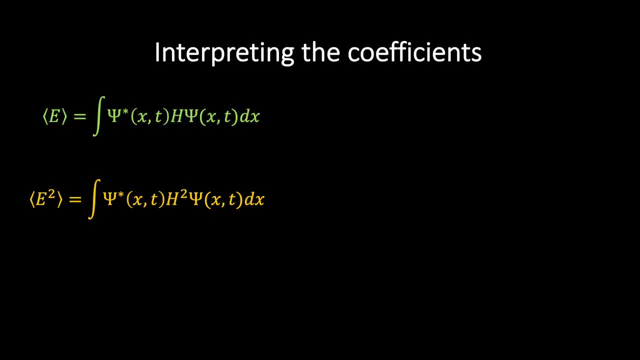 we use the energy eigenvalue equations we encountered earlier, as well as the orthonormal condition. If we then make use of these relations to evaluate the expectation value integrals, we find that the expectation value of the energy is given by the following green expression: 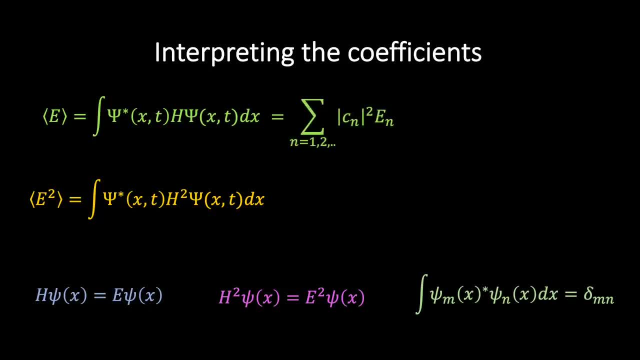 and the expectation value of the energy squared is given by the following yellow expression: And so we see that we're finally in a position to answer the question we originally posed, namely what is the physical meaning of the complex coefficients? If you recall from our discussion, 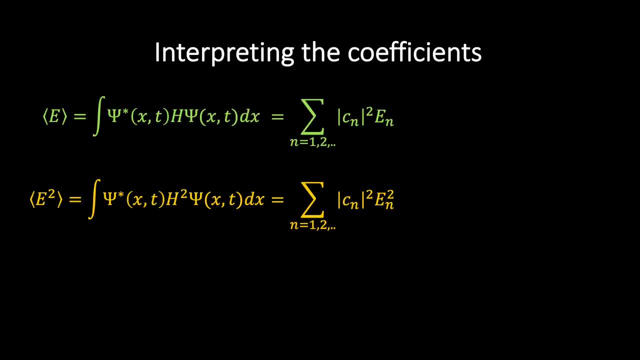 on probability theory, the expectation value of some variable x is given by the following expression: And if we compare this with our expressions for the expectation values of the energy and energy squared, we see that for a given value of n, the modulus squared of the coefficient 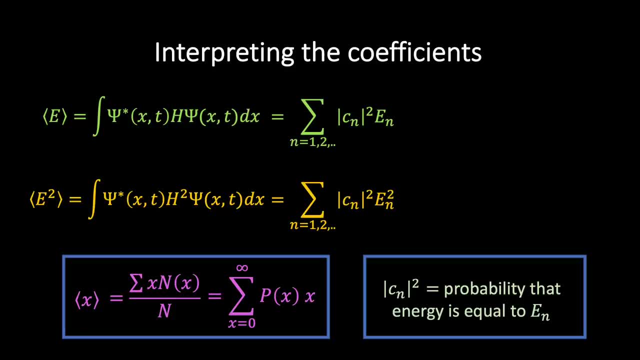 represents the probability that a measurement of the energy will return the value e, subscript n, And this fits perfectly with the normalisation condition that we found earlier, which said that the sum of the modulus squared of the coefficients must be equal to one. This is simply the statement. 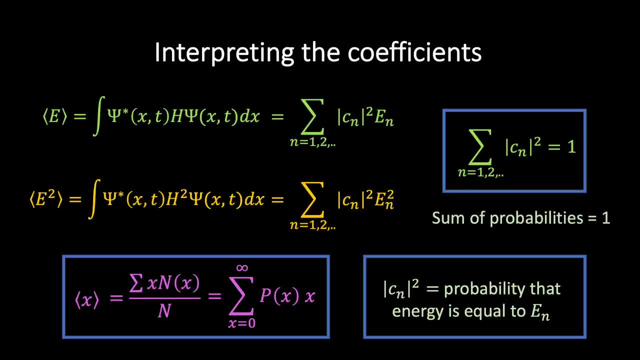 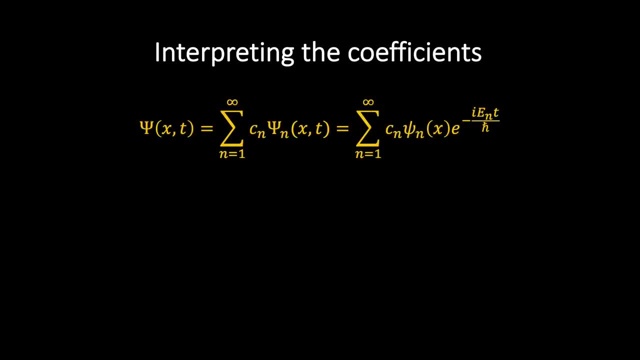 that the sum of the probabilities of measuring each energy state must be equal to one. And so, to summarise, we found that when the wave function corresponding to a particle in a one-dimensional, infinite square world potential is expressed in its most general form as a linear superposition, 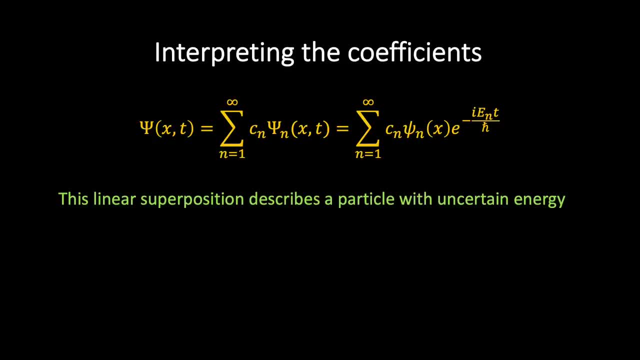 of energy eigenstates, then this linear superposition describes a particle with uncertain energy, And the probability of measuring a particular energy eigenvalue is given by the modulus squared of the coefficient of the corresponding term in the linear superposition. Now I must admit, 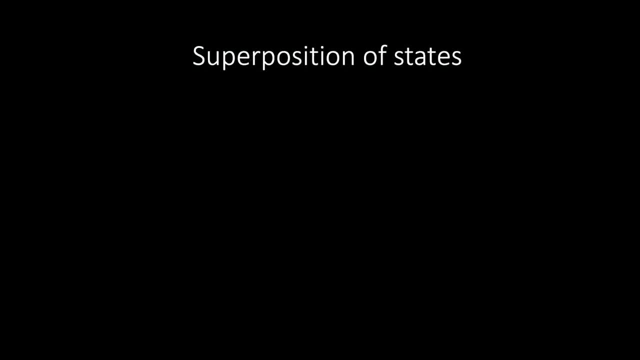 this has all been quite heavy going and abstract so far, so let's consider a specific, concrete example of a linear superposition of states, which will highlight how this whole formalism works. Imagine that a particle in the infinite square world potential has an initial wave function. 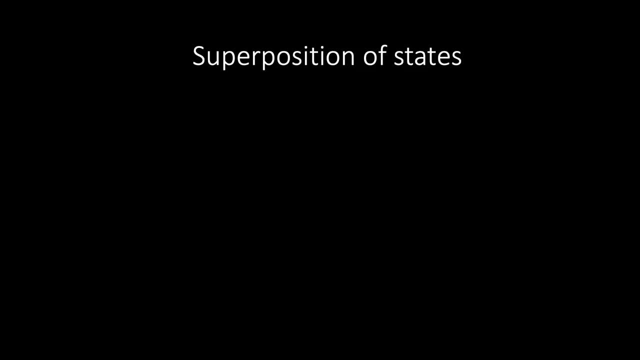 comprising an even mixture of the first two stationary states. If we sub in the expressions that we derived earlier for the normalised eigenstates of the ground state and the first excited state, we see that our linear superposition takes the following form. Now our first step. 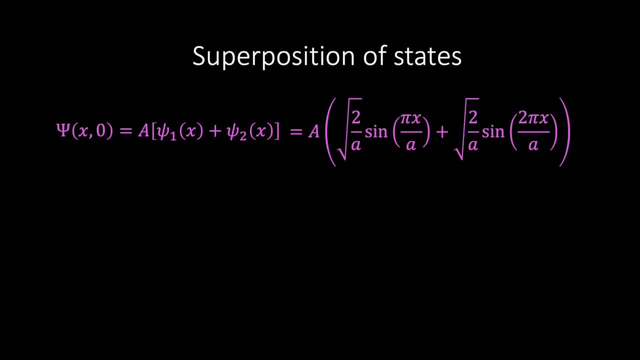 is to normalise this wave function so that we can establish the constant a. and to normalise the wave function, we require the following relationship to hold true: If we substitute our expression for the initial wave function, we find the following yellow equation: 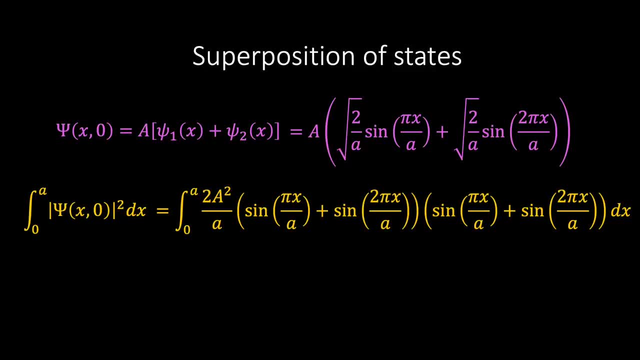 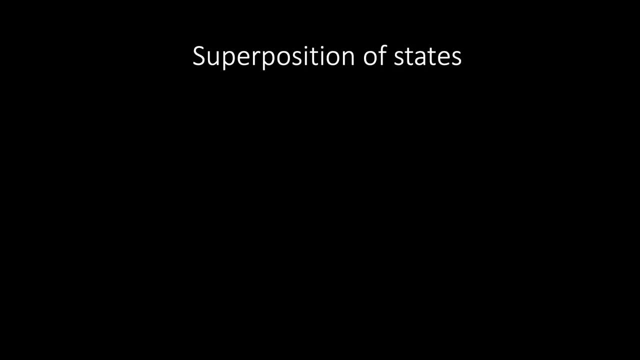 And if we then multiply out the bracket, we find the following blue expression. Next, if we rewrite the sine squared terms in terms of cosines, we find the following rather overwhelming blue expression: Performing each of these integrals is straightforward and follows the same logic. 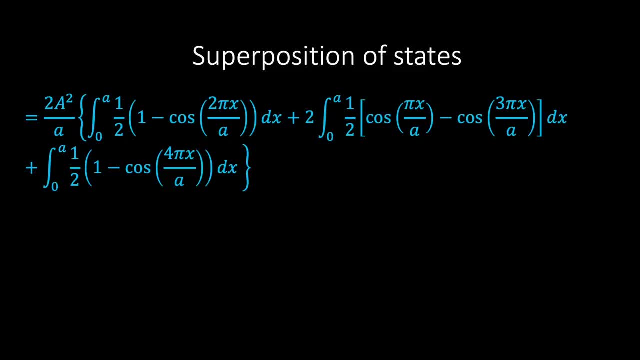 as previous examples we've looked at. When the dust settles, we find the following green expression: And then, if we sum in the limits, we finally arrive at the rather simple expression 2a squared, which must be equal to 1,. 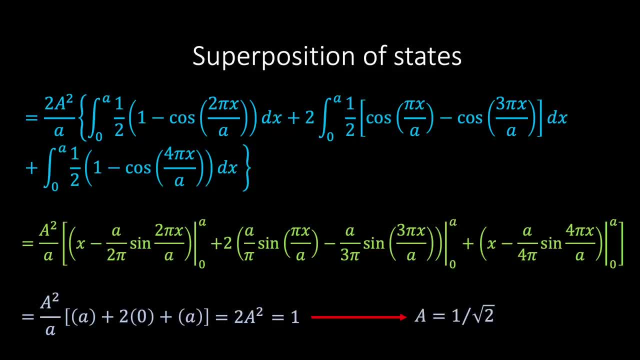 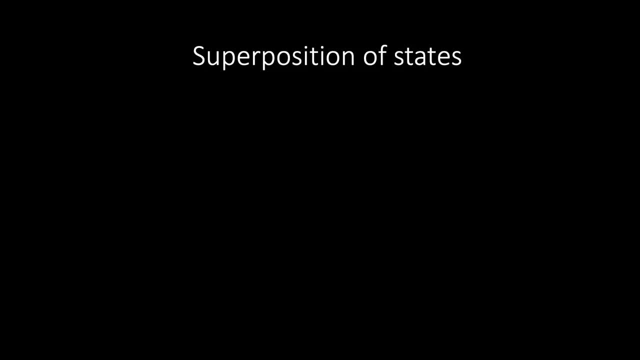 and therefore we see that a is equal to 1 over the square root of 2.. Once we've worked out the normalisation constant, we can sub this back into our original wave function expression and we get the following result: And after expanding out: 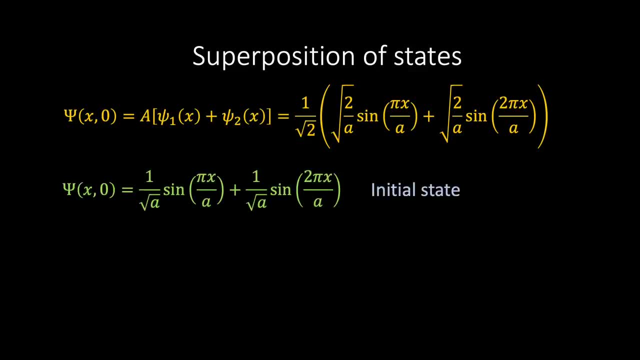 the bracket, we arrive at the following green expression, which summarises our initial state wave function. Next we want to match this up with the most general solution of the Schrodinger equation. We know from our earlier analysis of the infinite square world potential. 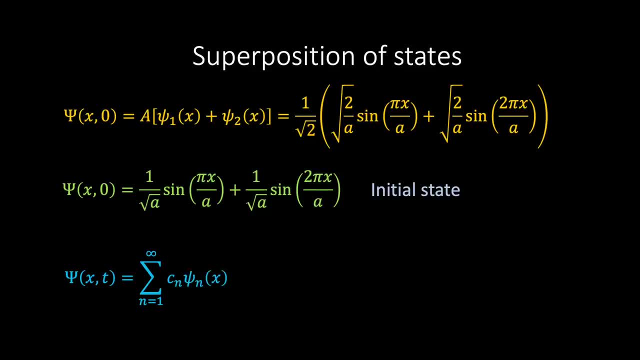 that the general solution is a superposition of eigenstates which, in the specific case of the infinite square well, takes the following form: The next step in our strategy is to set t equals to 0 and then match coefficients with our initial wave function. 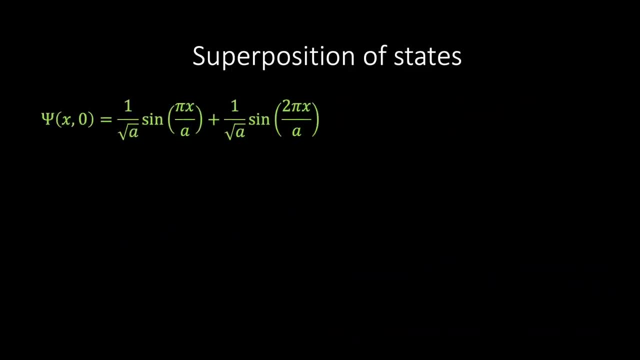 So let's do that. If we take our initial normalised wave function and compare the coefficients, term by term, with the most general wave function for the infinite square, well, we find from matching the first term that c1 equals 1 over root 2.. 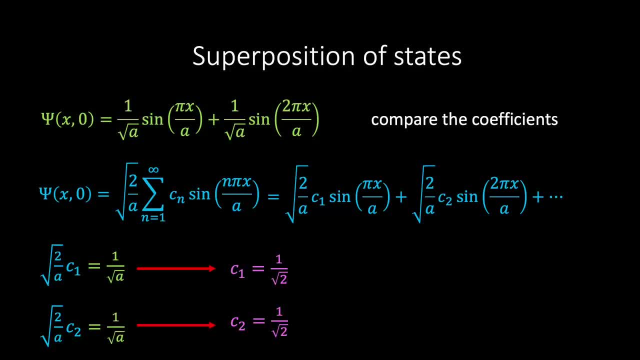 Likewise, by matching the second terms, we find that c2 also equals 1 over root 2.. And finally, we see that cn equals 0 when n is greater than or equal to 3.. And now that we've determined the coefficients, 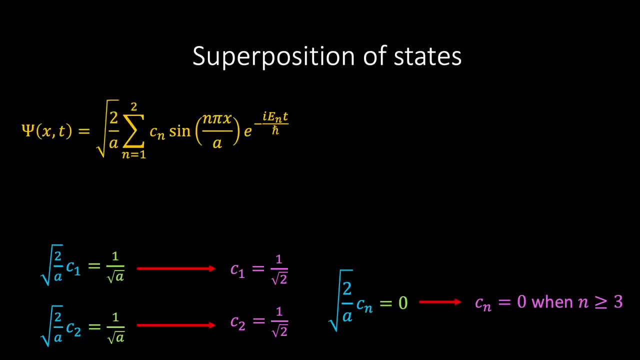 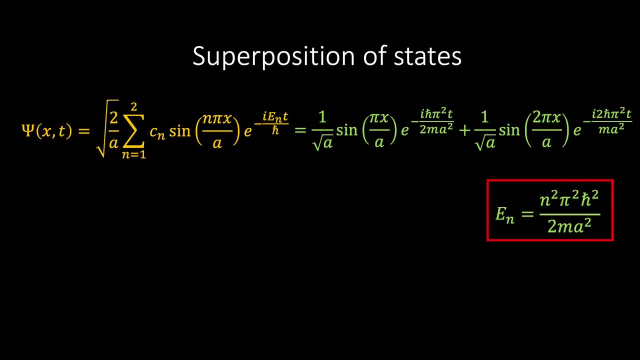 we can substitute these into our general wave function and we find the following green expression, where we've also substituted the values for e1 and e2 using the energy equation that we derived earlier. Next, we recall from the Einstein-De Broglie relation: 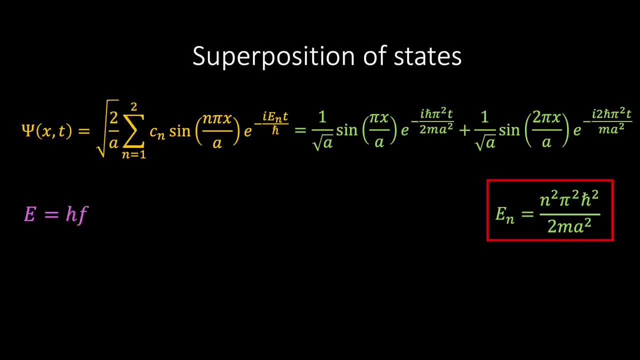 that the frequency is related to the energy by the equation e equals hf And therefore it follows that the angular frequency is related to the energy via the equation omega equals e over h bar, And therefore we see from the first exponential term that we can equate omega 1. 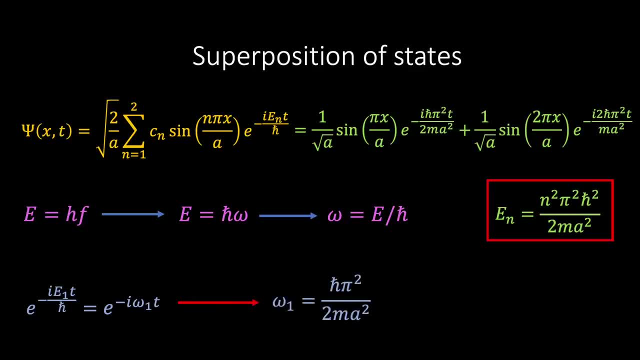 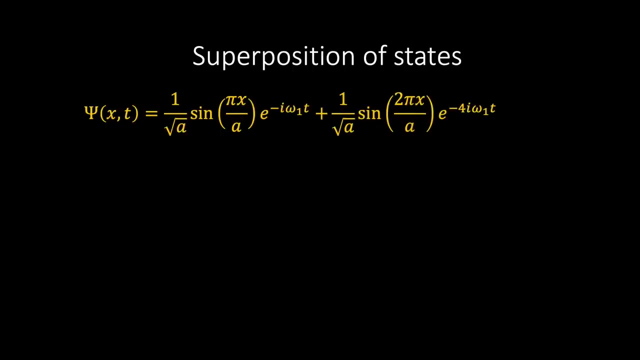 as being equal to h bar pi squared over 2ma squared, And we see from the second exponential term that we can write: omega 2 is equal to 4 times omega 1.. It then follows that our general wave function takes the following form: 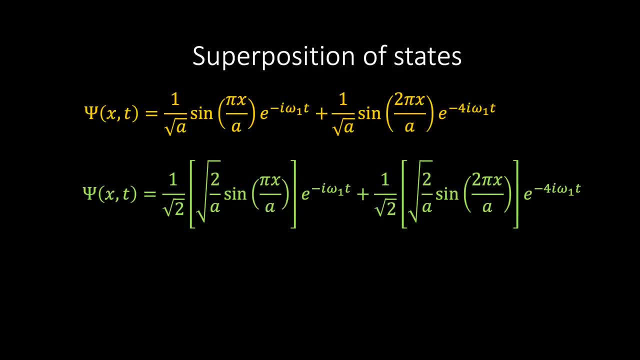 And we can then pull out a factor of 1 over root 2 and rewrite this explicitly in terms of the energy eigenstates of the infinite square. well, by noting that the term inside the first square bracket is simply the first eigenstate: psi 1,. 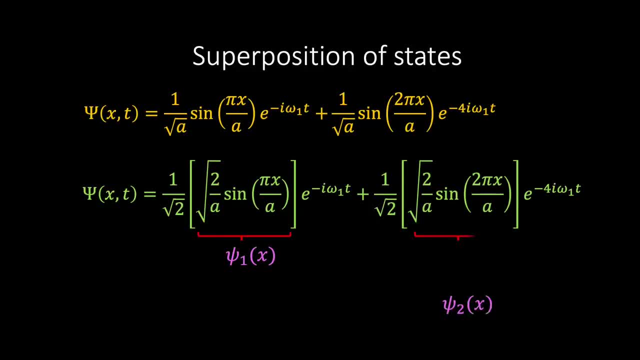 and the term inside the second square bracket is the second eigenstate, psi 2.. And therefore we can write our general wave function explicitly in terms of the first two energy eigenstates in the following way. Now one of the advantages of doing this: 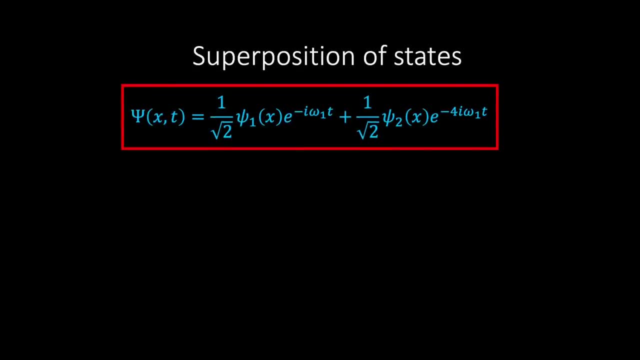 is that we can simply read off the probabilities of finding the particles in each of these energy eigenstates, as this information is contained in the coefficients of the two eigenstates appearing in the general wave function expression, In particular the probability of measuring the energy of the particle. 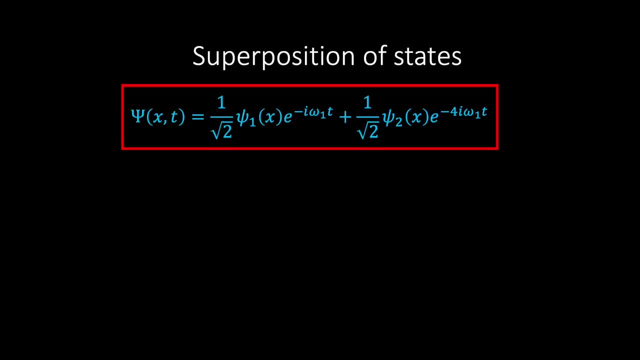 and finding the energy to be the eigenvalue, E1 is simply equal to the square of the coefficient of the first term, and we see that this gives an answer of 1 half. Likewise, the probability of finding the particle with energy, E2, is also equal to 1 half. 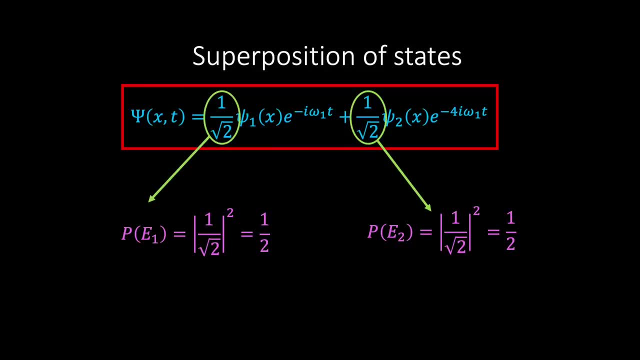 And so we see that the measurement of the total energy of the particle could lead to either of two results: the eigenvalue E1 or the eigenvalue E2.. This is telling us that there is an inherent uncertainty in the energy of the particle. 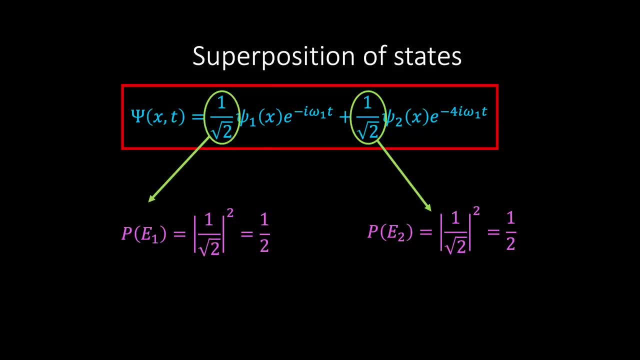 due to the fact that the wave function is a linear combination of two different energy eigenstates. To clarify this point, let's calculate the energy uncertainty which, as we saw earlier, involves calculating the standard deviation of the energy. Let's begin by calculating. 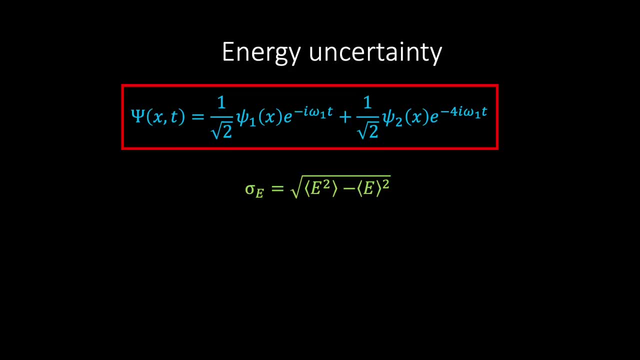 the expectation value of the energy, which is simply equal to the probability of measuring E1 multiplied by the energy E1, plus the probability of measuring E2 multiplied by the energy E2.. If we put the values in, we find the following expression: 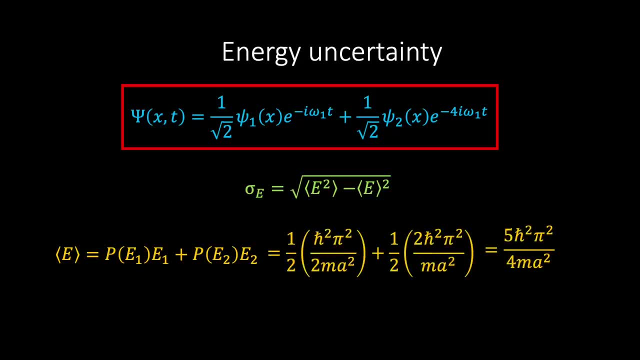 for the expectation value of the energy. This is telling us that if we prepared an infinite number of identical ensemble states and measured the energy of each of these states and then calculated an average, this is the value that we would obtain. Next we can calculate. 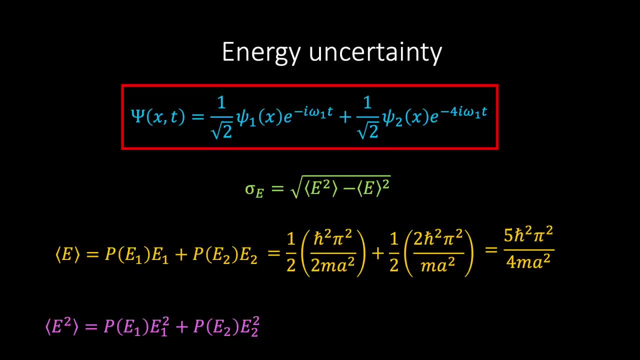 the expectation value of the square of the energy, which, after a simple calculation, results in the following expression: Now, if we sub these expressions into the standard deviation equation, we see that the uncertainty in the energy is not zero. And so we see that. 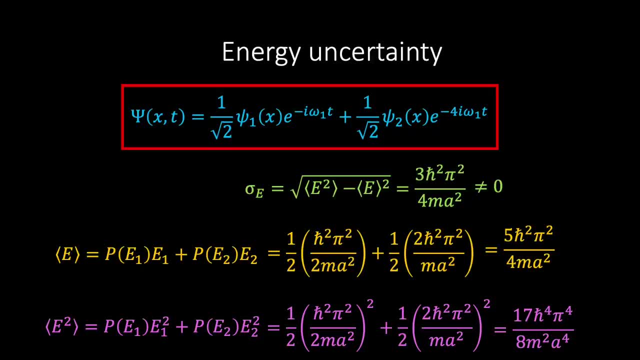 by forming a linear combination of states, we have introduced uncertainty into the energy of the particle, which is exactly what we expect based on our earlier discussion. Quantum states with uncertain energy are called non-stationary states because they have some observable properties that change with time. 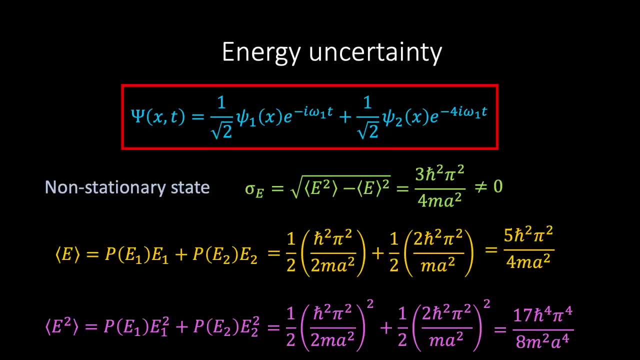 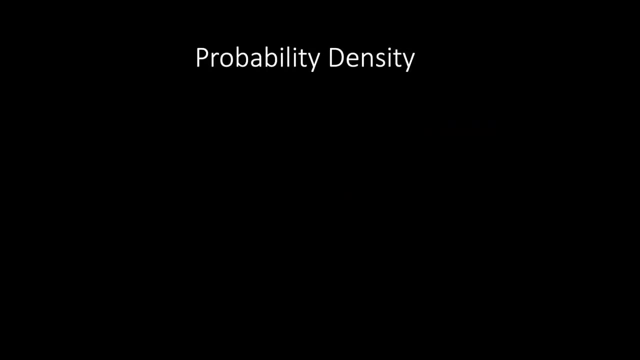 For example, we will now show that the probability density and position expectation value corresponding to this wave function will oscillate in time. So let's do that. Let's begin by calculating the probability density corresponding to our general wave function. As we've seen many times now, 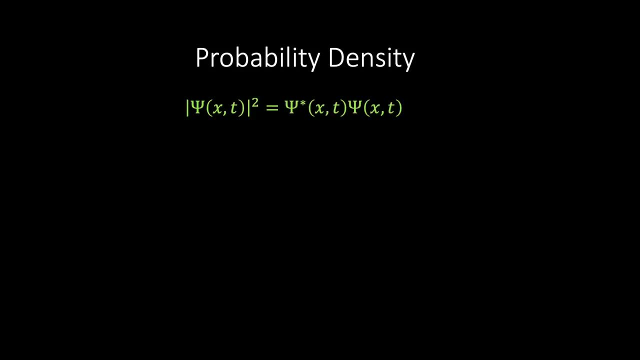 the probability density is given by the modulus squared of the wave function. And if we then sub in the general wave function we determined earlier, we find the following yellow expression. Next, if we multiply out the brackets and carefully group terms, we find this beautiful blue expression. 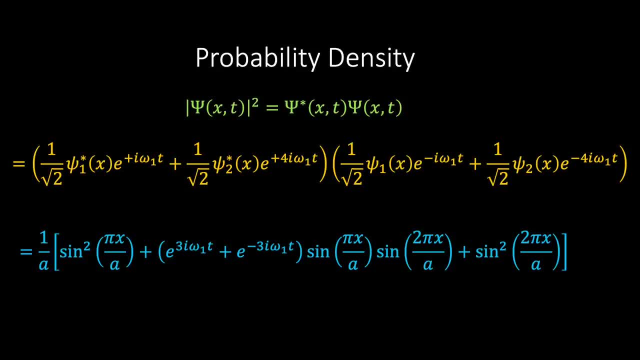 Now, the reason we have written it like this is because we can then use Euler's equation, which was introduced earlier, to write this term as 2cos, In which case we arrive at pure perfection in the form of this purple expression. 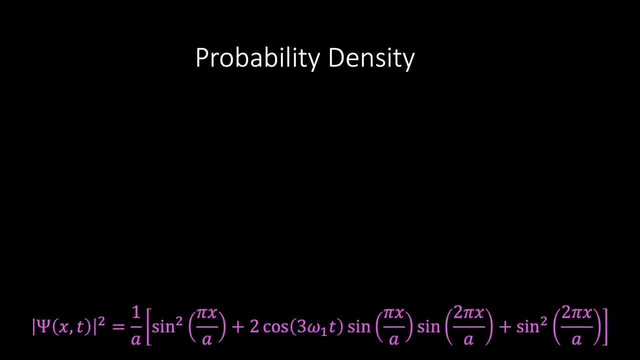 Now we immediately notice, by staring at this expression, that the probability density is a function of time. This was not the case when we were looking at the probability density for a single energy eigenstate. However, here, the linear combination of energy eigenstates. 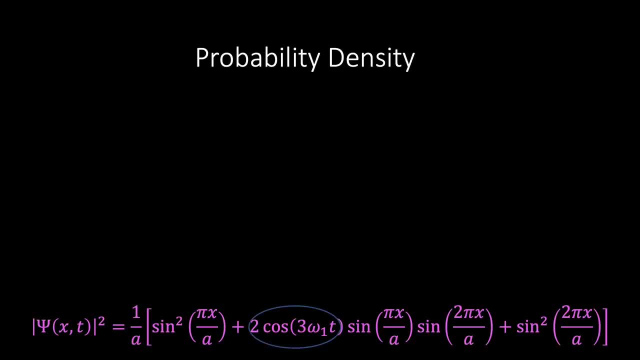 has led to a cos3ωt term. To gain a bit more insight into how this term affects the probability density and to help visualise what's going on, let's plot a graph of probability density on the y-axis and x-position on the x-axis. 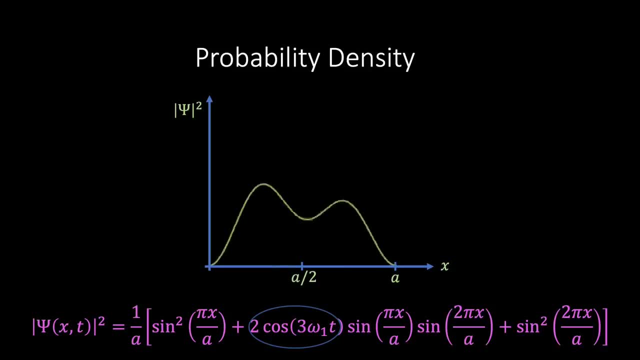 We see that the presence of the time cosine term has caused the probability density curve to oscillate back and forth about the centre of the box with a characteristic frequency, Since the probability density tells us information about where we're most likely to find our particle. 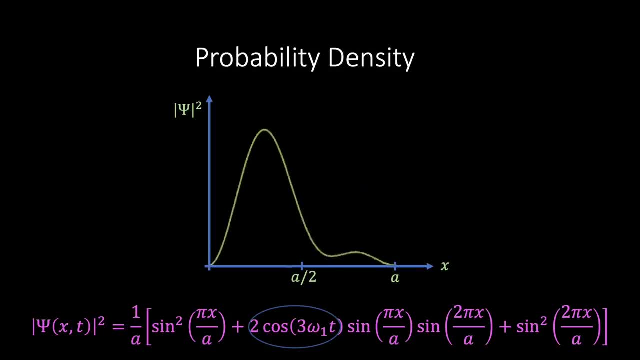 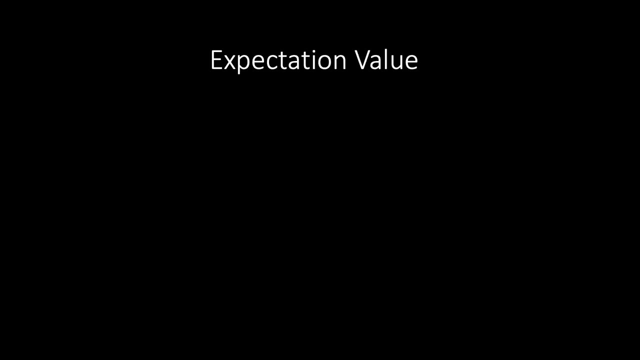 and since the probability density is changing with time, this is telling us that the location of where we're most likely to find the particle is also changing with time. To help understand this in a bit more detail, let's look at the expectation value of the position of the particle. 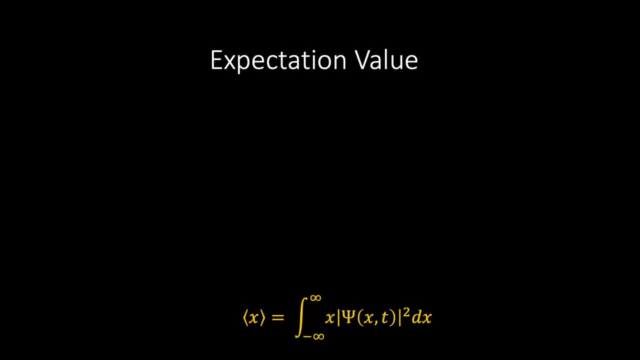 described by this simple linear superposition. Now I won't go through the details of this calculation, but it's safe to say that it follows in the same spirit as the other calculations that we've looked at in detail. Feel free to try it yourself. 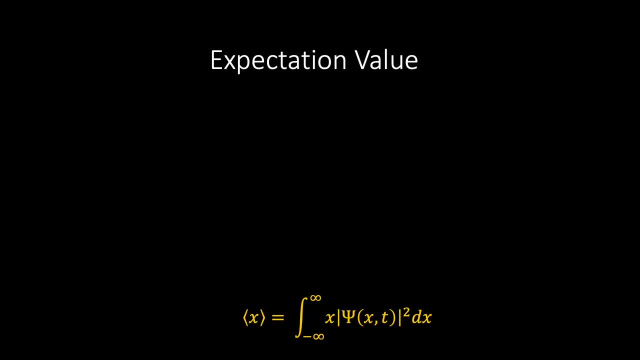 and if you do so, you should find that when the dust settles, the expectation value is given by the following compact expression: So what is this telling us? Well, this is saying that the expectation value of the position of the particle is oscillating about. 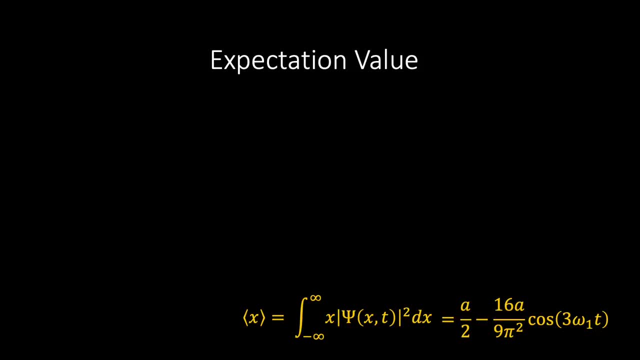 the centre of the box. To visualise this, let's superimpose the expectation value on the graph of the oscillating probability density that we looked at earlier. We see that the expectation value of x oscillates with a particular frequency. In fact, 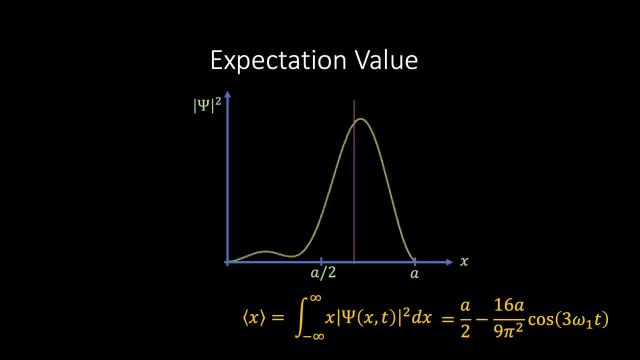 we can calculate this oscillation frequency. If you recall from earlier, we found that the angular frequency corresponding to the ground state was given by the following expression: and therefore 3 times omega. 1 is simply 3 times this, and we will label. 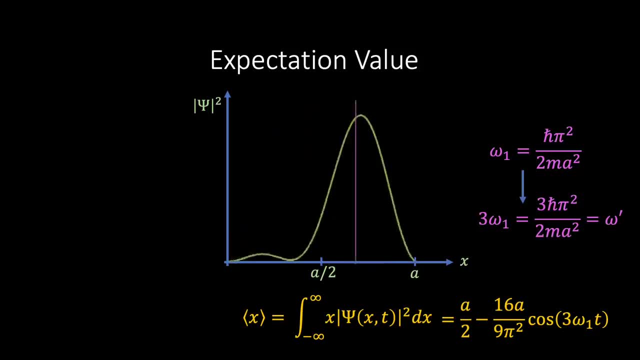 this angular frequency, omega prime. Now, if you look carefully, you notice that we can write omega prime as the difference of two terms, and if you recall the energy equation that we derived earlier for the particle in the infinite square, well, we see that we can write. 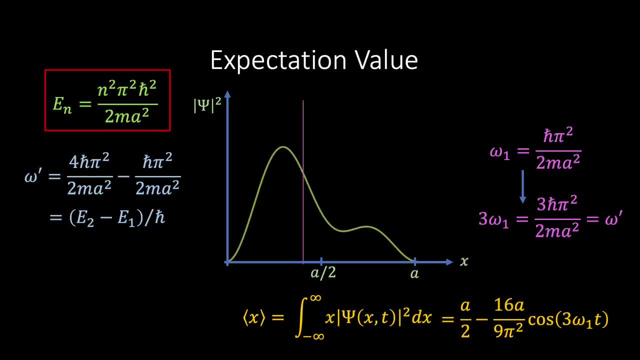 omega prime as the difference between the energy of the first excited state and the ground state divided by the reduced Planck's constant. And finally, we can rewrite the angular frequency in terms of the oscillation frequency and we arrive at the following beautifully concise result: 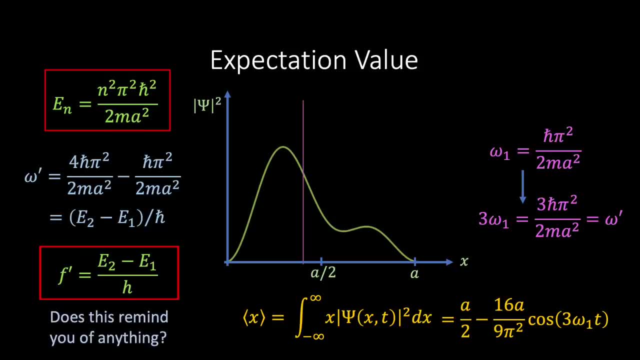 Now, the eagle-eyed amongst you might recognise this as the equation used to calculate the frequency of emitted light when an electron makes a transition between two energy levels inside Bohr's model of the atom, and you would be correct in thinking that there is a deep link. 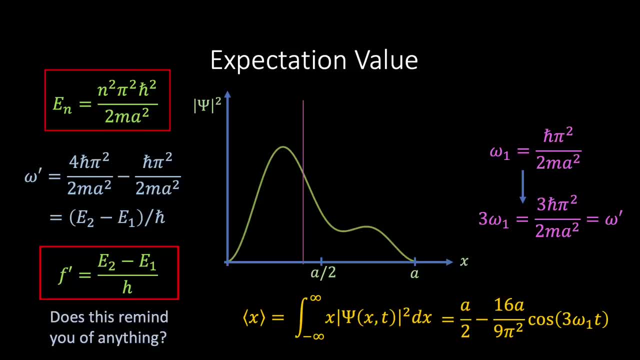 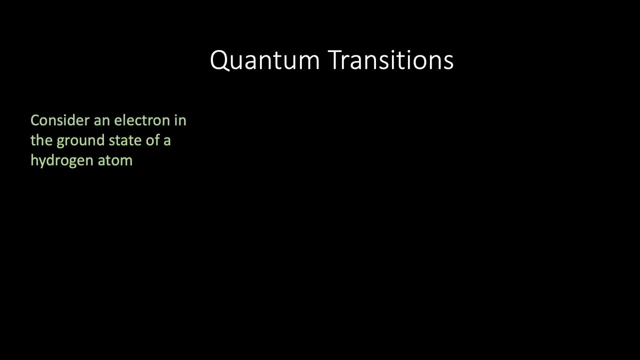 between our analysis and this famous result. And so, to end this quantum mechanical journey, let's discuss this exciting link in a bit more detail. If we begin by considering an electron in the ground state of a hydrogen atom, then according to Max Born's probabilistic, 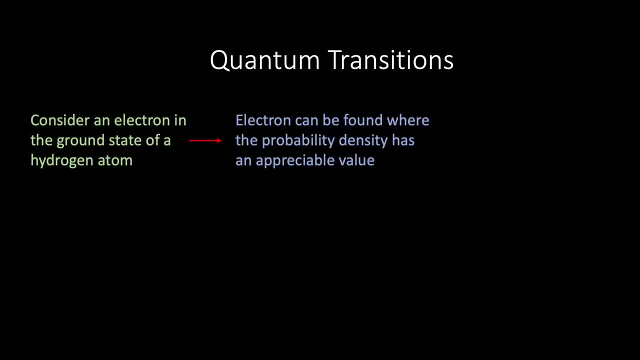 interpretation of the wave function. the electron can be found at any location where the probability density has an appreciable value, and it therefore follows that the electric charge of the electron would not be confined to a particular location within the atom, but rather distributed in proportion. 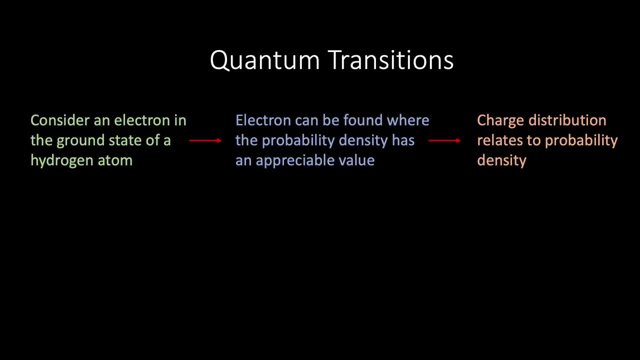 to the electron's probability density. Now, this might seem slightly counter-intuitive, but it follows logically from the analysis so far outlined. It's simply saying that the charge should be distributed in accordance with where it's most likely to be located within the atom. 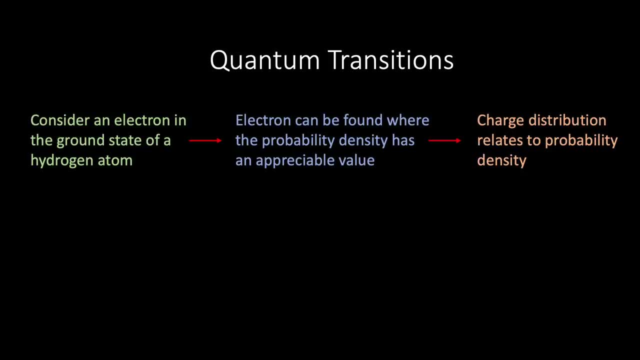 Now, when an electron is in the ground state of an atom, its energy is sharply defined And, as we've seen from our analysis earlier, this corresponds to a stationary state in which the probability density is independent of time and therefore the electron's 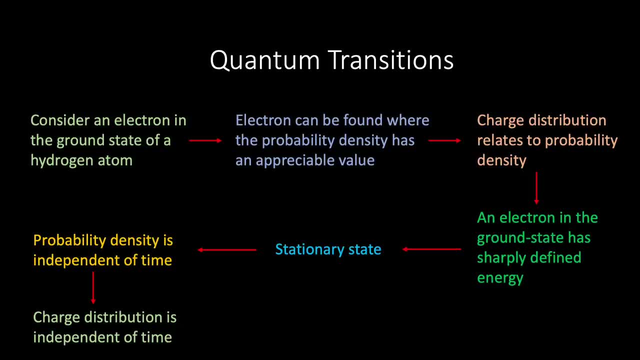 charge distribution is also independent of time. Now, according to classical electromagnetism, a static distribution of charge does not emit radiation. This means that the charge distribution in the atom does not emit radiation, and therefore we see that quantum mechanics provides a way. 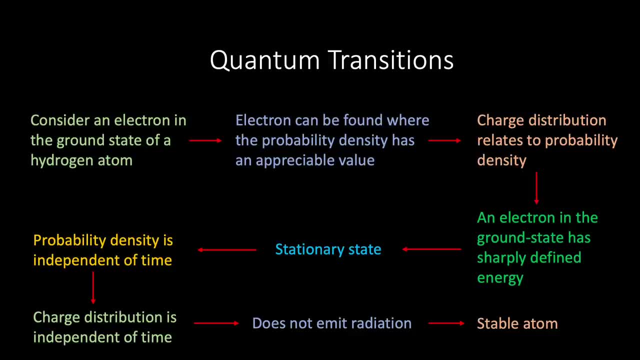 of resolving the paradox of the old quantum theory concerning the stability of atoms. If you recall, one of the great challenges facing the early pioneers of quantum theory was to understand how atoms could be stable, given that any orbital model of the atom predicted that the orbiting 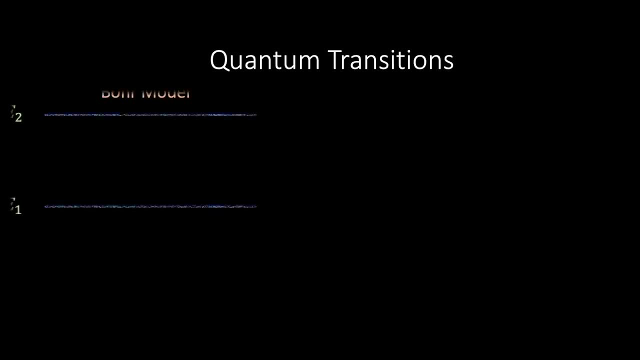 electrons should continuously emit radiation. According to the Bohr model of the atom, electrons that are excited to higher energy levels do indeed emit radiation when they make a transition from an excited state to a lower energy state. If we consider an electron in the process, 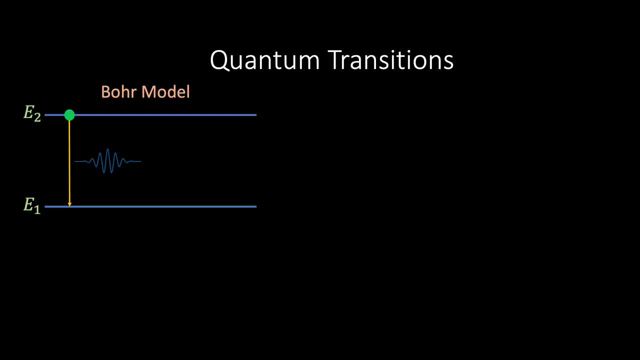 of making a transition, then, as we've just seen, the wave function describing a transition would involve a linear superposition of the first excited energy eigenstate and the ground state and therefore the probability density will oscillate, as we've just seen. 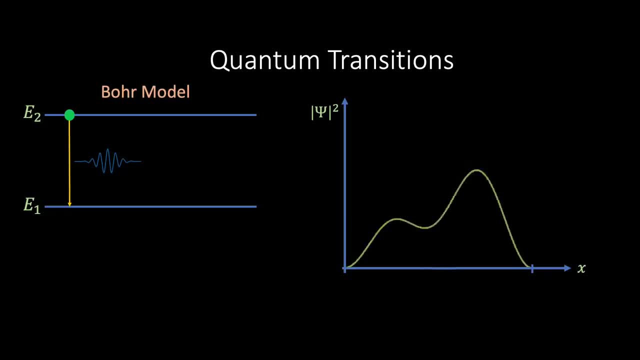 And since the probability density is proportional to the associated electron charge distribution, it follows that the charge distribution will oscillate in sync with the probability distribution, with a frequency given by the following expression: where E2 is the energy of the excited state and E1. 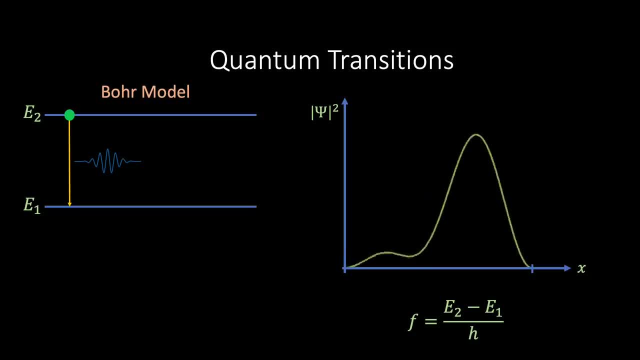 is the energy of the ground state. Now, according to classical electromagnetism, this charge distribution would be expected to emit radiation at the same frequency as the oscillation frequency of the charge distribution. But we note that this is also precisely the frequency of the photon. 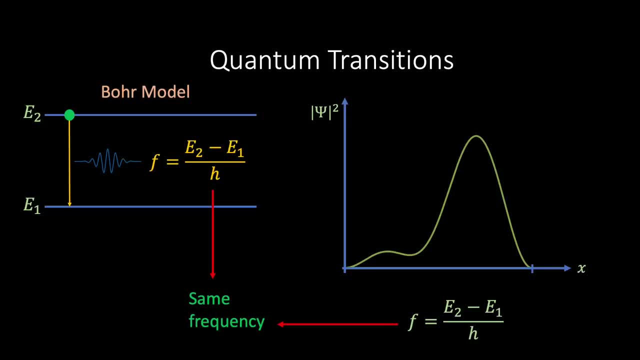 that would be emitted according to Bohr's model of the atom, since the energy carried by the photon is equal to the difference between the two energy levels. Interestingly, we see that this cannot happen for an electron in the ground state of the atom, because there is no 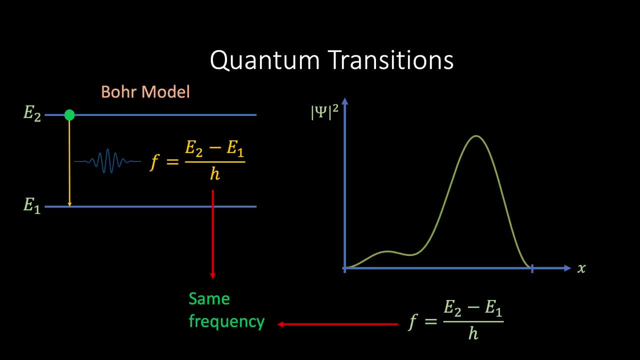 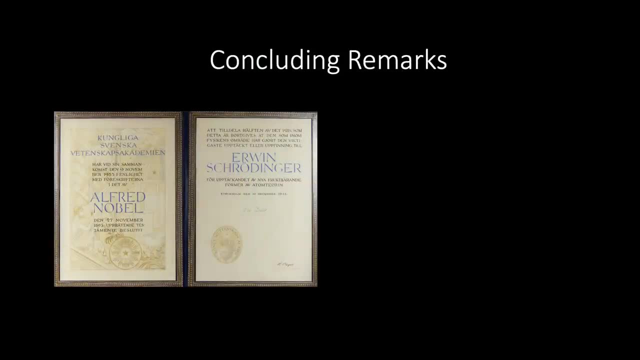 state of lower energy to mix with to produce an oscillatory probability, density or charge distribution. Now I find it quite remarkable that, even though we have used a very crude one-dimensional particle-in-a-box model for our analysis, we've been able to capture 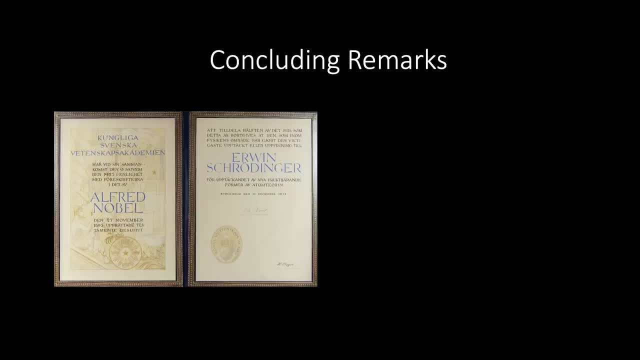 some of the most important and interesting features of the full quantum mechanical theory of atoms. In fact, one of the first things that Schrödinger did once he had developed his wave equation was to apply it to the hydrogen atom, and he was able. 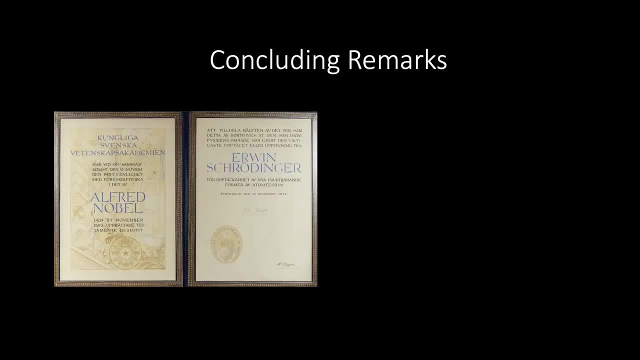 to show that not only does it correctly predict the energy levels of the hydrogen atom and the frequencies of the photons emitted in atomic transitions, but it also allows you to correctly predict the probabilities per second that those transitions will take place. It's interesting to note. 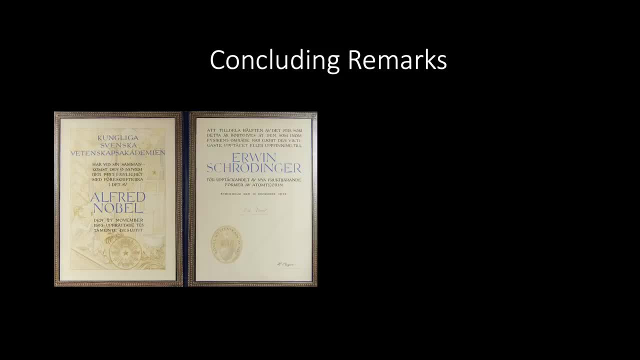 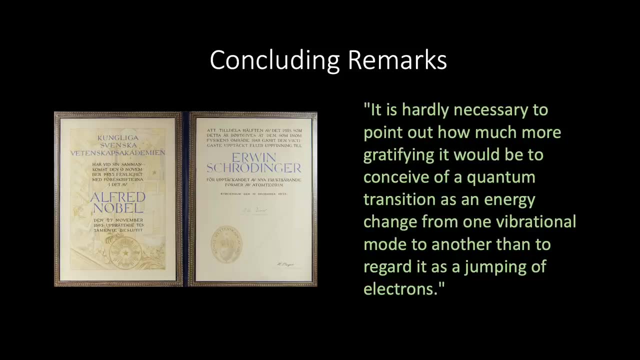 that Schrödinger believed his theory provided a physical picture of the process of emission of radiation by atoms. In discussing the advantages of his own theory, Schrödinger wrote: It is hardly necessary to point out how much more gratifying it would be. 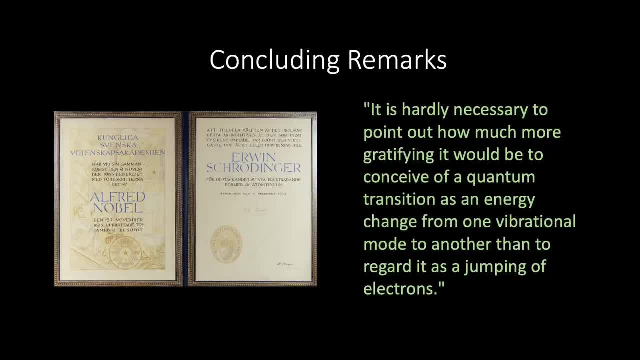 to conceive of a quantum transition as an energy change from one vibrational mode to another than to regard it as a jumping of electrons. There were certainly those who disagreed with Schrödinger's interpretation, but what is beyond all doubt is the magnitude. 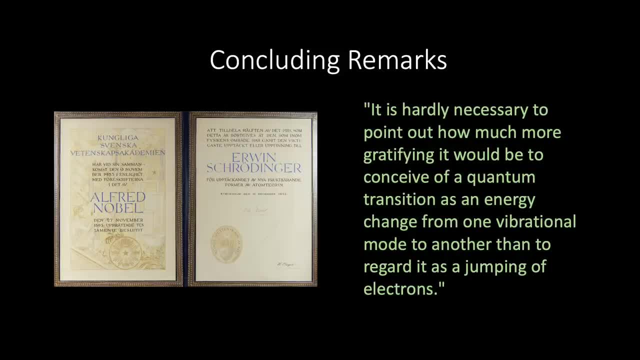 of the contribution that Schrödinger made towards our understanding of the atom. Unsurprisingly, Schrödinger was awarded the Nobel Prize for his groundbreaking work, and the equation that now bears his name lies at the heart of our modern understanding. 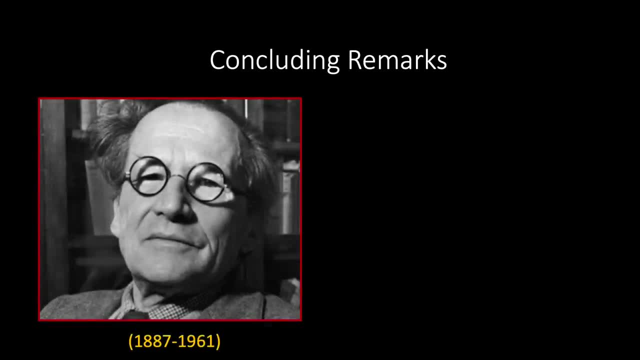 of particle physics, And I think this is as good a place as any to bring this quantum mechanical journey to an end, for now at least. The good news is that if you've made it this far, then you have covered some of the most. 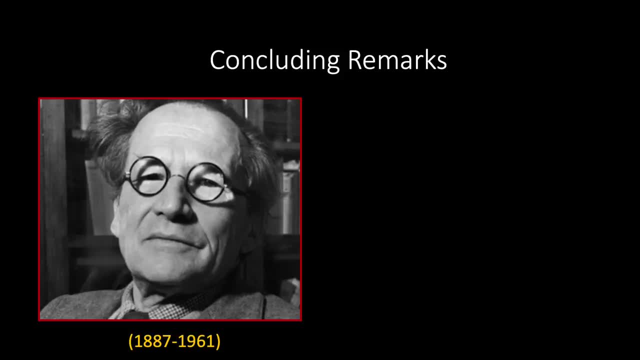 important ideas in any introductory course in quantum mechanics. And perhaps what's even better news is that in my next video I'm going to put Schrödinger's equation to the test when I explore quantum tunnelling and how it enables the stars to shine. 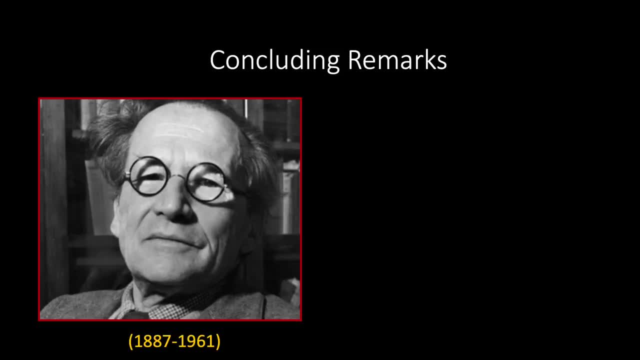 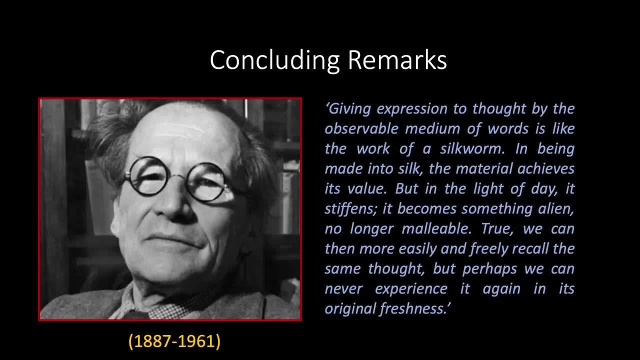 It feels only appropriate that I end by quoting the words of Schrödinger himself, who said: Giving expression to thought by the observable medium of words is like the work of a silkworm. In being made into silk, the material achieves its value, but in the light 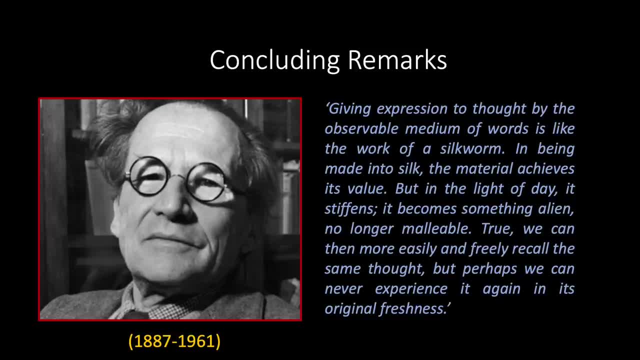 of day, it stiffens, It becomes something alien, no longer malleable. True, we can then more easily and freely name thought, but perhaps we can never experience it again in its original freshness. Thank you for watching.